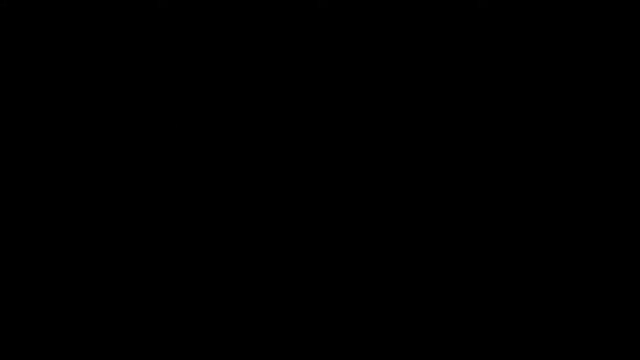 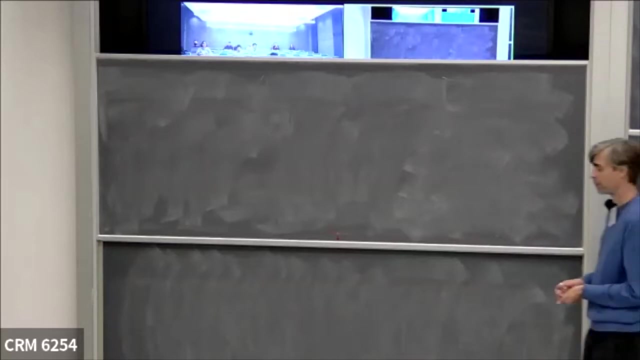 Okay, so this morning I explained non-equivalent steady states and gave an example in conformal field theory. So now the point is: I'd like to go further beyond CFT. So in CFT we could do all the computations explicitly for the DR0 sector, but in general it's much harder. 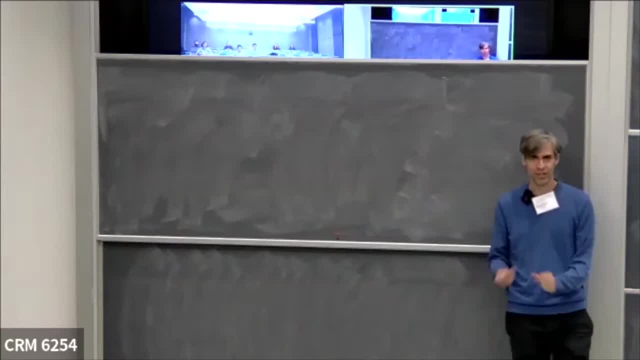 to do computations explicitly. I mean, this is a hard problem, right? So you have initial state, which is quite non-previewable, with different temperatures left and right, which is not stationary, and you go with an interacting many-body Hamiltonian. this is just a hard. 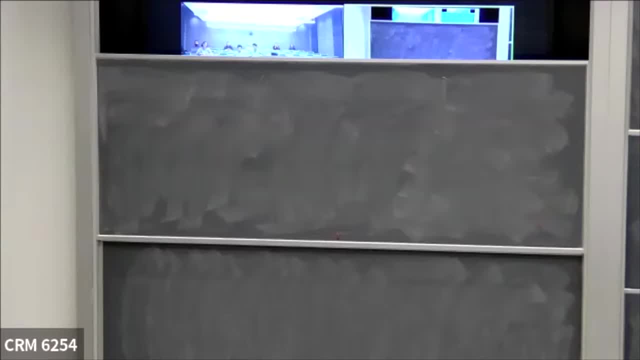 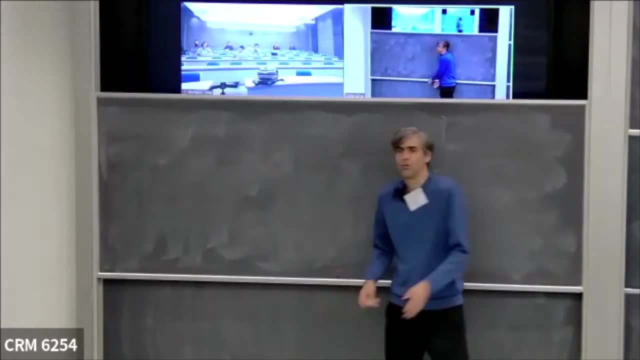 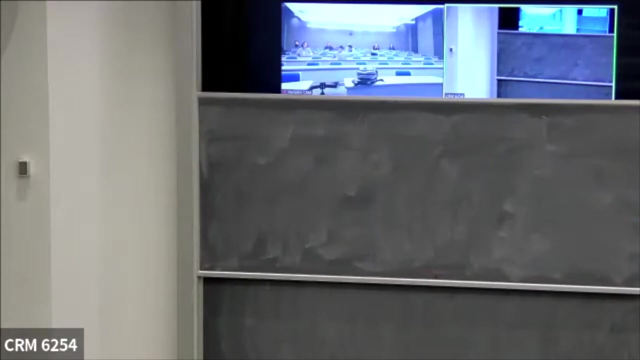 problem. It turns out that there are very strong techniques- I mean techniques that allow you to get quite strong results- And I want to show kind of well. first I start with one kind of small general inequality set of inequalities that we can write for. 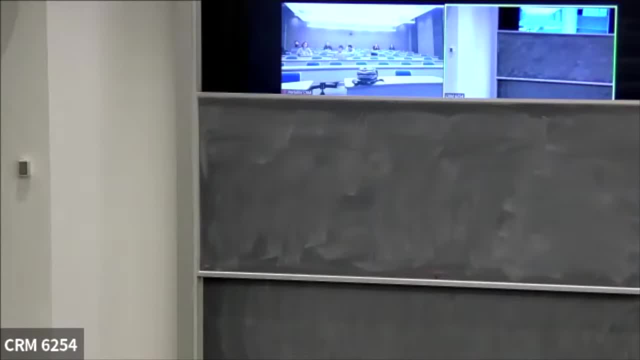 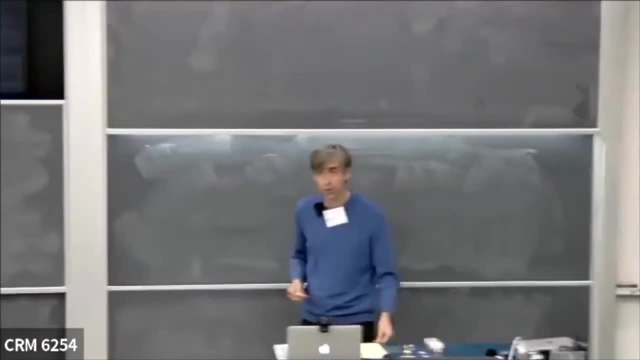 stationary state averages, just some general inequality that comes from. I mean, it's not a complete general proof, but some general physical principles, so something we can write without having to know too much about the macroscopic systems, And then I will talk. 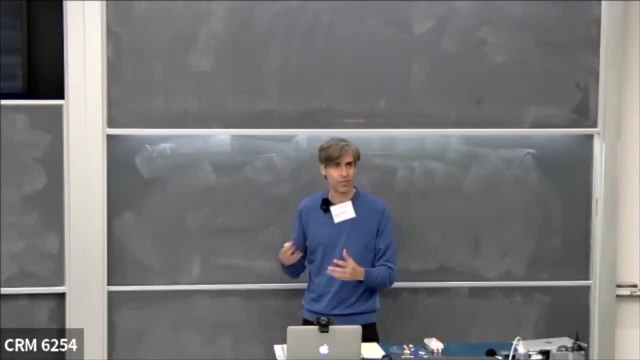 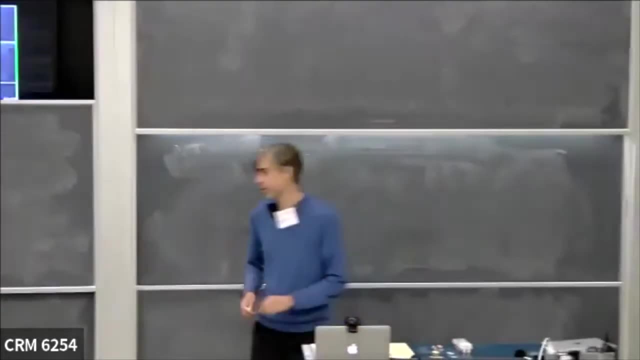 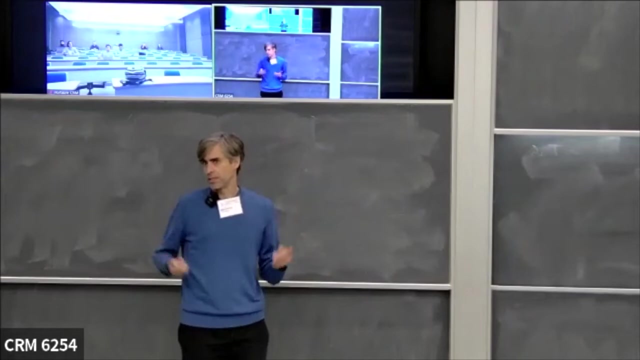 about the hydrodynamic idea, which are, you know, physics ideas. you can use hydrodynamics to divide stuff, And that really allows you to calculate a lot of things, And eventually, with hydrodynamic ideas, one can go well, in principle, to interacting systems, although of course then it can be. 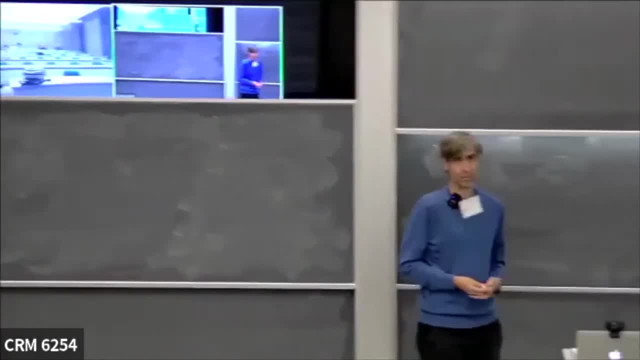 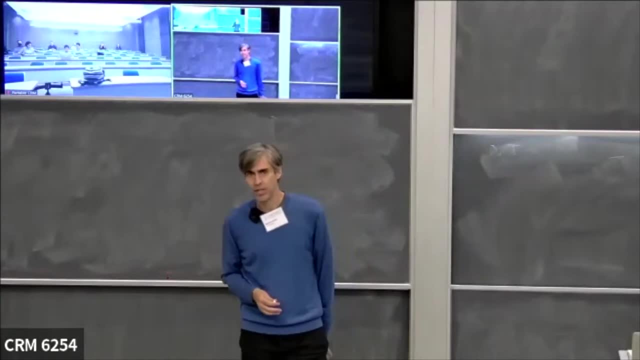 complicated to have something explicit. but to integrable systems where you can have something quite explicit. I'm not going to, I don't want to go into too much of the details of integrability and all that I mean. I don't want to be technical here but explain the. 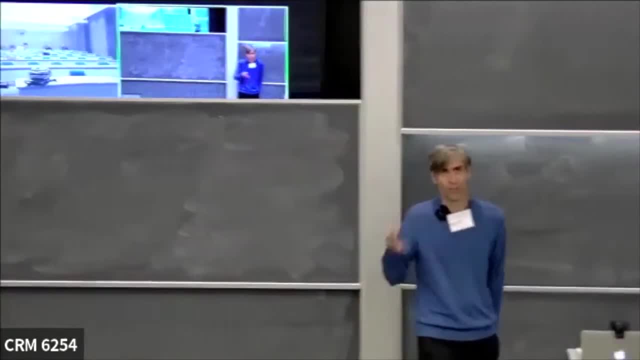 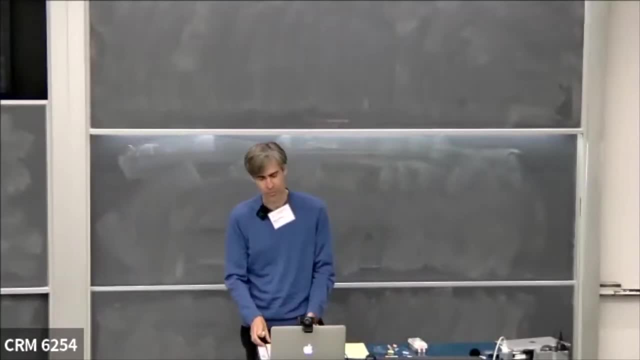 main ideas and I can illustrate everything, even with three fermions and see you know five goals and generalize to integrable systems in some way Using known results from beta and test without having to do by beta and test results. I'm not going to do any beta and test in here, Okay. So the first thing I start with is some 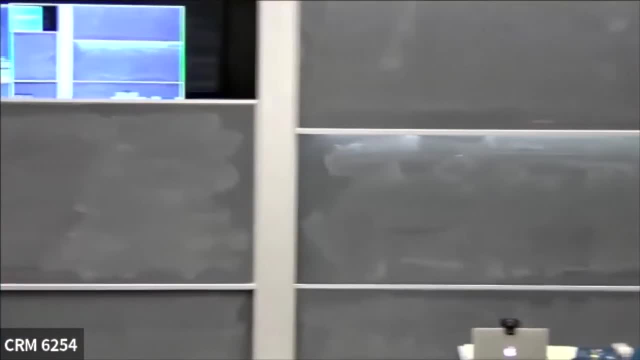 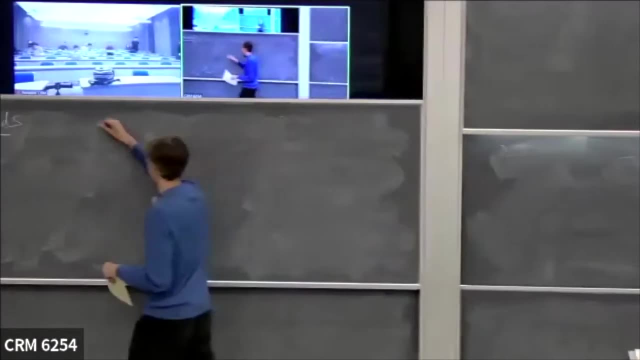 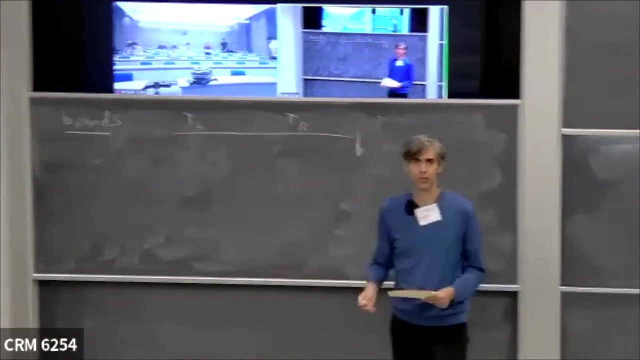 kind of a general bounds or inequalities. So, remember, we have now, so we still think about T left, T right. if you wish, then something about more complicated, but we have T left, T right and the system there and we let time evolve and we look at stash and we stayed. 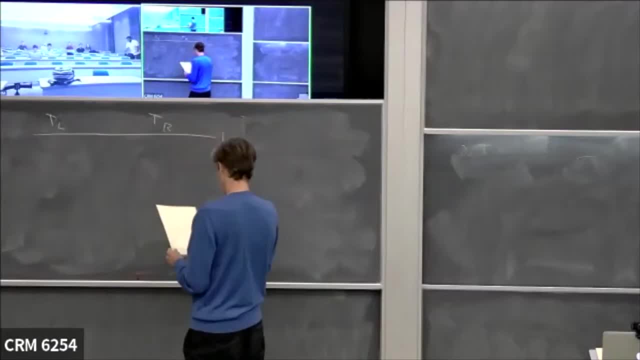 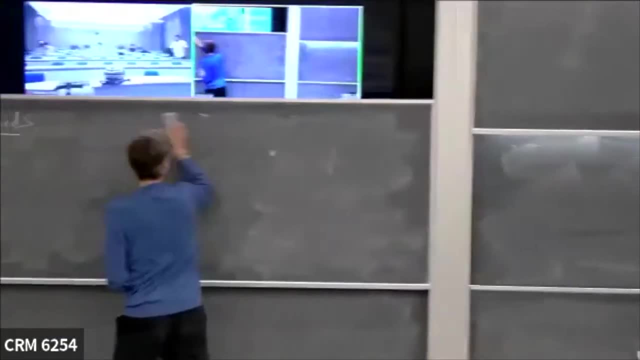 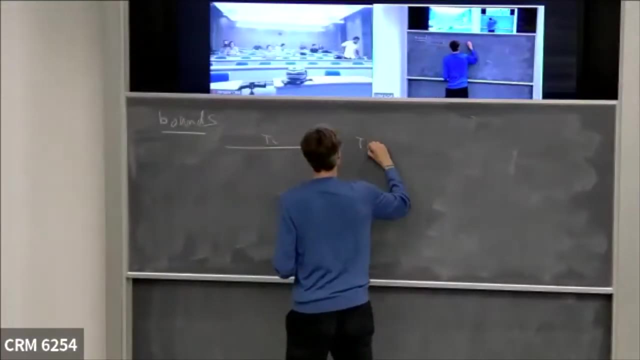 far in time. So, yeah, I don't know if I, I my pictures in my here are inverted, So I'm going to have now time. go upward instead of backward, if you allow me, otherwise get very confused. Okay, So this is T left, T right time, evolved like that And once in what's happening now. 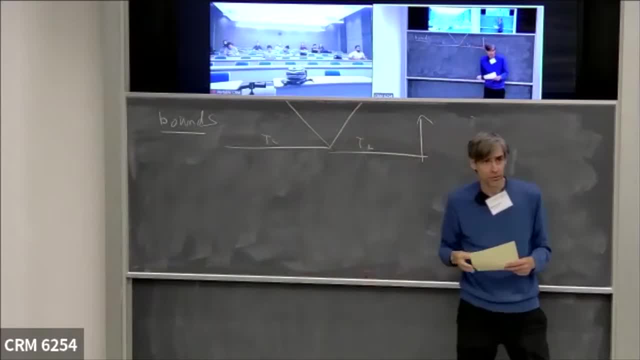 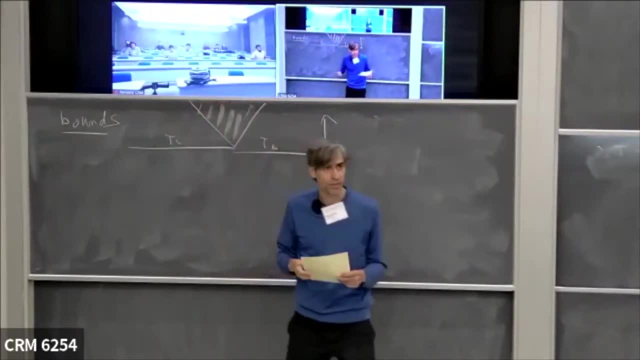 we know that there is some kind of light cone, light cone right, So beyond that is still T right. there is some T left and something non-trivial is happening in here, And then what's happening? So there are certain equal inequality that we can write for our basic. 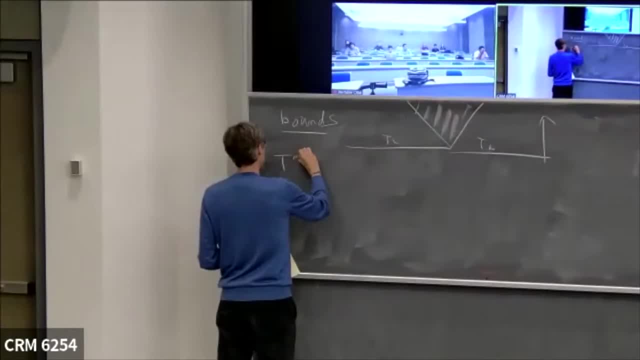 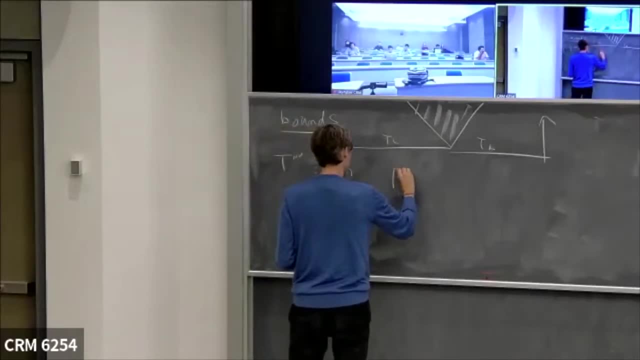 quantities. Okay, So I'm still thinking about the stress energy tensor and I'm still thinking about relativistic theory, say Q of T, right? So I still have some energy density, some current of energy, which is the momentum, because it's relativistic variance momentum, and some 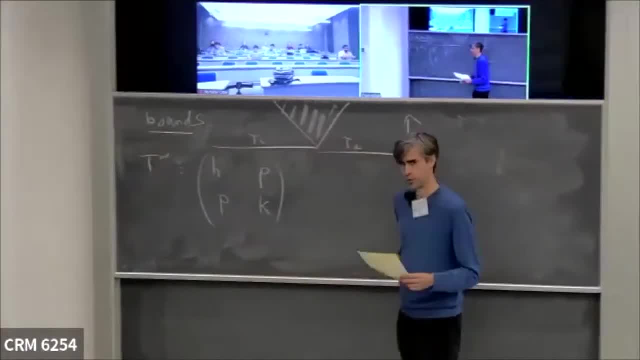 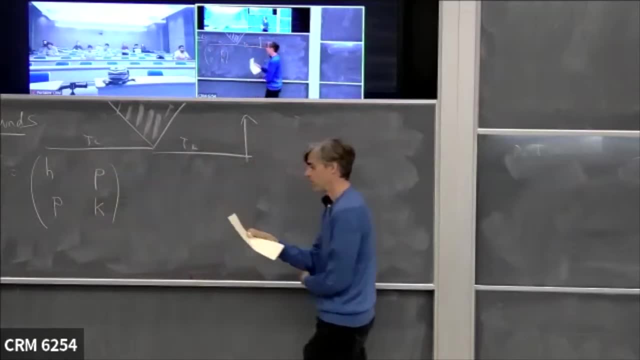 current of momentum, which I am going to call K here, just to give it the letter. Okay, In CFT this is equal to H. then I have simplification, But in general, well, I, you know, I don't know what, what that is, This is just some. 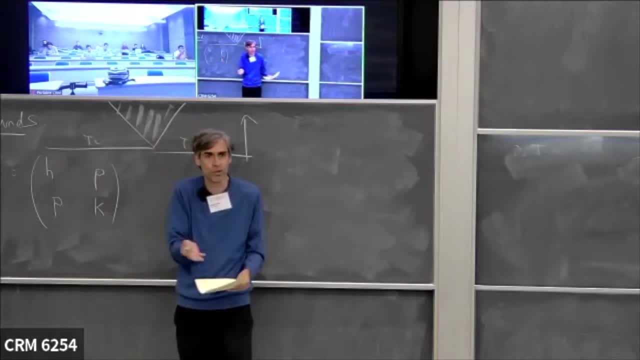 other operator. right, I can write explicitly the operator in some given theory, but it's something complicated. Okay, So these are just local operators. It takes some form, and doesn't matter too much what form they take. Then I calculate their average in this initial 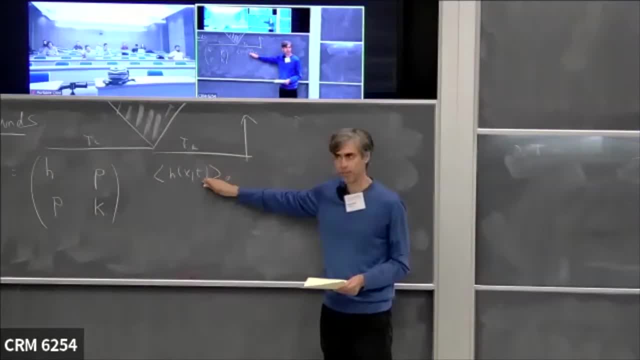 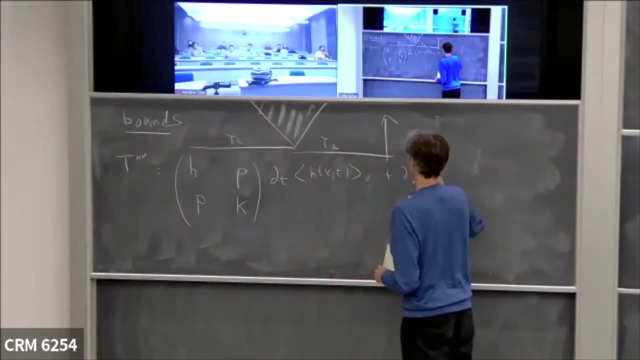 state, evolving time, space time- Look at what happened in space time. Okay, And I know that these will satisfy some continuity equation because they are, you know, conceptually current right. So I'm going to have this continuity equation for the energy that involved. 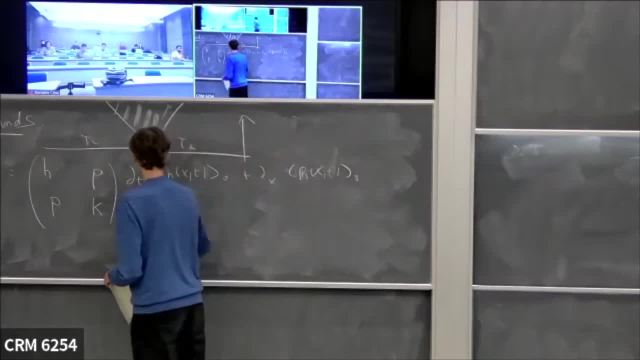 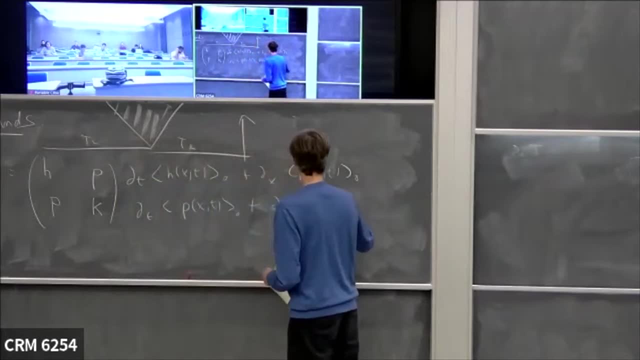 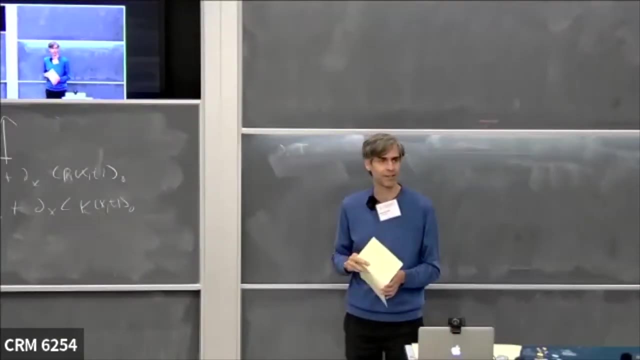 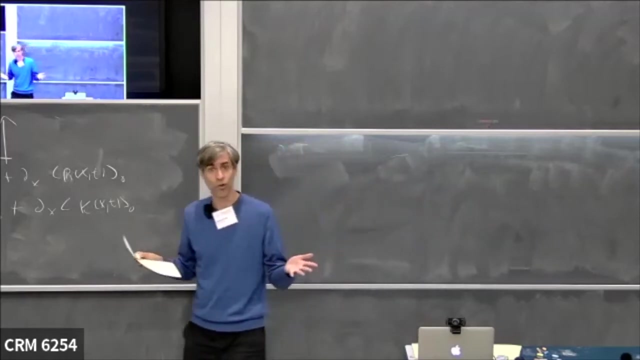 the average energy density, momentum and continuity equation for the momentum itself. So momentum continuity, and that's going to be involving the average of the momentum current. What's the momentum current physically? Do you know what's the momentum current physically, Physical meaning of that Current of momentum? So how the momentum changes in space or something. 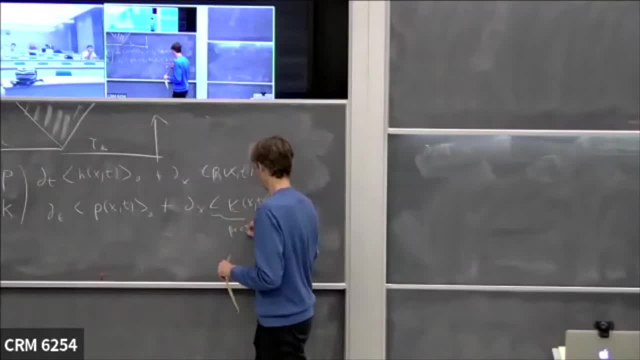 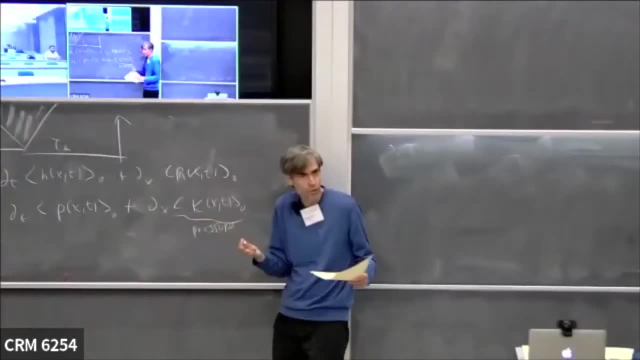 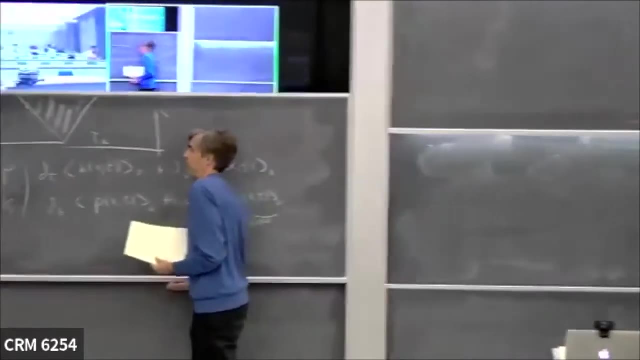 It's, it's a pressure kind of you know. so, indeed, this size data, So this is a pressure quantity. It's, it's even on the time reversal, for instance, like the energy right, It's some kind of some, some simple quantity, but it's, you know, it is a non-trivial function. 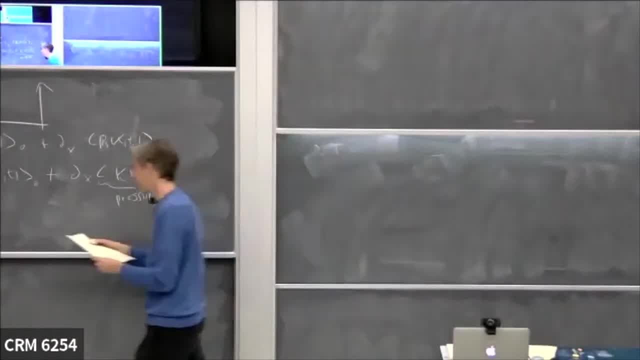 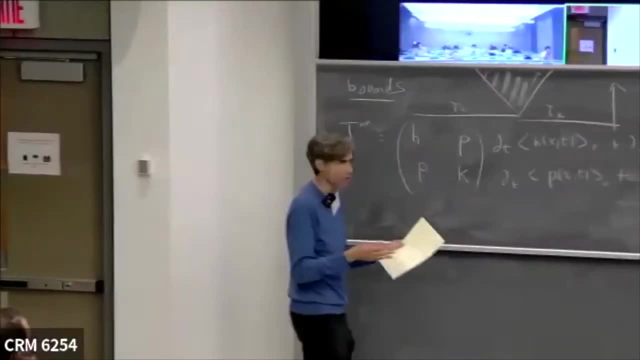 of XT and I don't quite know what it is. Okay Now. there's so the inequality that one can write the following, and this is in relativity KFT with velocity one, but one can change the Lycone velocities. The formula will change, but for now I take it to one. So the quality. 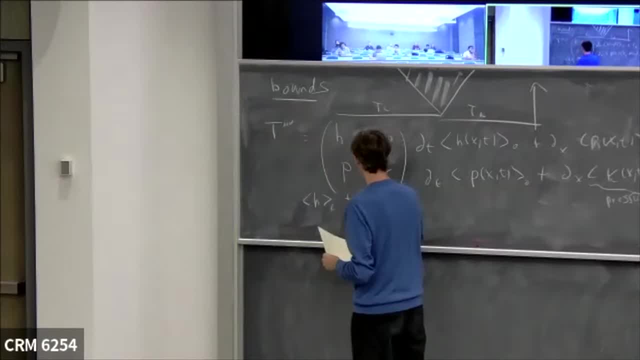 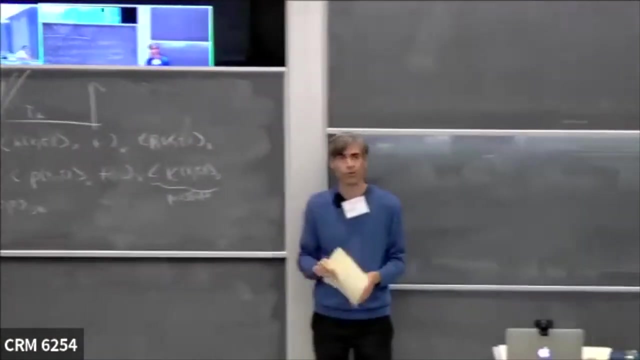 is that if you take the average of the energy density on the left minus the average of the energy density on the right, divide by two, that always is greater than the average momentum in the stationary current in the stationary state. So that's a lower bound. 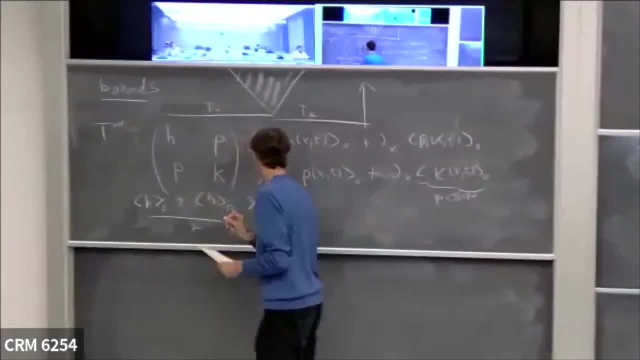 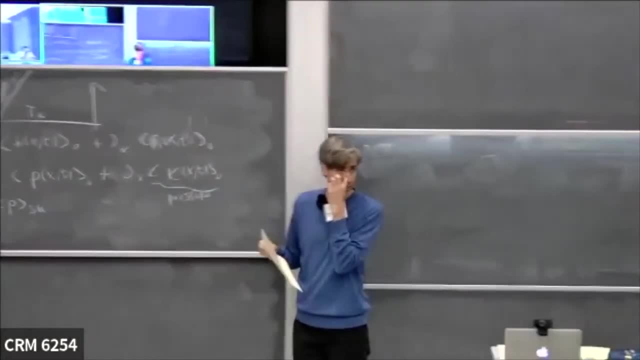 Sorry It's. it's a upper bound for what the current in the stationary state can be. It depends on the difference of energy. The energy is on left and right. If the energies are the same, there's no current, But there. 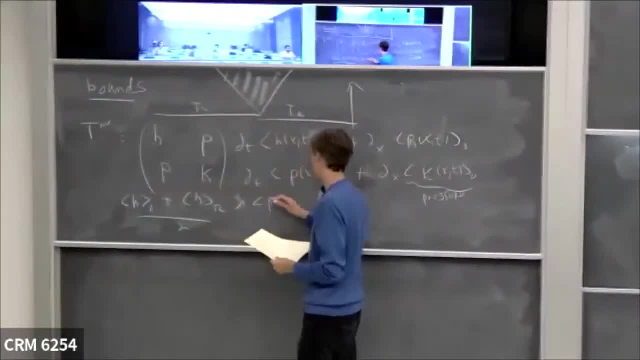 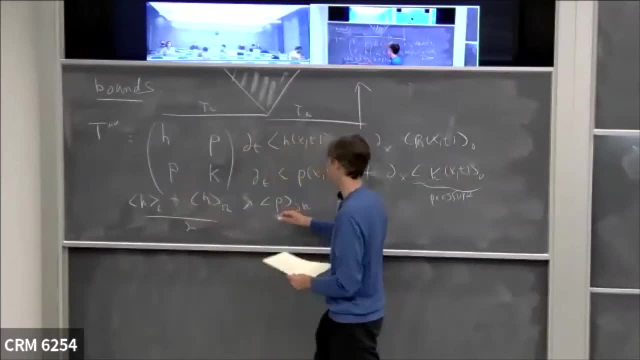 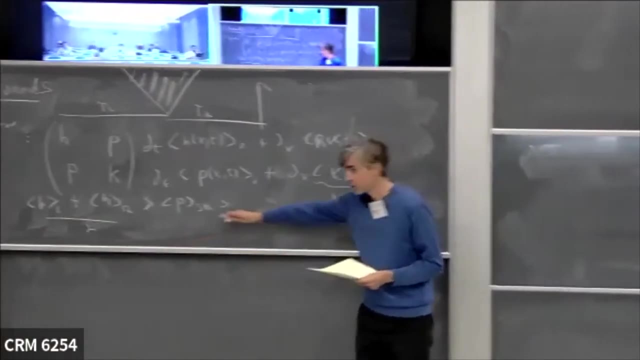 is there, but I mean this is a lower bound, So somehow the current must be. I mean it cannot be too much. If it cannot be too much, if the current is too high, I mean you have to have a big energy difference. More interestingly, there is also a lower bound for the stationary. 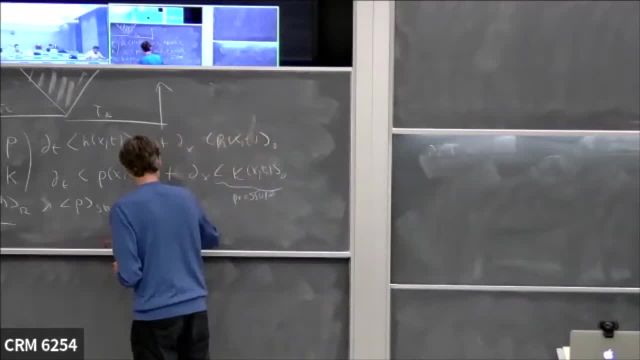 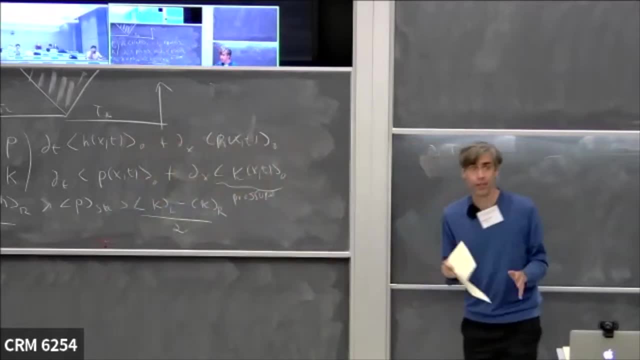 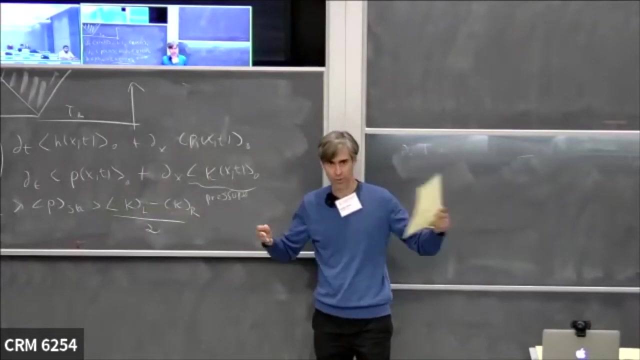 current which is determined by these pressures. So K left minus K right, divided by the energy density of K left minus K left divided by two. So there must be a current if the left and right pressures are different, which is natural Right, Because you have pressure there, more pressure there and less there, You're going. 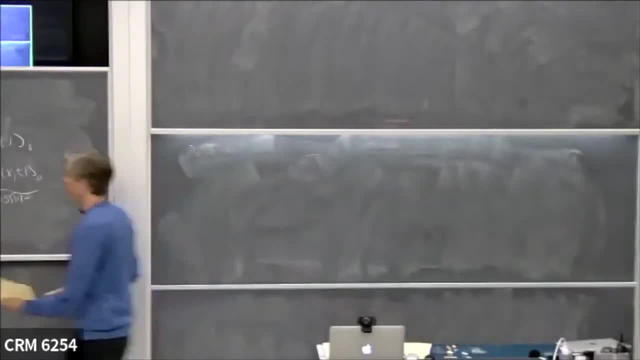 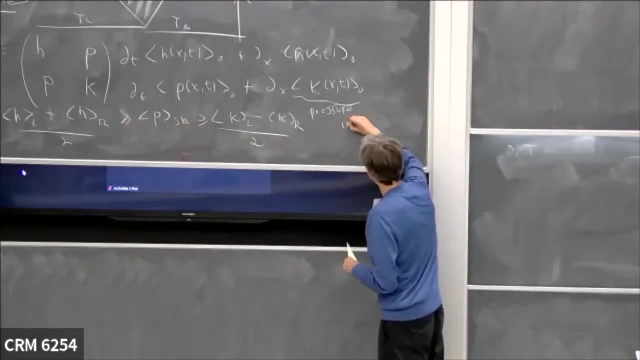 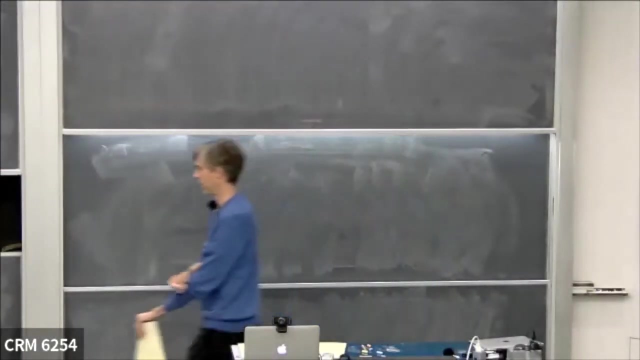 to have a zero current. Okay, So there's these. generally inequality that should be satisfied: is smaller or bigger available? and in CFT you can check in CFT, because now K is equal to H plus You have, you have equalities on both sides. So these two bounds are exactly saturated. But in general, 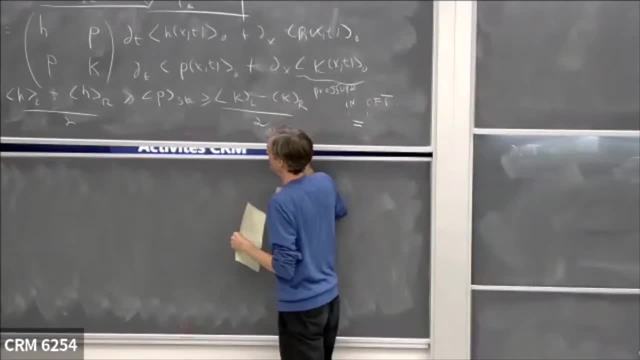 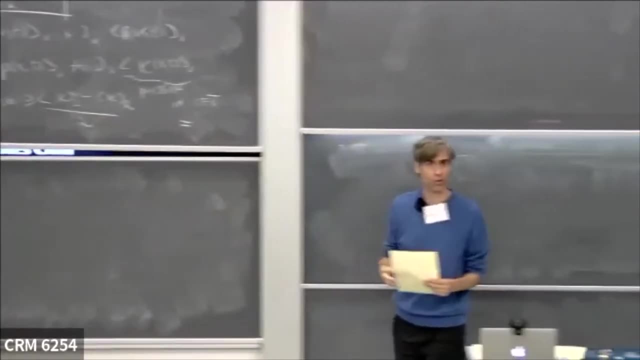 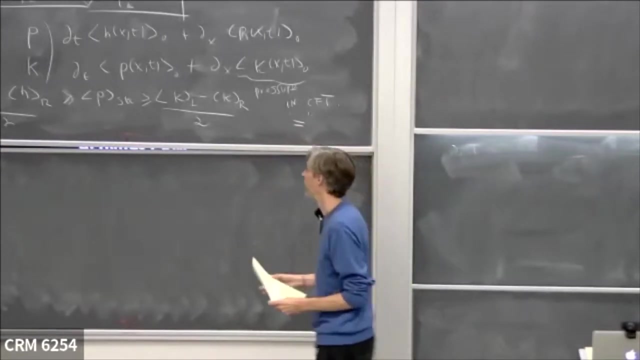 these are bounds. We don't quite know exactly. So the stationary current average momentum is not just simply determined by the pressure or the energy, like it is in CFD, as marginal. So why is that this bound? Well, you can argue for it. not completely, but you can argue for it. 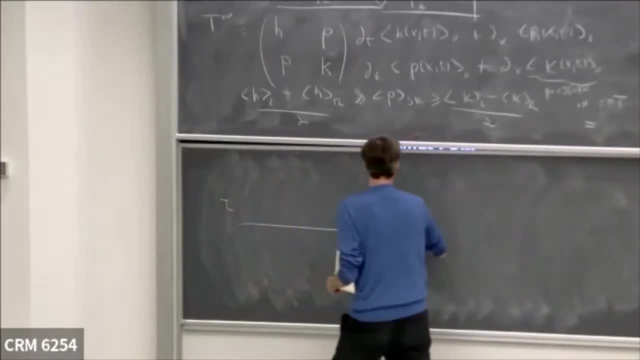 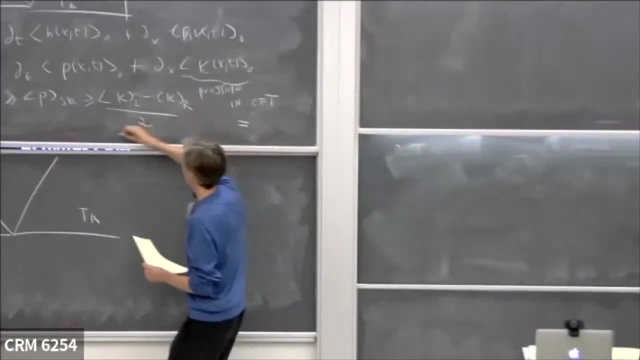 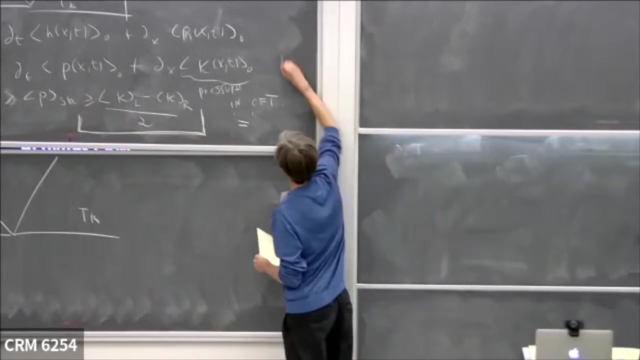 like that. So you have again your T left and T right there And you have this cone like this And you write: I'm going to do just the second bound. The first bound is something similar, So I'm going to use this one here And you consider that continuity equation for the momentum. 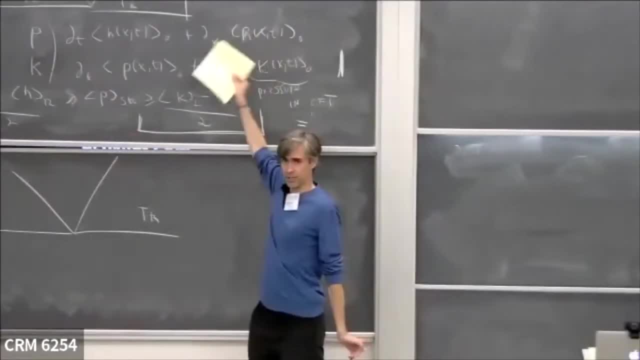 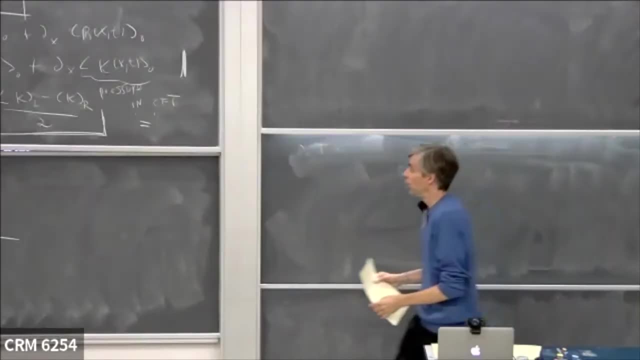 This is momentum density, which is also the energy current. So this is what allows us to calculate something about the current, Because the density is the current of energy. This is the conserved density. So okay, So there is this continuity. 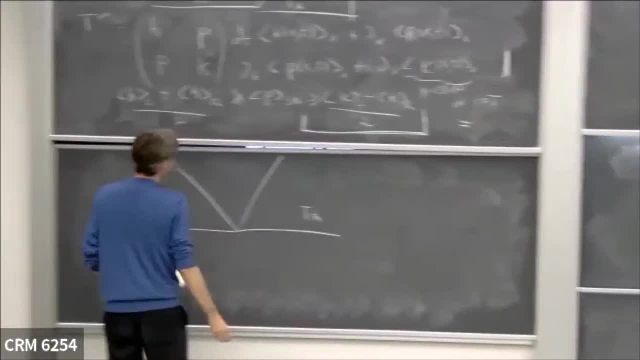 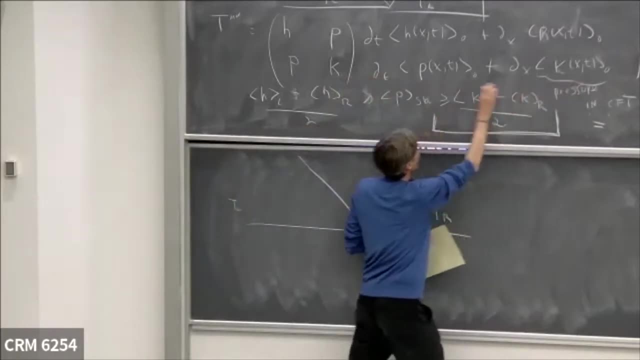 equation And we have that structure like that And what you do? you just write the global form of the continuity equation So you kind of integrate that over space-time. So if you integrate that over X and T, when you integrate that over X and T, you use the T derivative. 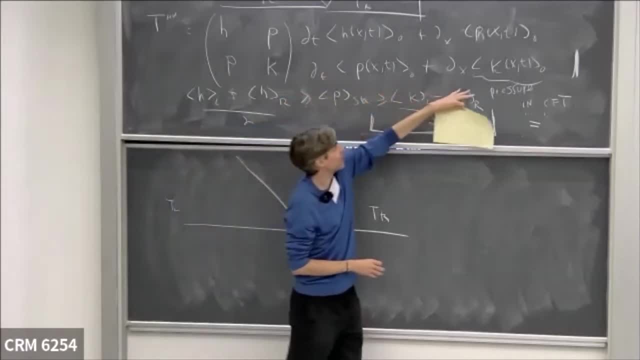 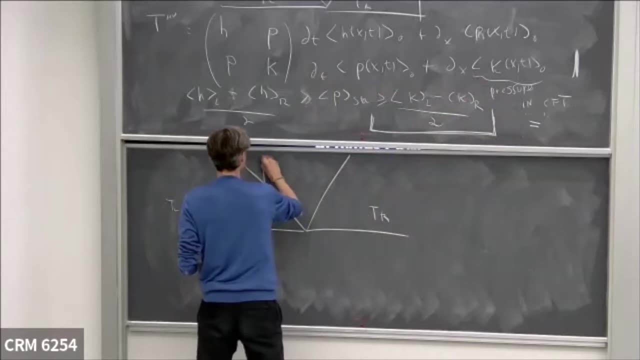 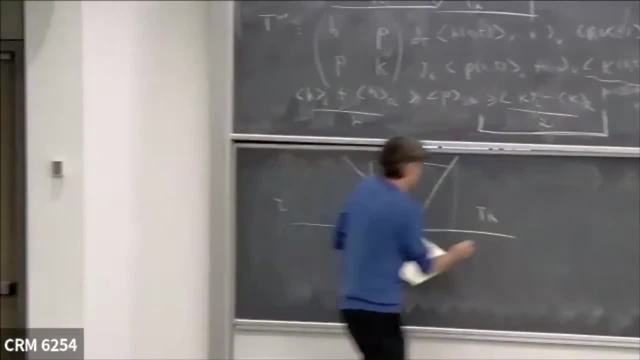 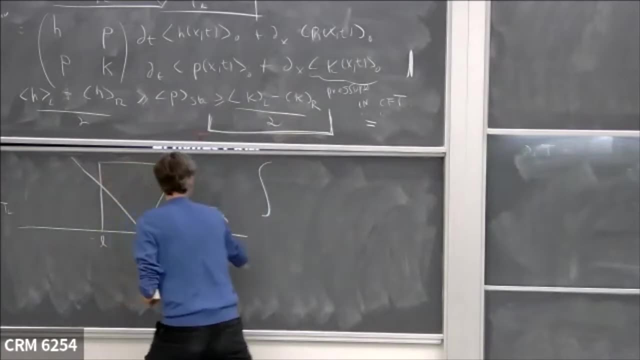 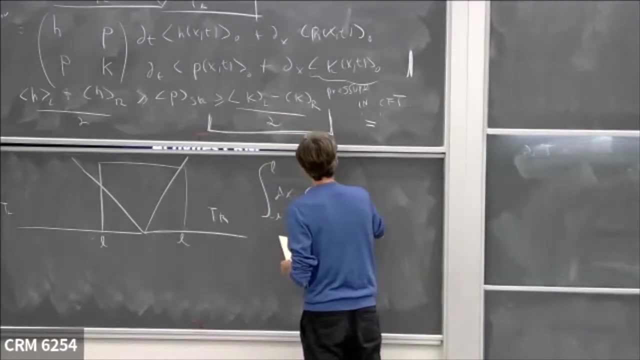 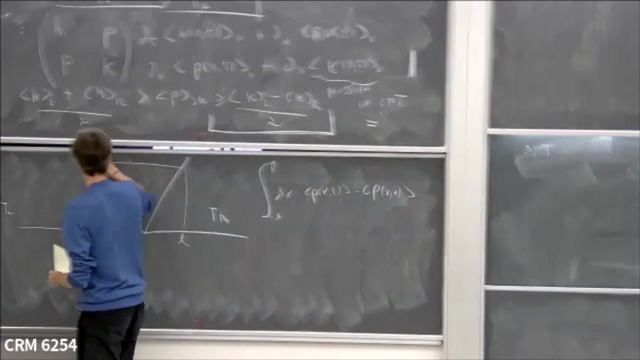 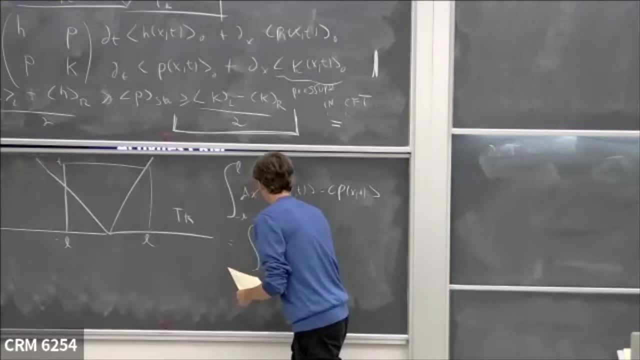 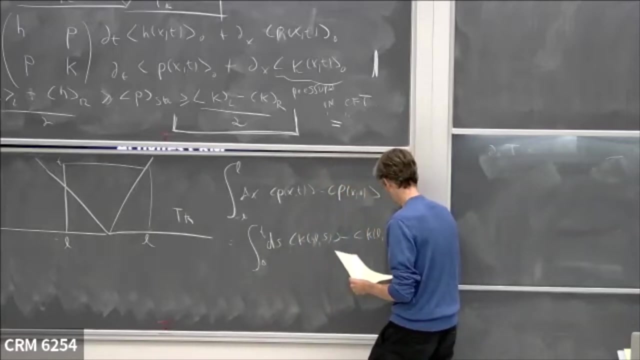 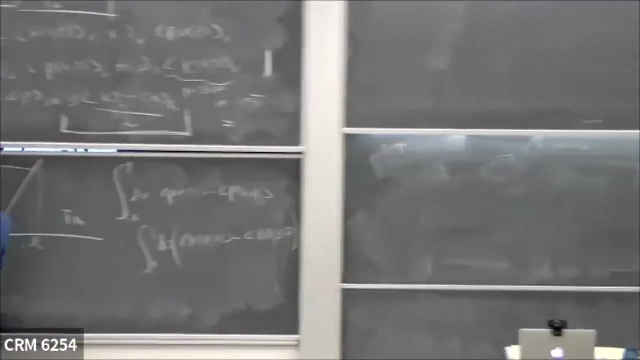 This must be equal to the integration, from zero to T, of the average pressure. So the pressure at minus L S minus the pressure at L S. That's it. So I have this relation. Okay, So this is what's happening. So I have this one, that one, that one and that one. Okay, Now the current in. 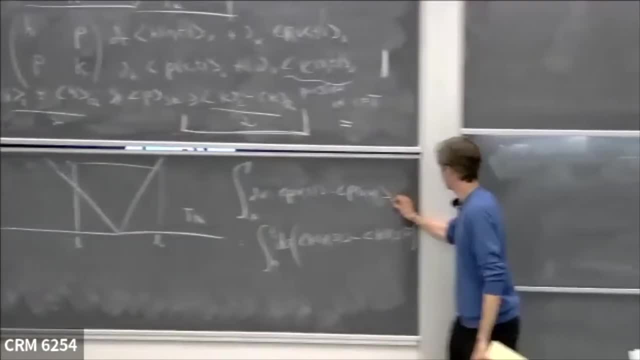 the initial state. Okay, So I have this one, that one, that one and that one. Okay, Now the current in the initial state. So the momentum is zero in my initial condition. So that goes to zero. Okay, Then I have this and: 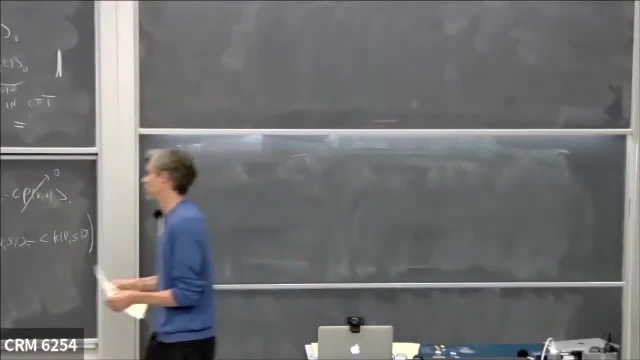 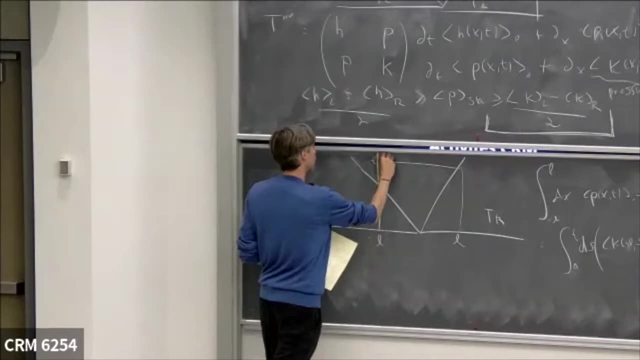 that. And then the idea is simply to- I mean to use a bit of physical argument here- If I take T very, very, very large, going to infinity here. Okay, Well, I know that for L fixed and T going. 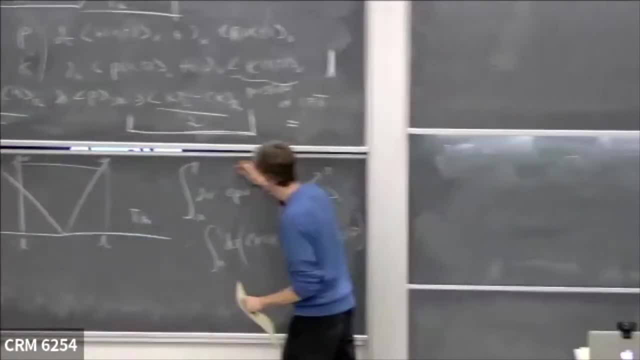 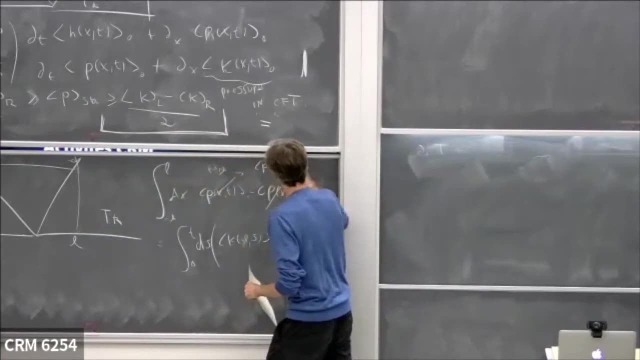 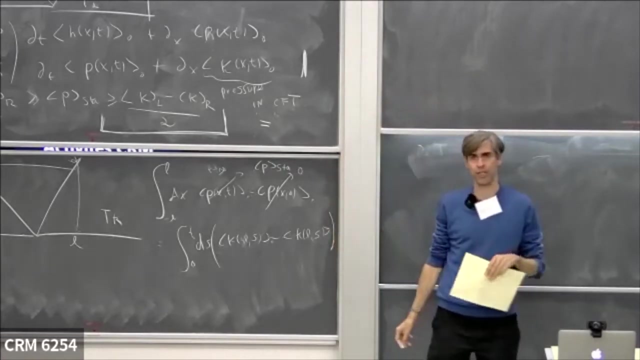 to infinity. that is going to be what At T goes to infinity. that's going to be the average P in the stationary state, constant for all X. T, very large for fixed L. you know that goes to the stationary state. So the left-hand side then is going to be two L times the stationary state. 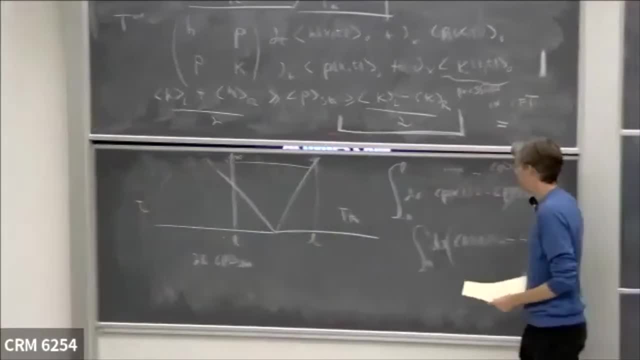 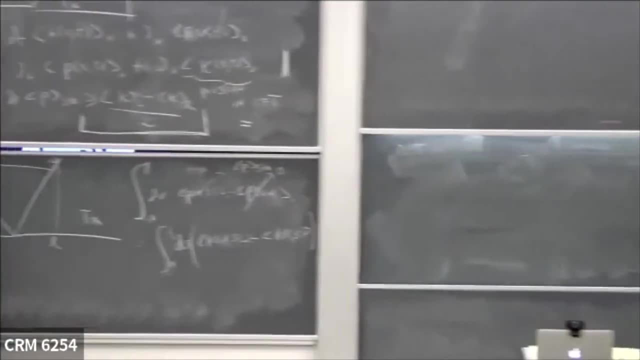 average of the momentum. Okay, Well, the right-hand side, well, I don't know what it is, It's something a bit more complicated. Okay, But then if you think about that, suppose I have a pressure there. average of K. 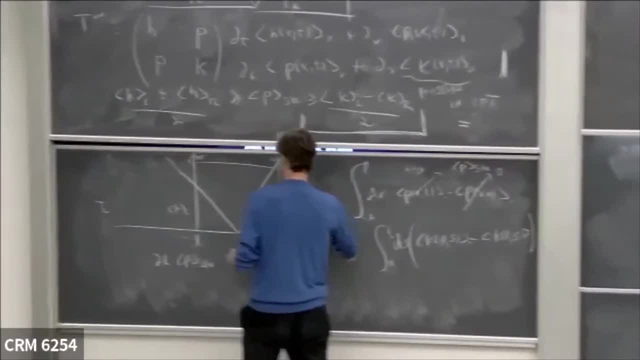 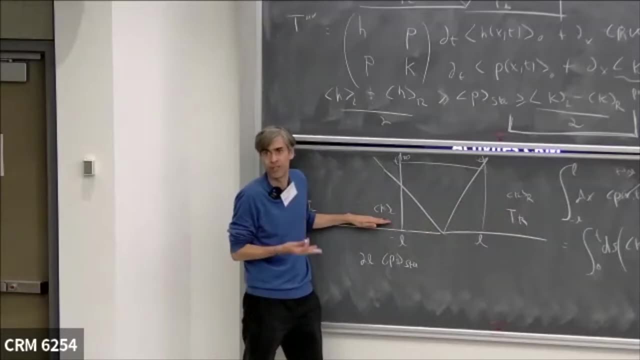 left and average of K right here and I have temperature higher here than there, then the pressure should be higher. In relativistic QFT that can be shown, that the pressure is monotonic with temperature, And what happens here? Well, I'm going to have some average of K. 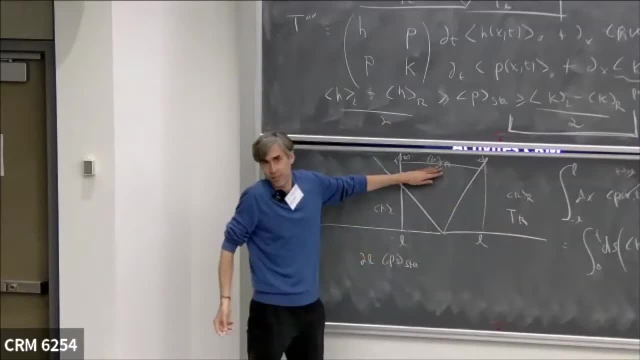 stationary, which is going to be something in between, right? So physically I don't know exactly, But supposedly- I mean intuitively- it should be something in between. So how does it go, The pressure from there to there? It should kind of change. 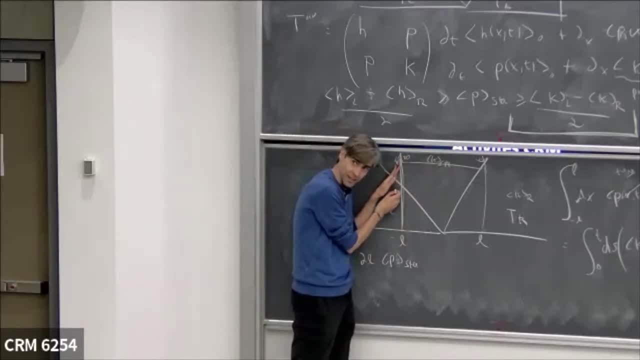 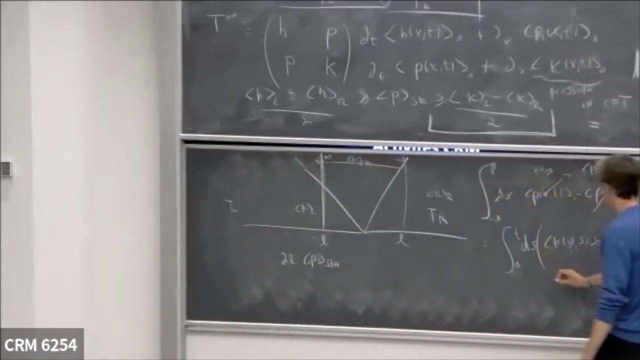 more or less monotonically from sorry, from something high to something in between, and here, from something low to something in between. Now, one can try to make these things more precise now than to bounce now, But just with this idea, okay, you write this bit here as: 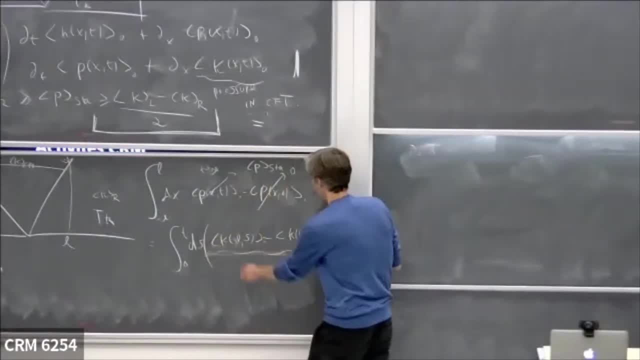 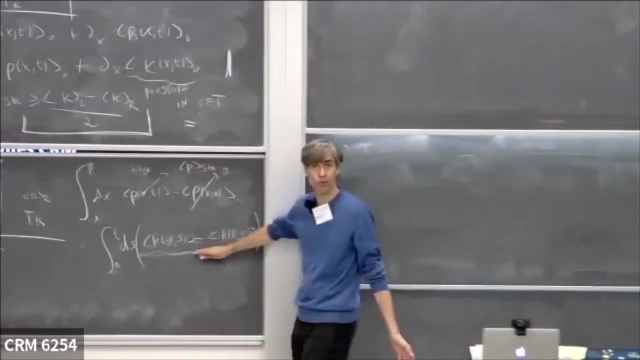 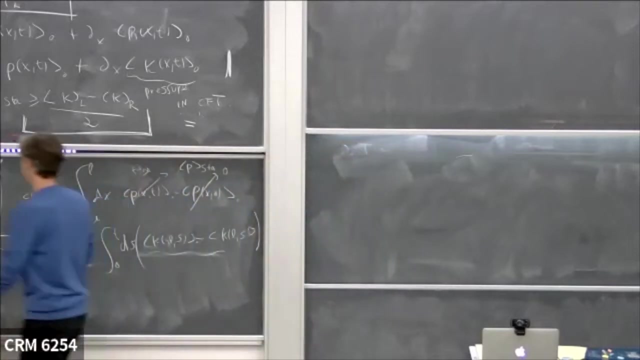 this bit here as well. okay, So you have something on the left minus something on the right which is large, And as time evolves it goes to something zero. So this is something positive throughout time. So we have, from zero to T, something positive And in fact, from here to 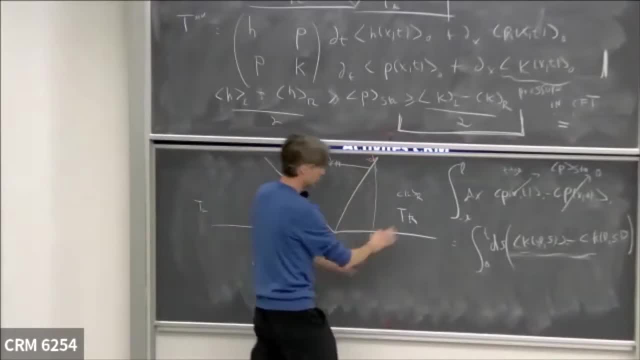 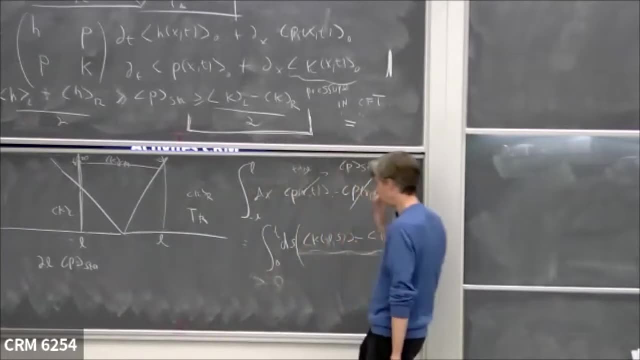 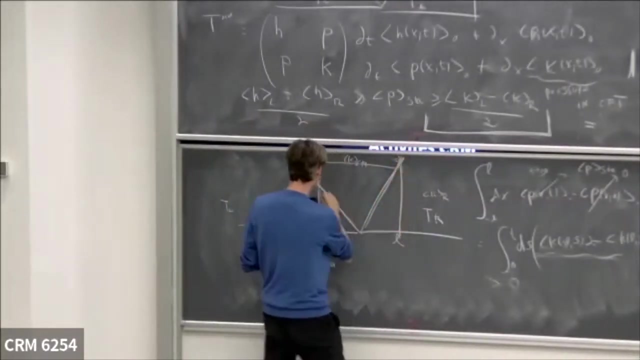 there it's, yeah. so let's say just, this is just something positive. greater than zero, okay, Sorry. greater than no precisely, sorry, So great, yeah, more precisely. So there is this light cone, So this is really K left minus K right all the way there, plus something positive. 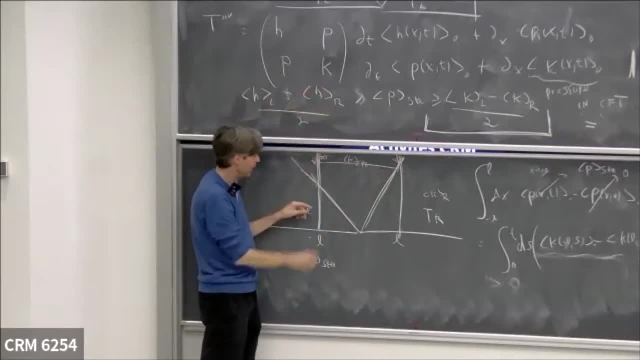 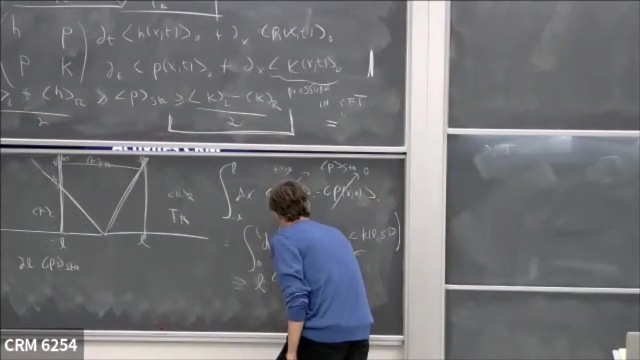 will happen later on in time that I don't know what will happen. But is this K left minus K right? all the way there, right? And that's multiplied by L all the way up to the light cone? essentially okay, So that will have the factor L: K left minus K right. 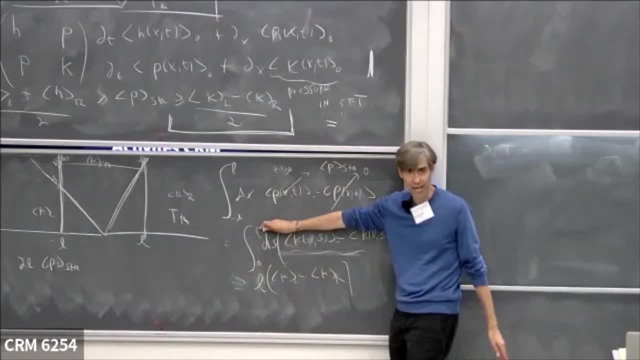 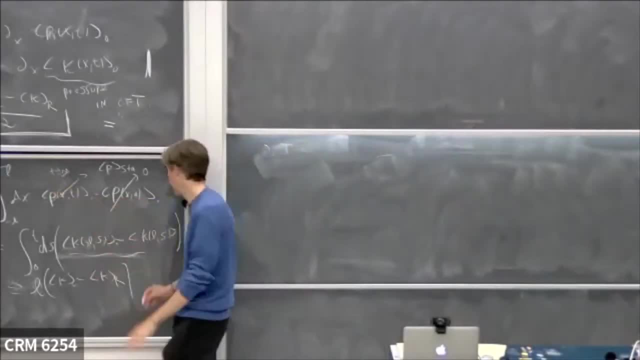 which is the bit of the integral. from zero to time equals L up to the light cone plus the rest. The rest I don't know. I don't have much control over the rest. okay, But I'm saying from physical argument is positive plus some constant. 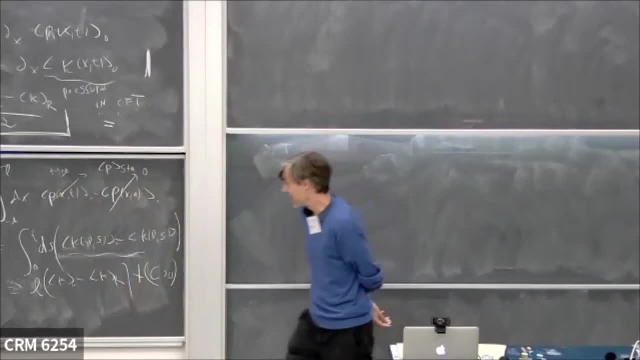 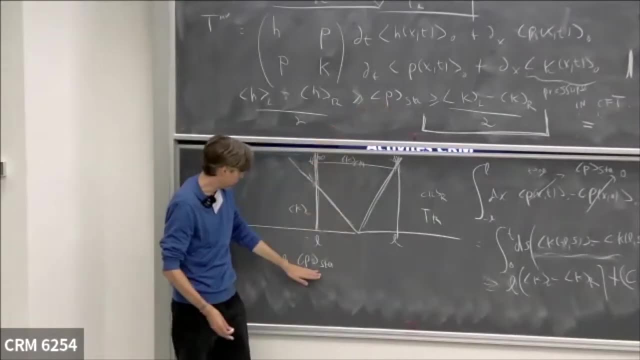 which is greater than zero. Okay, And that's the thing. So essentially you basically get that relation that P you divide by two, L by two, So you have P is greater than KF minus K, right over two. So just by a simple arguments, 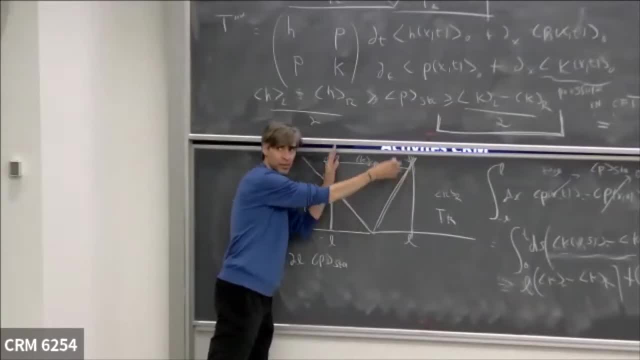 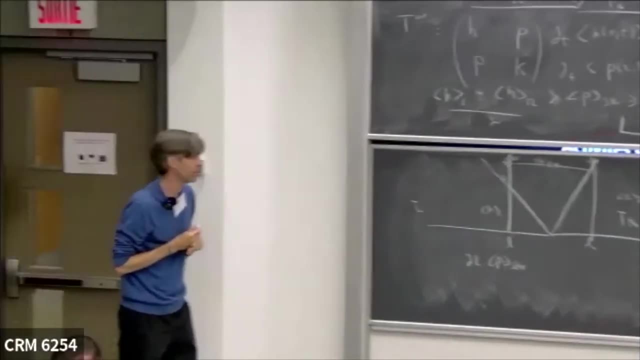 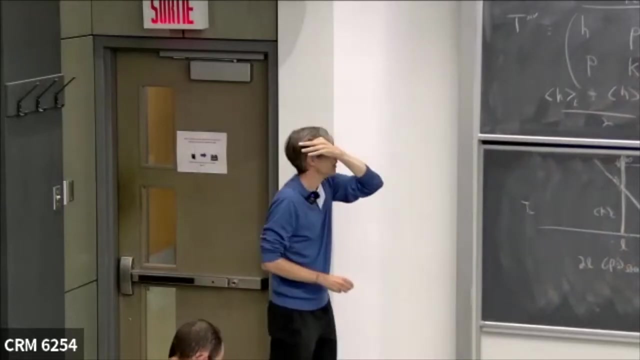 looking new. using the light cone and using a simple idea about you know how pressure should change in space time. You get the non-trivial inequality for the session And the similar inequality you can do on the other side by using the other conservation law for an upper bound. 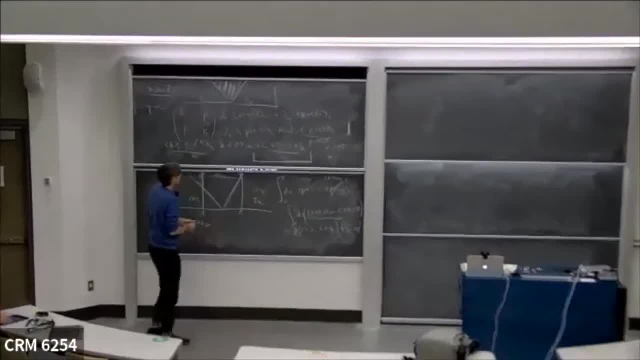 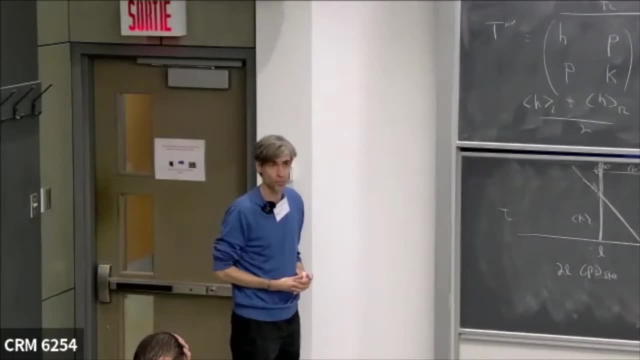 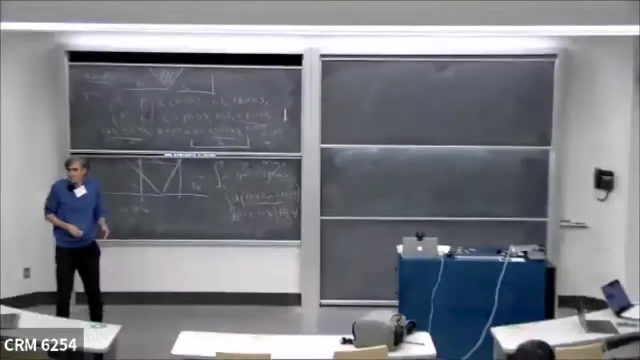 So, you know, the interesting is probably the lower bound. I mean, you must have a current in general. if this general intuition is correct, If you have a difference of pressures on the left hand, Okay, So that's okay. Somehow we're wondering at the beginning about: is you know? 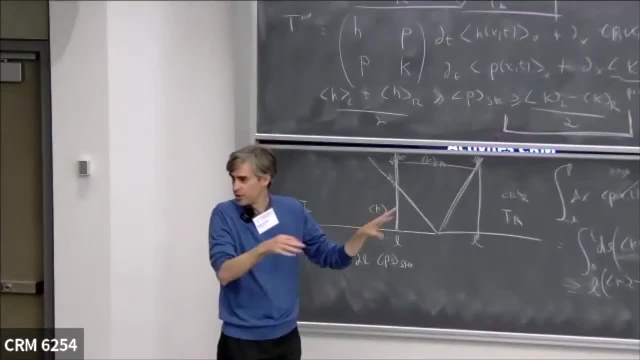 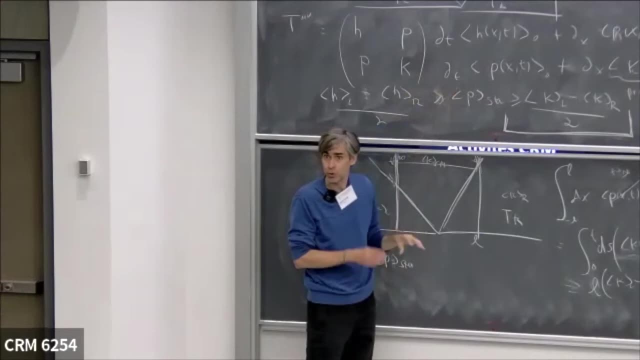 is it a non-equivalent steady state that we get or is it diffusive? and all that and all this right. If you have that structure, relativistic, invariant. look at energy, It is not diffusive. You have a true, non-equivalent steady state emerging. 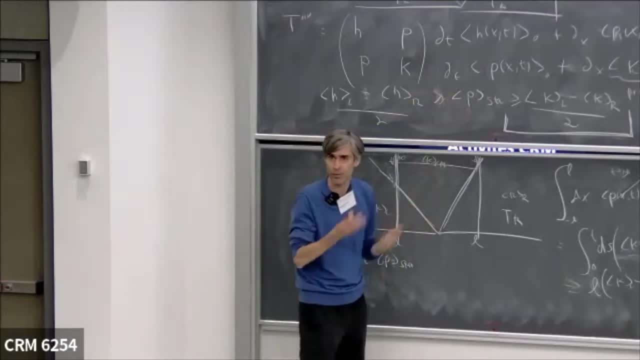 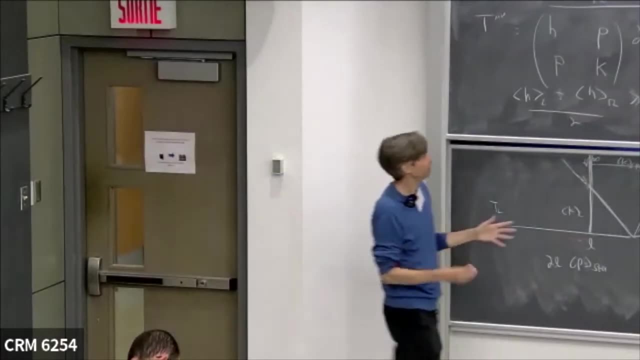 You must have a non-zero stationary current And so it's not time reversal invariant and all that Okay. So this is showing that you must, that you have ballistic transport in general, when you have a relativistic invariance, I use: P equals the current of energy equals. 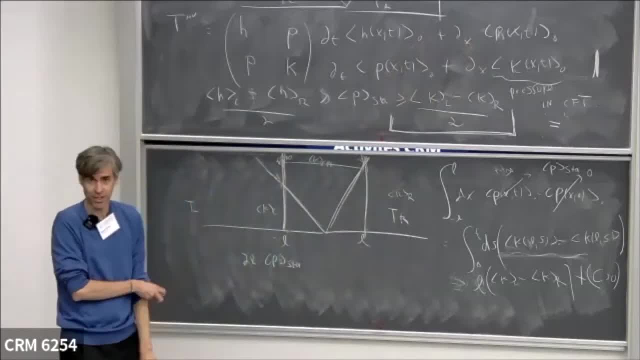 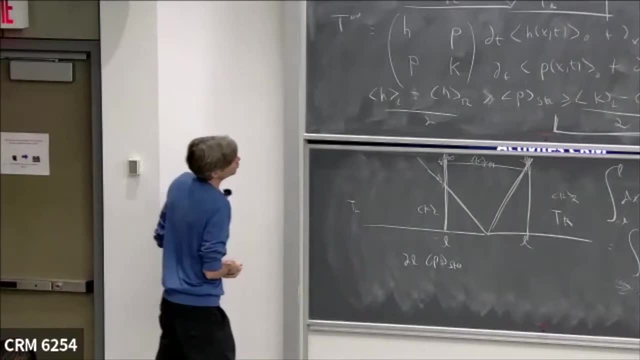 the density momentum. So, for energy transport, relativistic invariance, you have ballistic transport. Okay, It's not diffusive, It is ballistic. So this is actually the general situation Whenever you have currents which are, which are not. 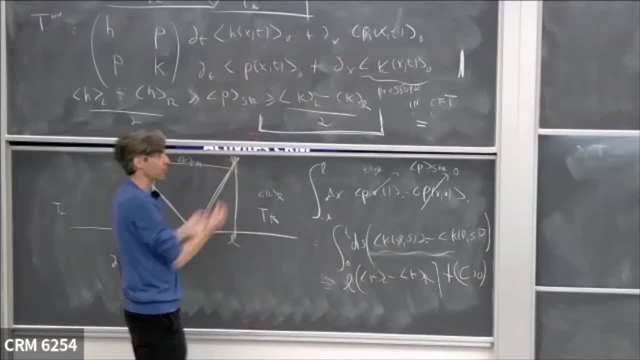 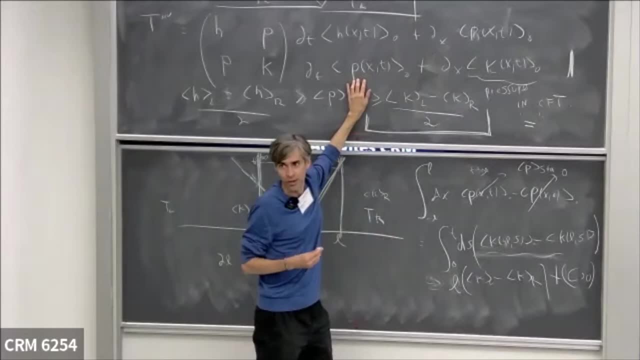 which are functions of densities: constant density with appropriate property, So like if you have densities which are of same type as current, like time, reversal, anti-symmetric, for instance- you mean they don't need to be equal, but if they're the same type, 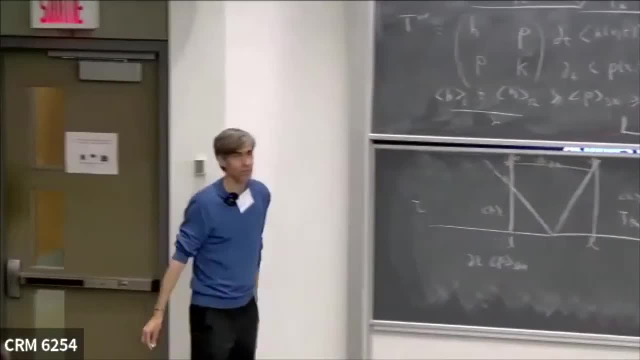 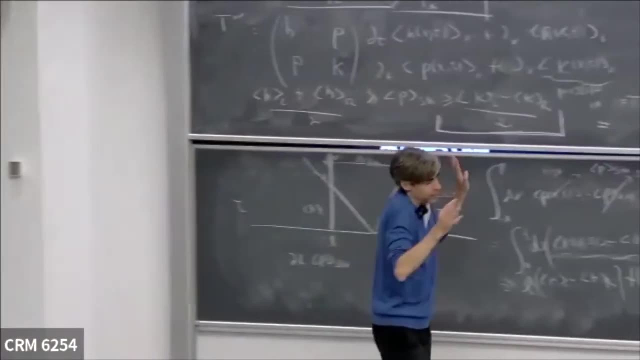 then that would lead to no to non-trivial average values of these currents at our time and ballistic transport Okay. But this is kind of just to show in general. in the relativistic model you must have a basic transport for energy and you have a lower bound for the current. 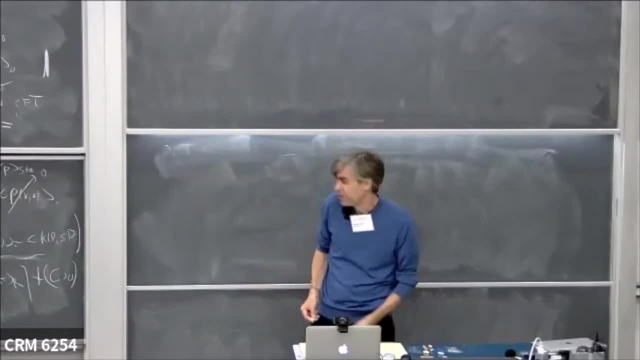 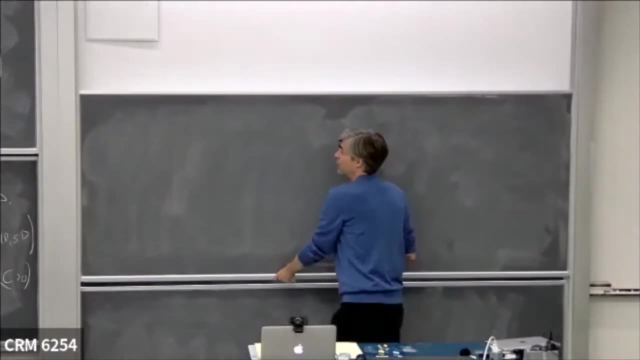 Now, what is, what are these currents, How you calculate them? Okay, It's just a general lower bound, with some some dual idea. You could make it more precise where to calculate precisely what this stationary current is and to get this more. 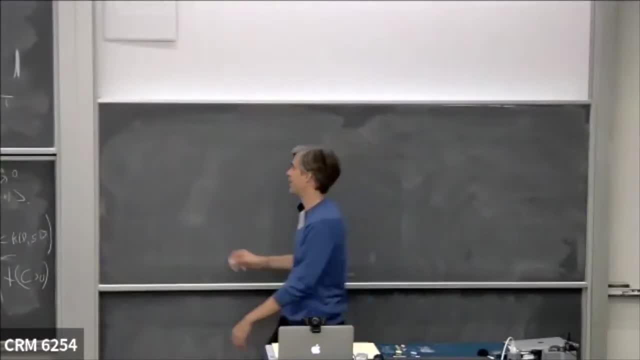 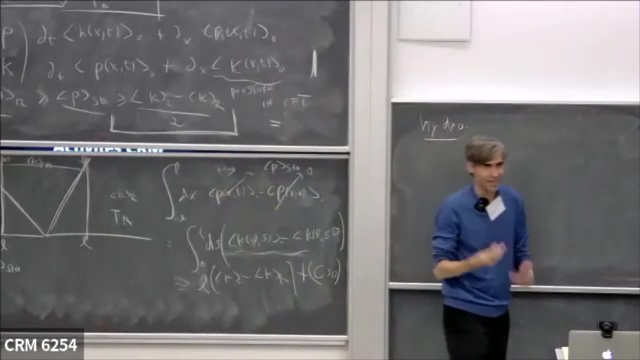 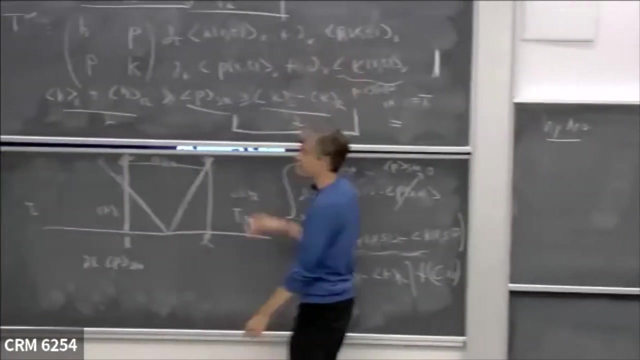 you know kind of more physical about what's happening. what you have to use is hydrodynamics, okay. So you have to consider such conservation loss and say a bit more about this. So release conservation laws at the level of averages after time evolution and say a bit more about these things. 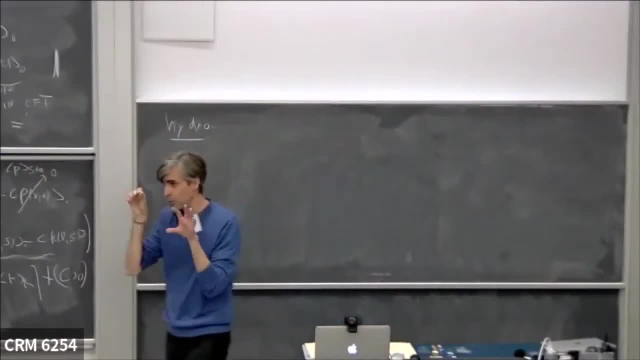 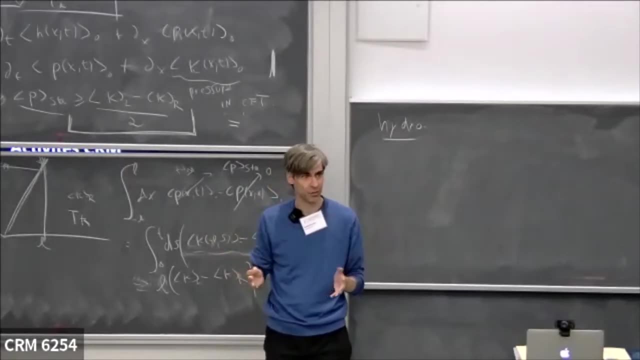 In 1 plus 1 DCFT, we can write. we could write the conservation loss for the fundamental observable themselves, the microscopic observables, right, We'll write specifically and solve that. No, it's very, very simple, But in general it's complicated. 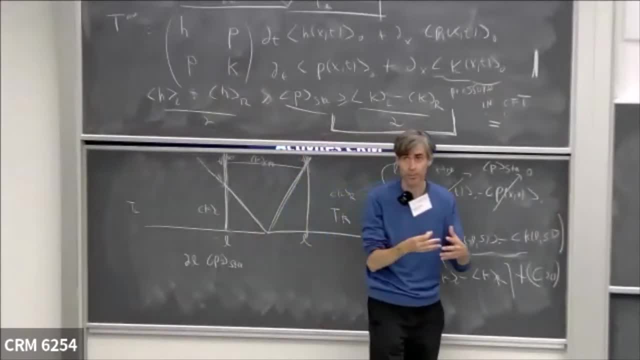 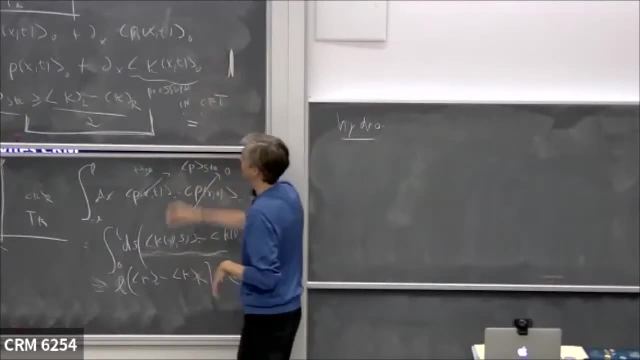 You don't know what K looks like. I mean, the microscopic observables are just complicated. They don't close among themselves in conservation law- okay, But you can write averages, okay. And the idea of hydrodynamics is to just simplify the problem. 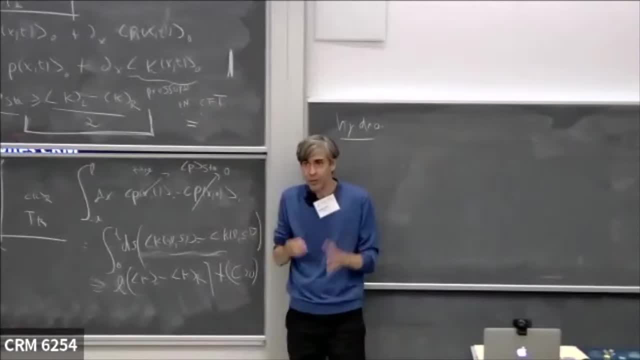 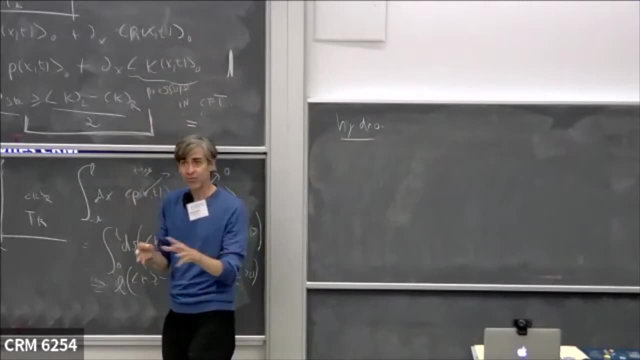 at the level of the averages. And the way you simplify is that you kind of make sure that you close the system of equation. So in CFT we didn't have to take averages to close the system of equation. DT plus DXT equals zero and DT minus the XT bar equals zero. 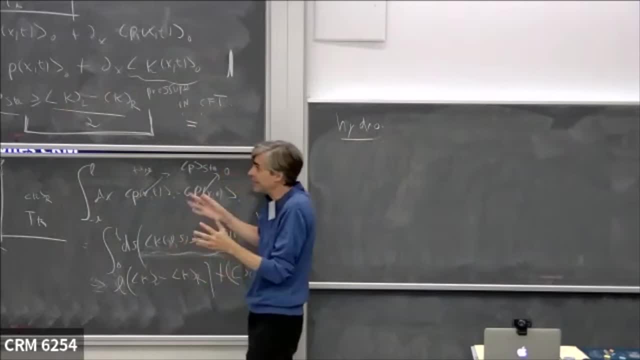 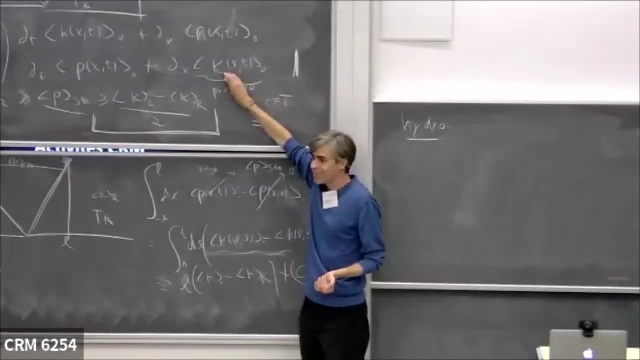 So you close them on yourself microscopically. okay, Just need T and T, bar nothing else. But in general it's not true. K is something complicated, But then at the level of averages, Hydro says that, well, maybe we can write this average. 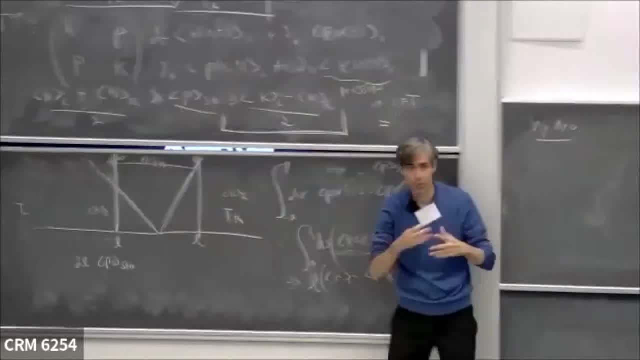 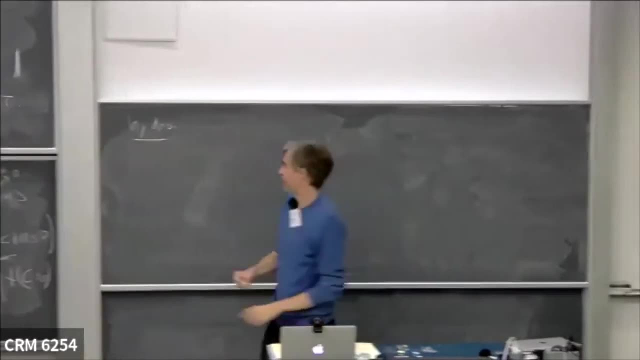 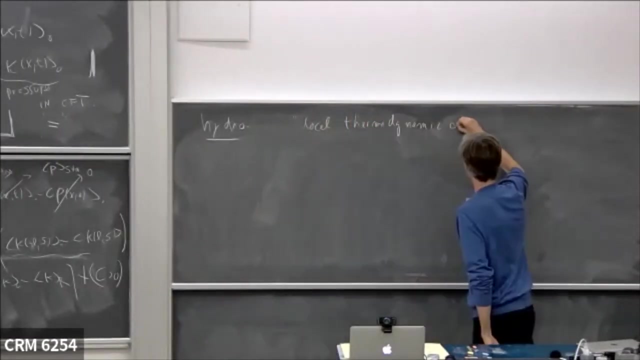 as a function of the other averages that are there, and then close the equation and get something that is tractable. okay, Now, what is the physical principle? Well, physical principle is that it's often called local thermodynamic theorem. It's actually not a very good way to call it. 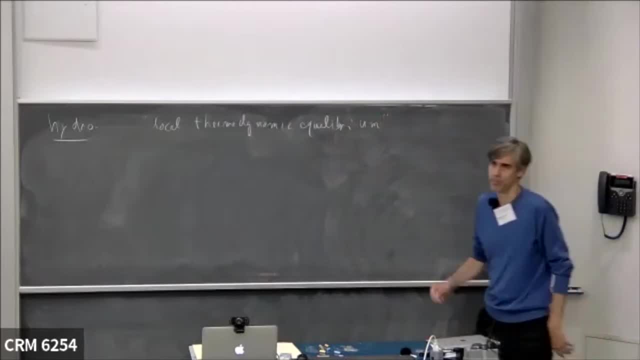 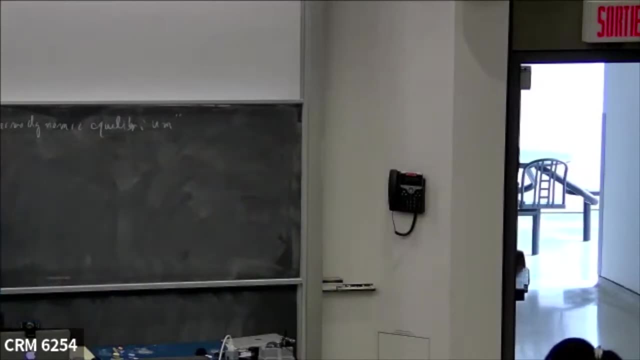 but if you look on Wikipedia, actually you'll find that Wikipedia maybe is not the best, but you might find that in books as well. okay, So what it means? it says that well, you kind of you will want to have. 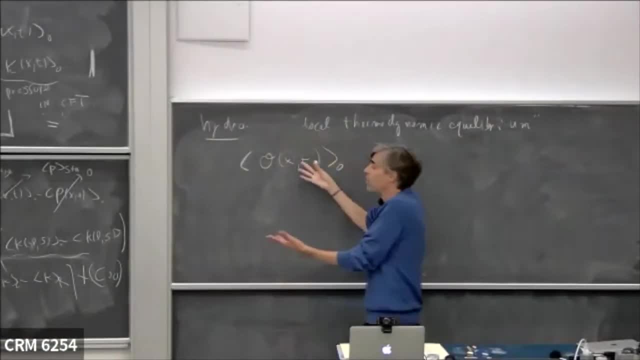 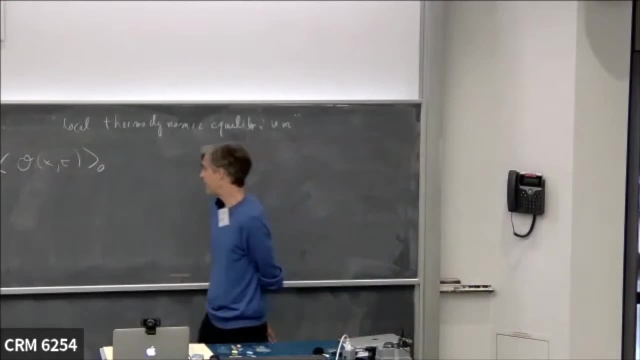 you know, evaluate averages of observables in space-time, evolving space-time, from the initial state, which is that you know T left, T right, initial state or anything else, And so you don't know what it is. but what you see is that 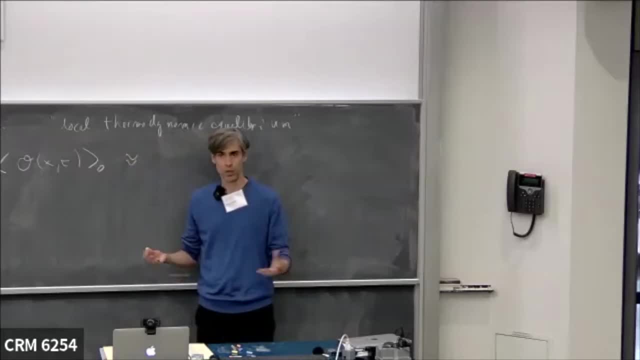 actually this is the many-body system, okay. So things evolve in time, okay. And I'm looking locally somewhere in space-time, I'm looking, say, here or there, you know, And things change kind of smoothly. Like here, the pressure changes smoothly. 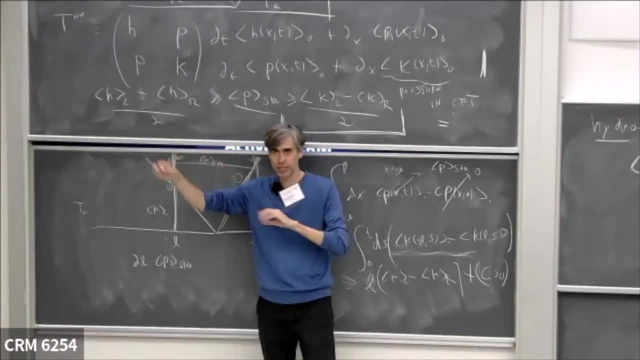 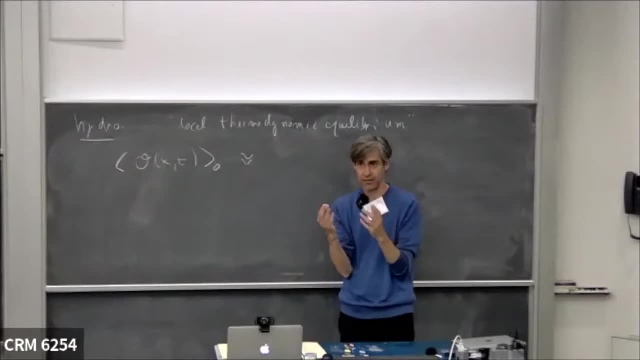 From high to something medium. Things change smoothly in space-time, with luck. okay, Maybe it should change smoothly And so locally it's the state that you see should look like a stationary, homogenous state, something you know that has maximized entropy. 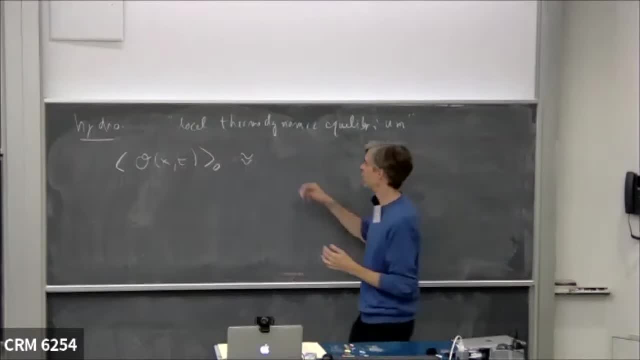 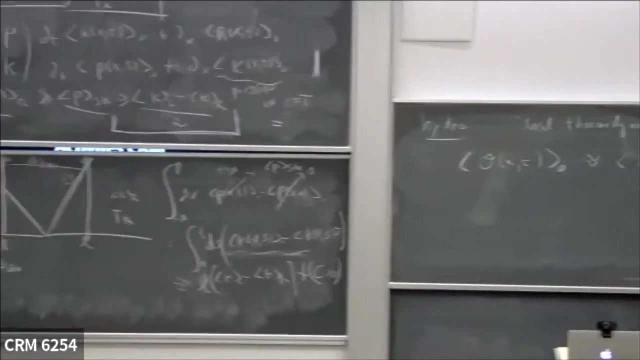 like the thing that we're looking at at the beginning, right? So this is locally, a maximum entropy state. Maximum entropy state at x. yeah, Ah, so this is a good question, Not necessarily, right? You may have a front there. 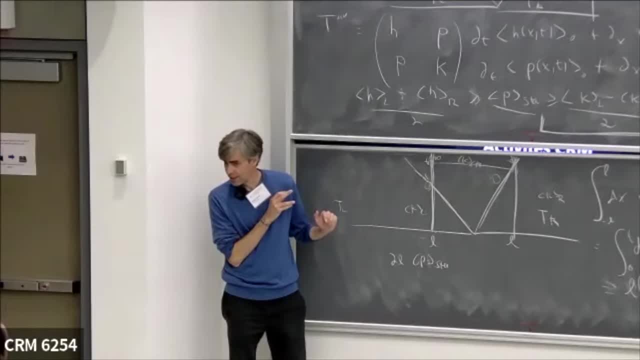 You may have shocks, You may have all kinds of things happening. Yeah, that's correct. So I'm hoping that, like almost everywhere, let's say, but not at the icon in general, Yes indeed, So that will break somehow near the icon. 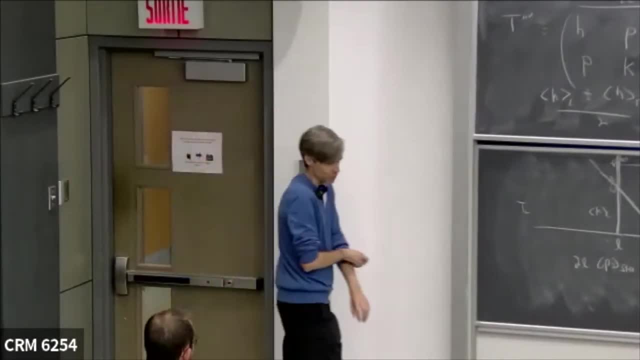 Then we have to consider how it breaks, And this is interesting to consider. how it breaks indeed. Yes, yes, yes, But so I mean that's So. I mean that, you know, will have to be dealt with. 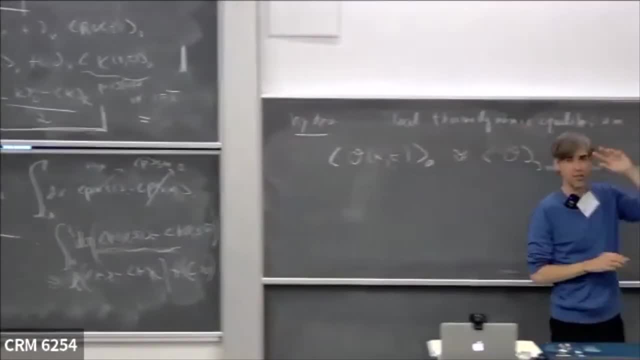 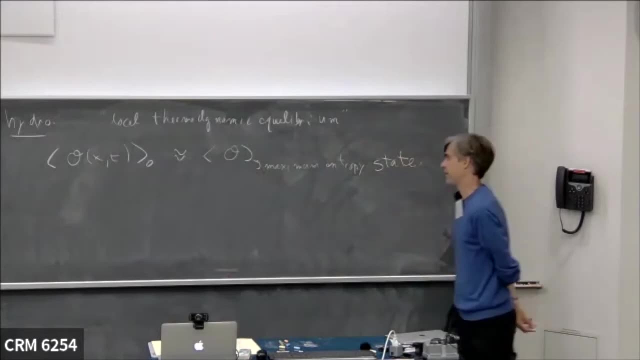 you know this kind of singularity but it can be dealt with. eventually, If it's smooth, nice and almost everywhere, it's actually not too bad. It's okay. we can do something okay Locally. it's a maximum entropy state. 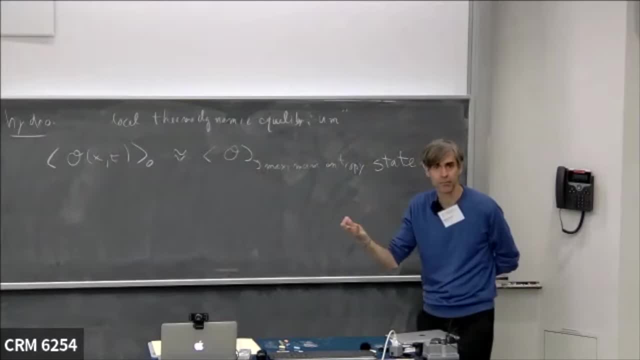 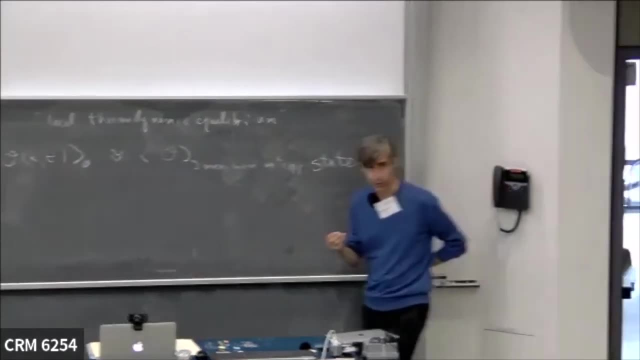 that depends on where you look at in space-time, right? So that's the idea of hydrodynamics. the local entropy maximization. Now we know what is entropy maximization. That means that you know locally we have something like exponential, manual exponential. 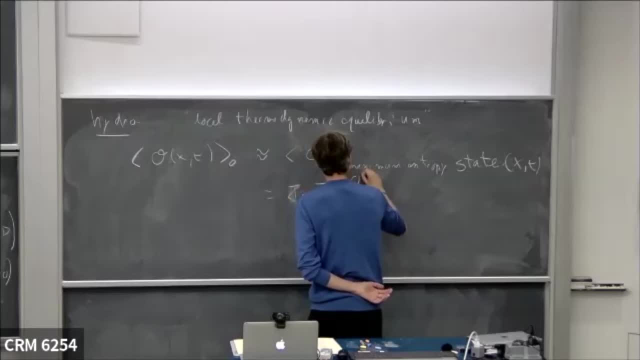 minus this beta-IQI that I was writing at the beginning, right, So all the conserved charges being involved, right, But now the beta-Is. well, they depend where you look. So they depend on X and T, and then you put this observable: 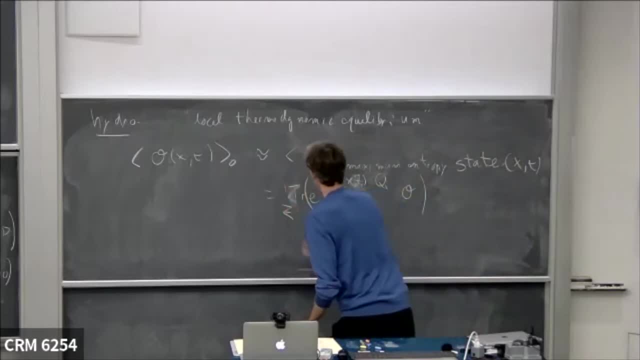 And of course what I mean is always the you know the limit when L goes to infinity. So I look at local observables, I take a density matrix on an infinite space and then I evaluate local observables there. That's my- you know average. 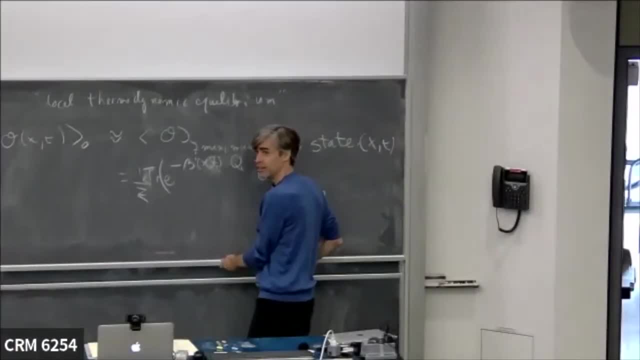 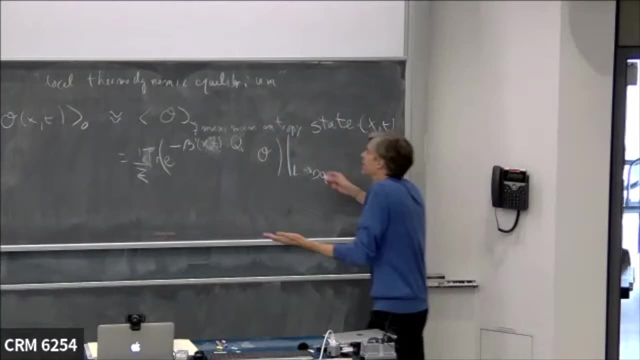 Like the stationary state average. I was doing right. This was an infinite volume average, but just for local observables, for a family of local observables, okay. So maximum entropy: state maximum entropy which respect the conserved quantities, of course. 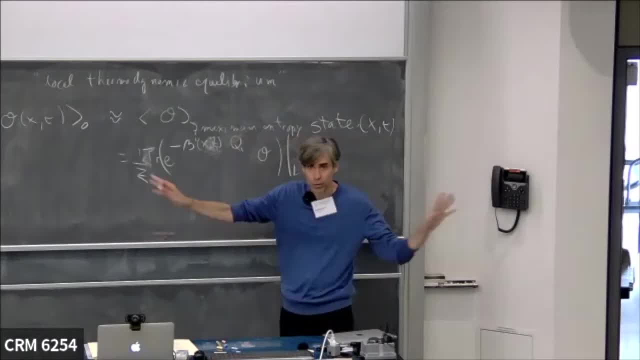 So I need to know where the conserved quantities are, all the conserved quantities- So I have to have some kind of completeness right. So if I miss some conserved quantity, the question I get are just wrong, And that's a typical mistake that people do in this area. 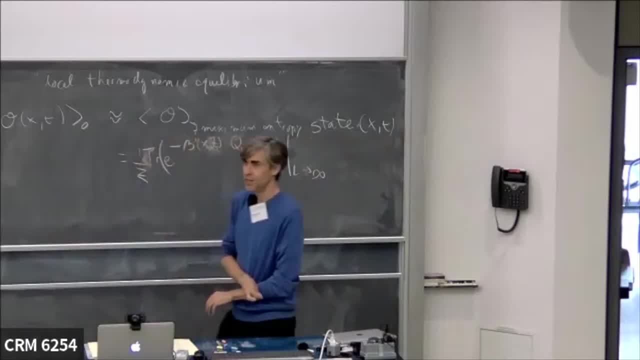 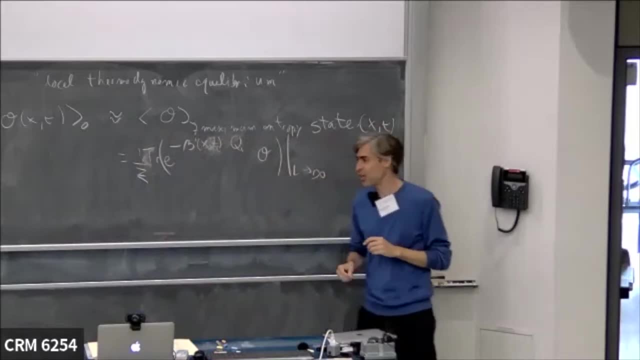 that you don't know all the conserved quantities. you write some equation. it's incorrect, So you have to have them all and it's not completely clear what it means to have them all actually. And in fact, that answer I will. 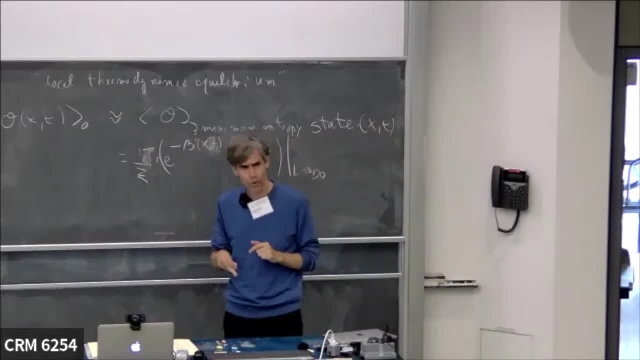 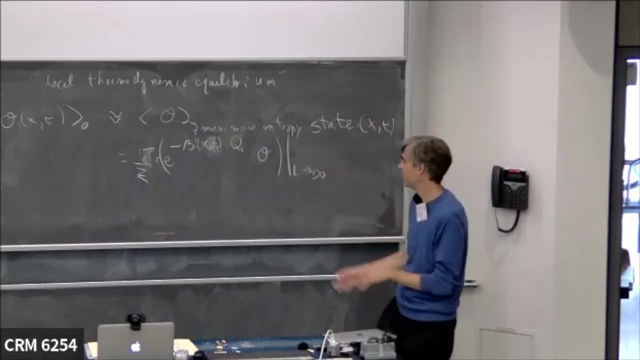 that question I will answer partially in my seminar on Thursday- I think is my seminar- in a slightly different context. but give a partial answer to the thing, not the full thing, but at the linearized level. You can want to give a full answer at the linearized level. 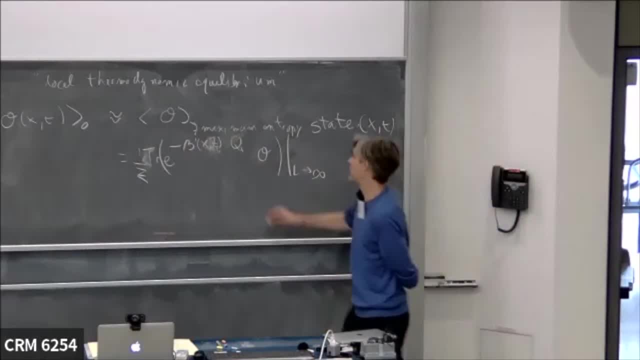 of what are all these conserved quantities? okay, But for now we say okay, so we have to find them out somehow. okay, These are all the quantities that are extensive. That's kind of the idea. So there should be some kind of conserved density. 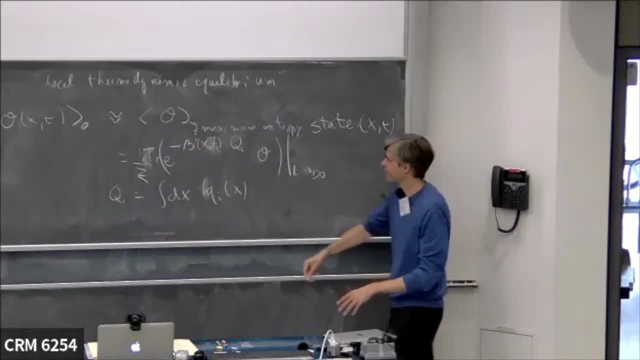 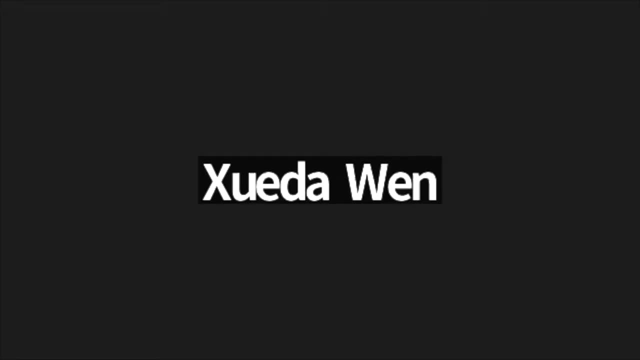 local enough in space or something, and you should be able to write that and then you put that in, okay. So this is the hydrodynamic approximation. It's an approximation should be valid maybe a thousandth of time, when things are smooth enough, and all that. 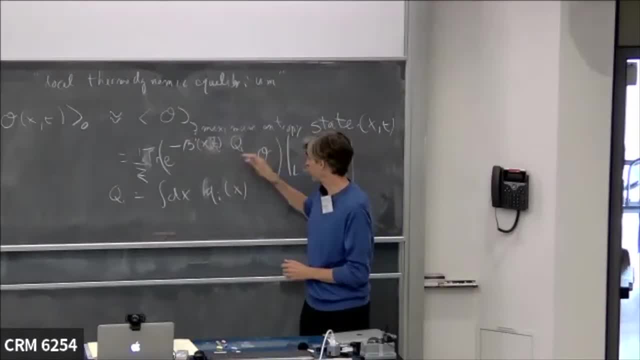 In CFT. this is for the Viradero sector. this is exact, it's true. right There's a jump at the light cone, but in between- this is always true with something that is constant in between, and you know T left, T right, and so on. 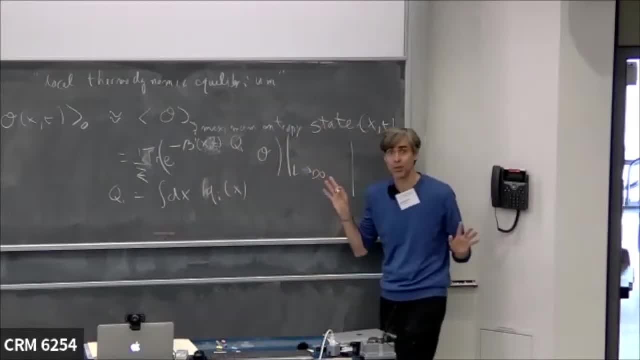 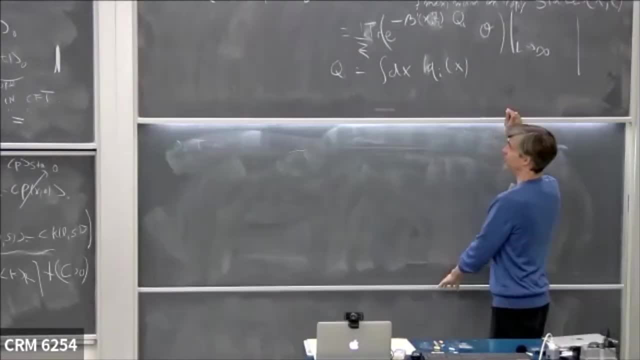 So you generalize that you say: well, let me assume that that's always true everywhere in space-time. This is the hydro approximation and you would like to deduce a dynamics from that. This is an approximation for local observables, but it doesn't tell you how to evolve things. 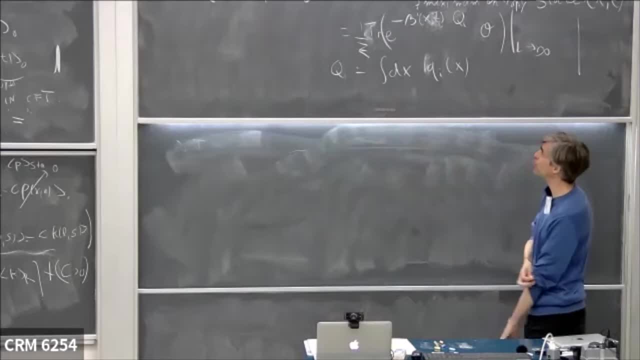 but what it does? it does something very important: that it reduces the number of degrees of freedom to just the concept of quantities, right? So a theory. you have to evaluate all the local observables to know the state. So infinitely many, but a large infinity, right? 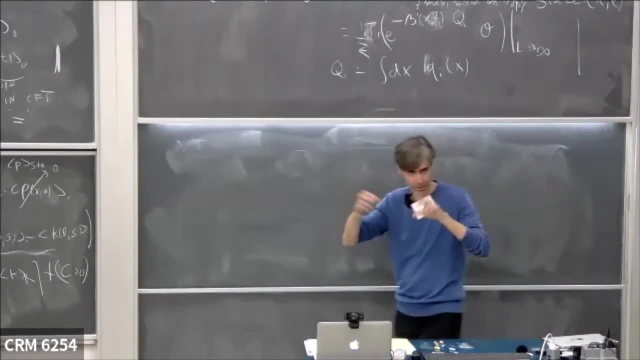 Two to the n, if you have n sites and you know, spin half on each side, something like that, all the. or four to the n, all the local observables. right, There's a lot, a lot of things to evaluate. 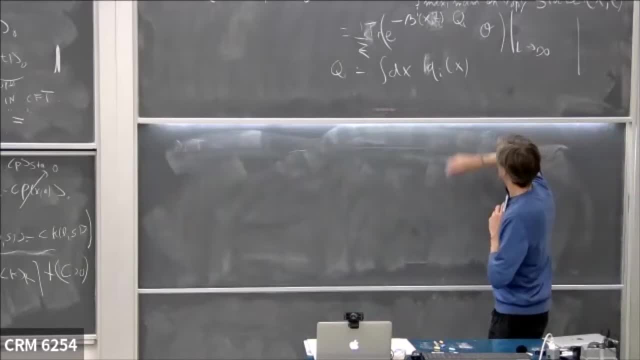 but now you say, well, all you have to do is evaluate. you know, you just have to calculate all the beta i's. you reduce the degrees of freedom. is the beta i If you have three conserved quantities, like as is typical of a relativistic invariant? 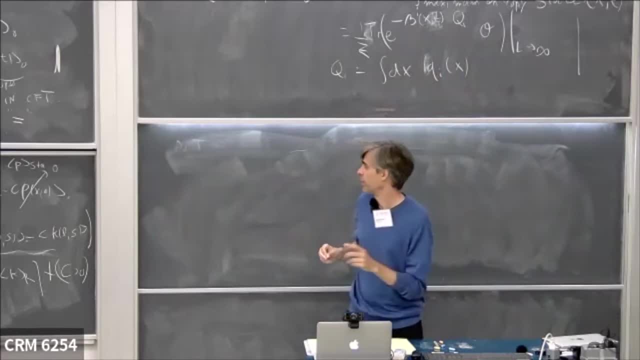 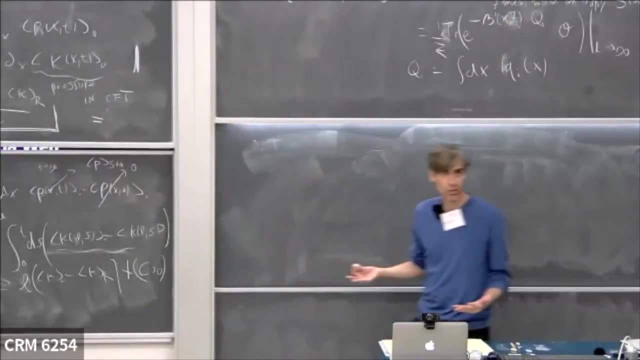 non-integrable systems, because you have. well, you actually have two. sorry, Galilean, you'd have three Relativistic. you have two: the energy and the momentum. that's it okay. So you just have two conserved charge. 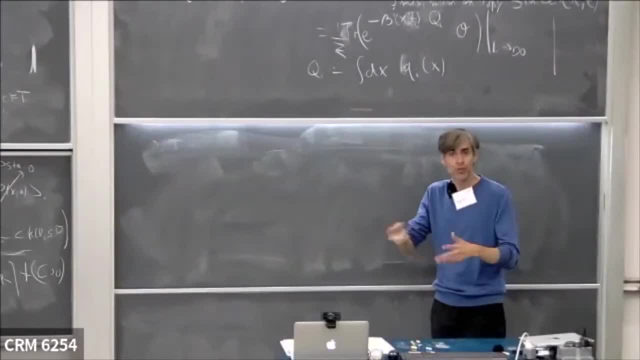 put there the energy and the momentum, and that's it. So you reduce a lot. two functions, right? Two functions of x and t, And okay, so that's rejection. Now what dynamics do you write? Well, the dynamics is very simple. 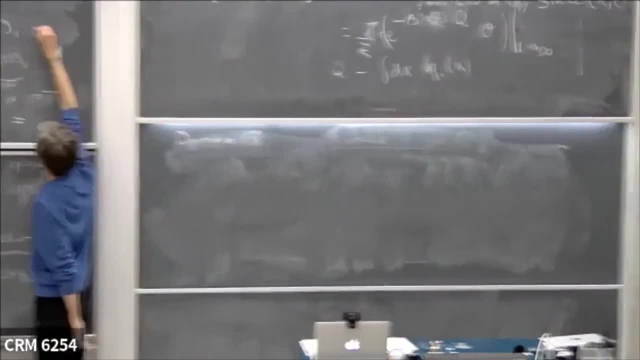 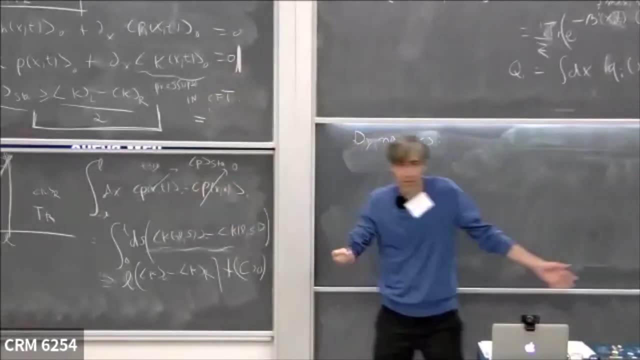 Dynamics is the one that I've written there to get these. I had forgotten equals zero was here, right? Sorry about that. Equals zero, Dynamics is the same as I had written there. okay, It's the conservation equation, right. 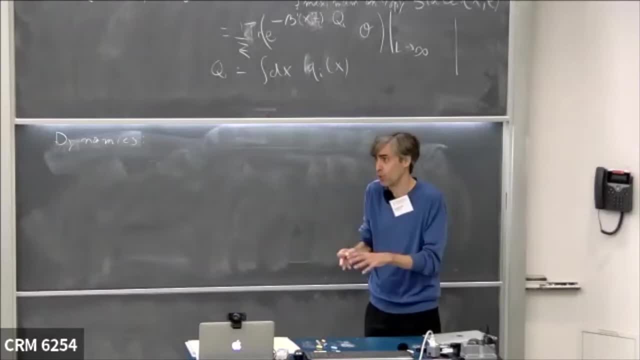 So, of course, conservation equations are true always, macroscopically and anytime, anywhere in time, space, time, no matter the initial state. it's a true thing. It's just from the dynamics, So from the macroscopic dynamics. 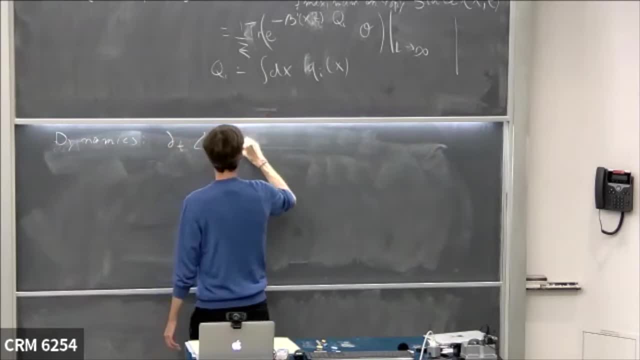 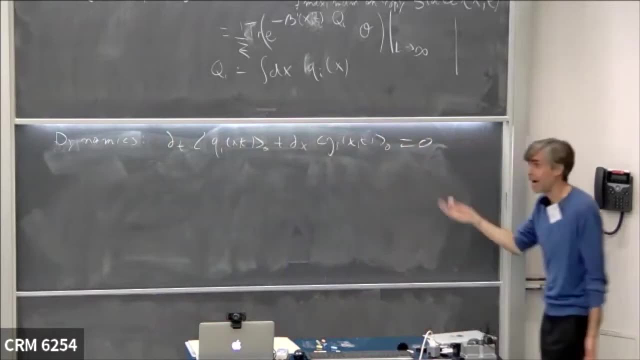 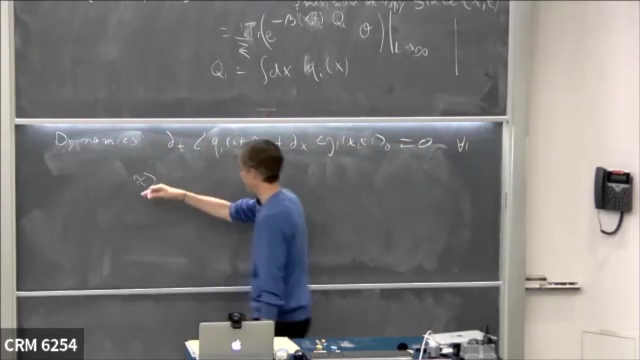 We have dt of qi initial state plus dx of the related currents. That must be equal to zero for all i's right, For all the conserved that you have for all i's. And now you use the- let's say approximately imply, as I think. 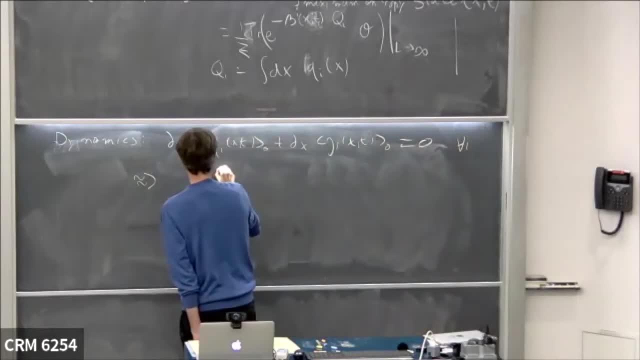 the algebraic approximation. So this is now dt of qi in this maximal entropy state. So that depends on the betas of xt, Okay, Plus the x of ji that depend on beta of xt, And that must be equal to zero. So now you have as many equations for i's as you have betas. 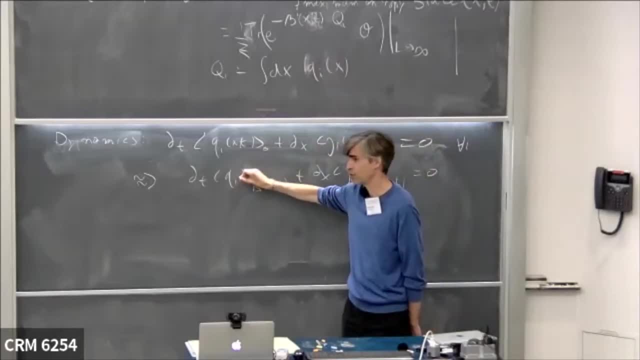 Okay, That's all right. right, So you have as many, because you have a question for every conservation law and you have a beta for every conserved quantity. So you have as many equations as you have unknowns, and that's your system of equation. 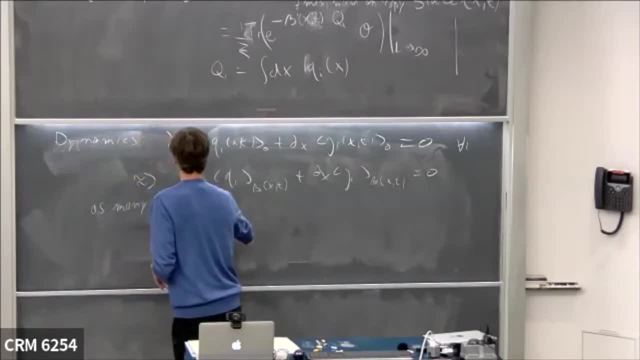 As many. this is kind of important equation as unknowns, and that's your system of equation And that's unknown function. These are the Hadrow equation. In fact, these are the earlier scales, the earlier Hadrow equation, It's the earlier Hadrow dynamics. 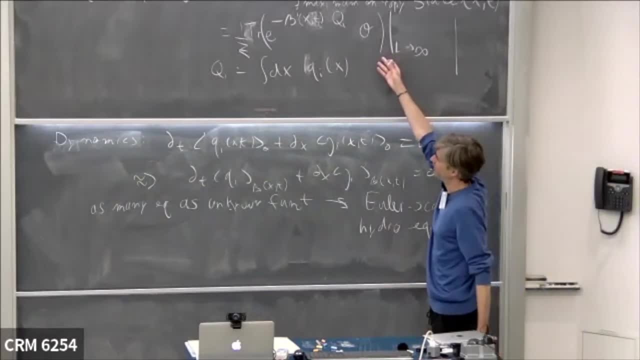 because I have made this very strong assumption that there's local entropy maximization, full maximization, In fact, in reality is not quite true. You might have additional terms and full Hadrow dynamics is actually a derivative expansion, So you add the higher derivative terms there. 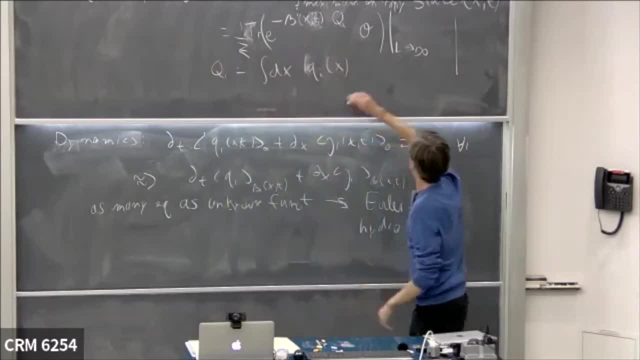 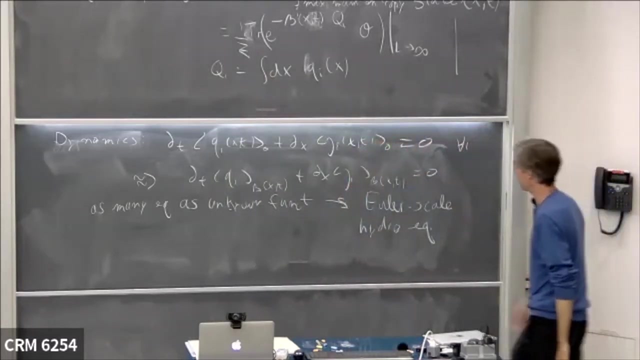 So the average observable is not just that, it's that plus derivative of beta, And what are the higher derivative terms? Then you have to use Kubo formula and our kind of formulas to evaluate that. But that's kind of another story. For now I just have the little Hadrow dynamics. 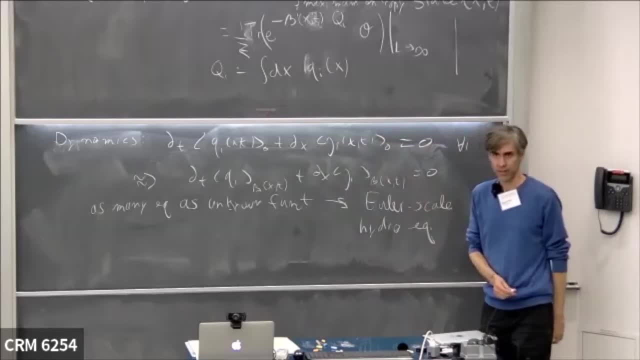 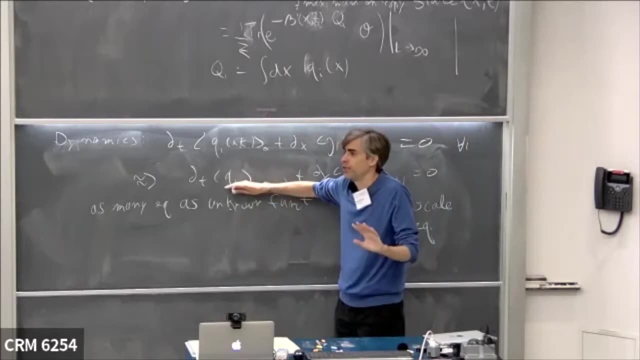 This is it. These are the equations that you want to solve. Okay, So now you just put your. you know your initial condition, you know QI on the left and on the right. you kind of know what it is. 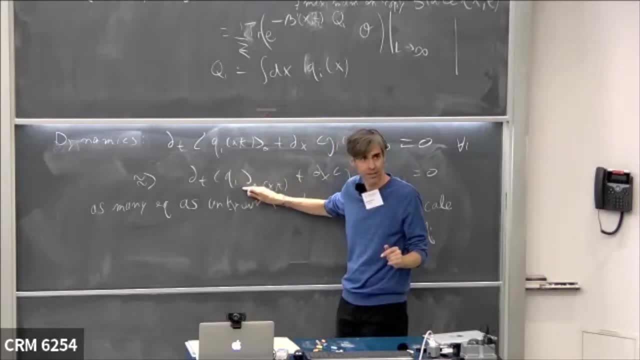 Suppose you can calculate, you know average and equilibrium states, okay, And then you put that in here and you solve it. What's important is that the currents here. you have to write them, you have to know them in maximal entropy states. 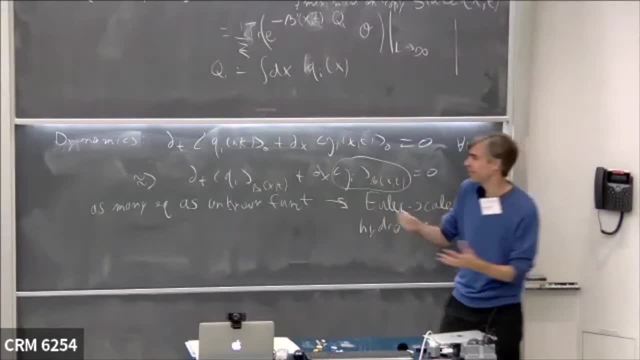 in these equilibrium states, But they're not necessarily equilibrium, by the way, right, They could involve the momentum and all that, but there's maximal entropy states, okay, So you have to know all the currents and all the densities in these maximal entropy states. 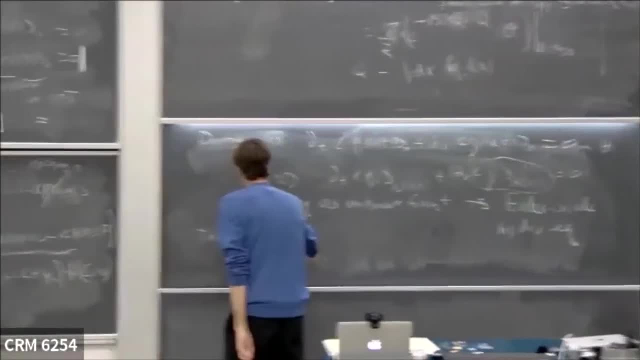 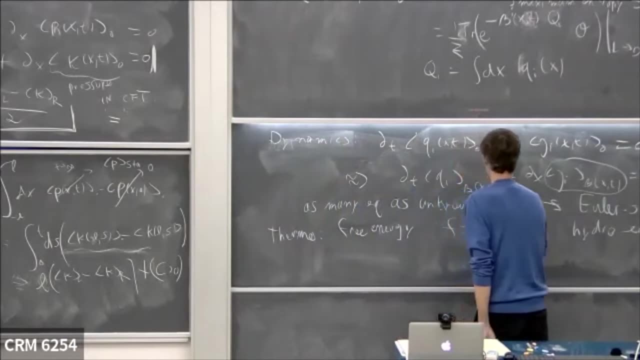 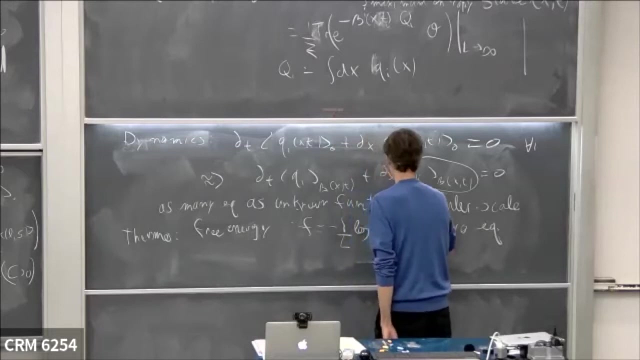 Now, of course, from basic thermodynamics. if you know the free energy which you can often calculate, the free energy which is F equals no minus one over L log of the partition function at L goes to infinity. This is the free energy density, okay. 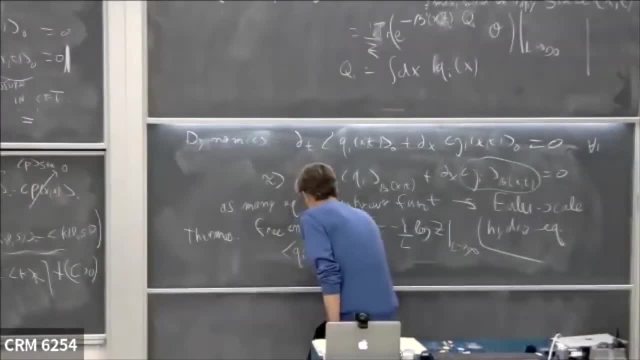 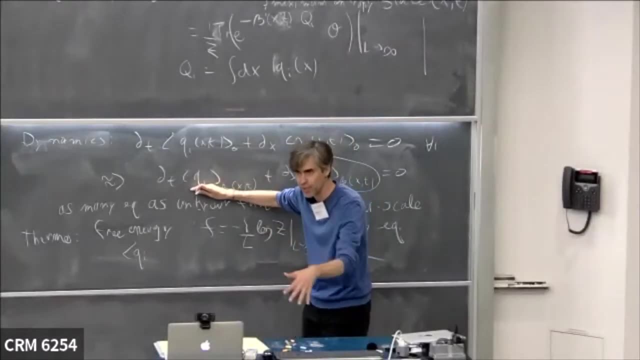 Well, you can calculate then the average, you know the average densities, QI at any point in space-time. this is now a maximal entropy state, is is a. it's a stationary because it's involved, the constant quantities, and it's homogeneous. 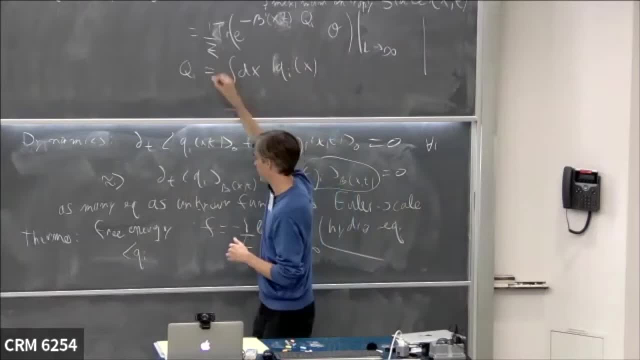 because constant quantities are homogeneous. that's all okay, I can put that in any point. So this QI in this maximal entropy state is nothing else but the derivative of F with respect to beta I. So okay, so if you know the free energy. 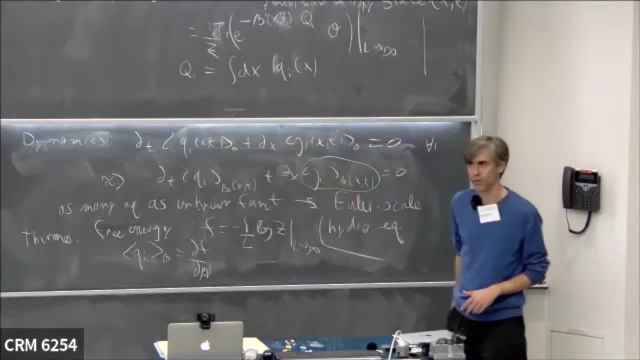 in terms of all the betas, and sometimes you can calculate that. well then, you know well the average densities. okay, But what about the JIs? Well, you don't know, you don't know. there's no partition function for the current time. 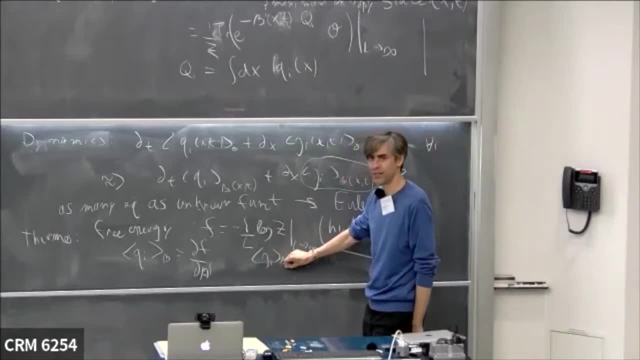 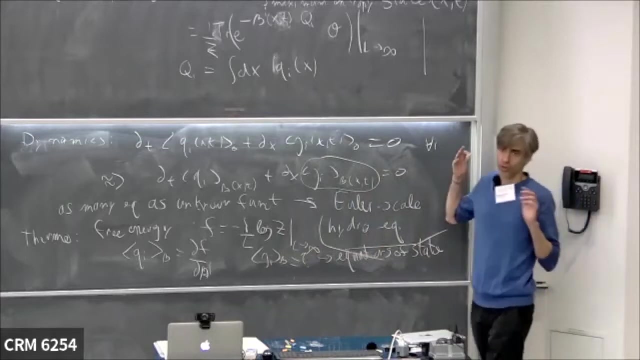 So the JIs a function of betas. this is a non-trivial thing that you must know. These are the equations of states. These are the things additional to standard thermodynamics that you must know in order to do hydrodynamics. 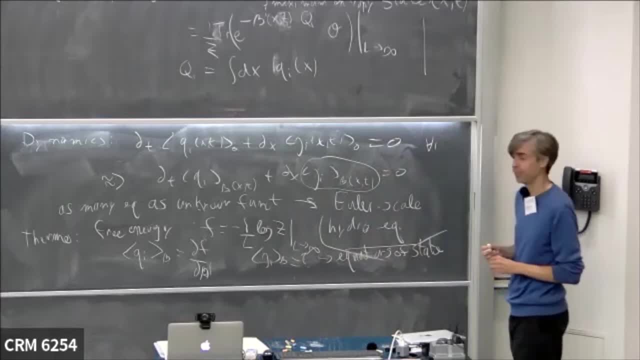 or other, hydrodynamics, okay, The currents, the average currents, okay, In CFT we knew the average currents because, well, one of them is the density right, The momentum momentum, and because, by tracelessness, the other. 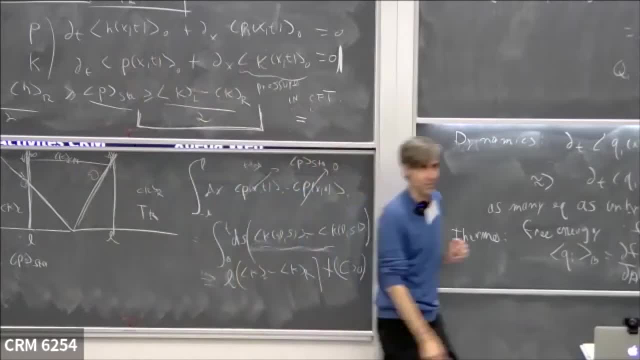 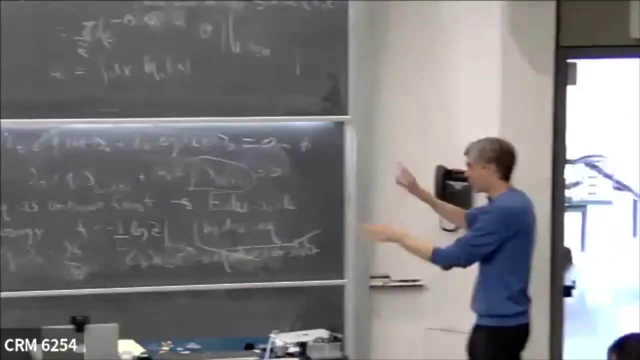 the pressure was also just the energy. okay, That's in CFT, But in general then you don't know, you've got to calculate it, okay, So there's data. So this is the general kind of setup, going beyond CFT. 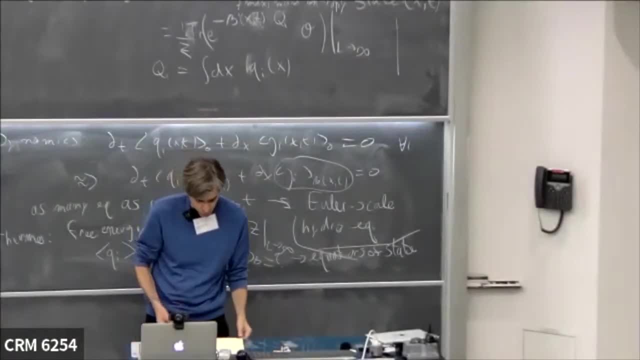 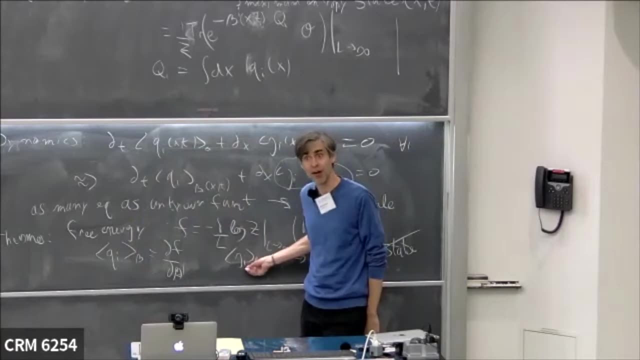 in order to solve this problem, So this kind of initial value problem using hydrodynamic idea. okay, Well, it depends how lucky you are If maybe you can calculate them exactly somehow. If you cannot, yeah, you've got to model that. 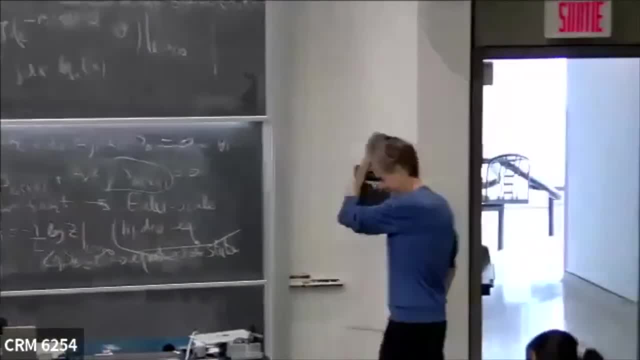 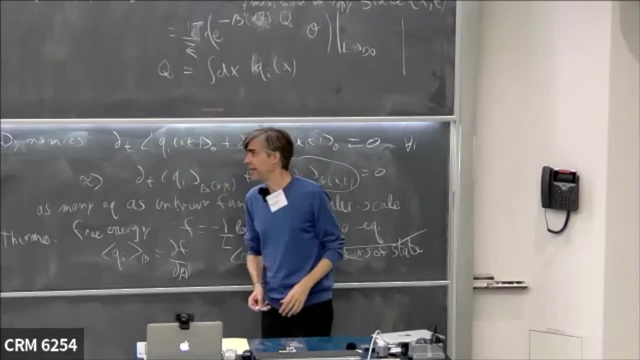 I mean, yeah, they're, let's see. In fact, in fact, if you know the free energy function of all the betas, then there is a general result of ours. Maybe there are some results before also, I don't know. 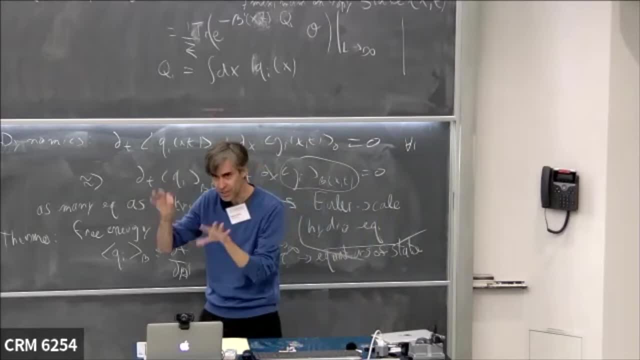 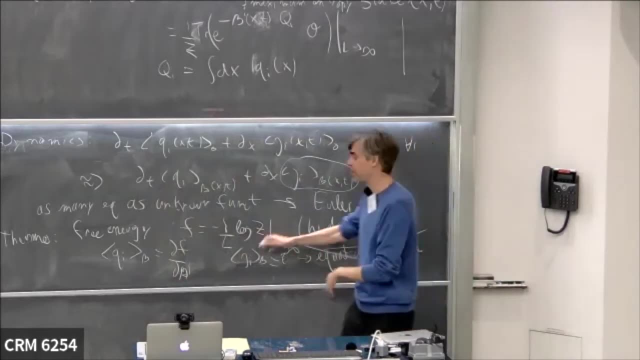 But if you know that, if you just have two or three consequences, well then actually you can calculate which is, in fact, it's okay, It's not too bad, You can eventually get that. For instance, you can use the relativistic variance. 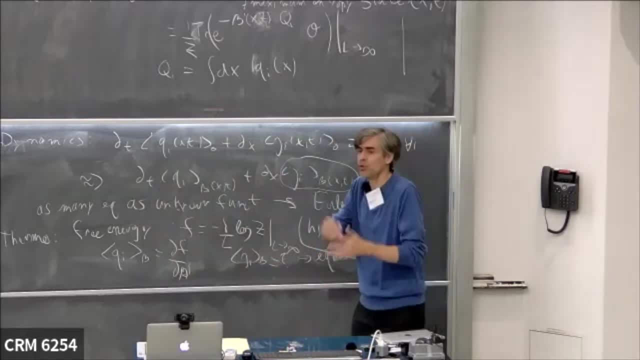 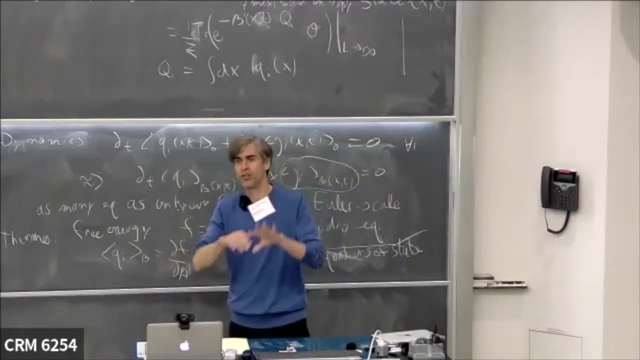 now that stuff and then you can calculate, For instance in typical Galilean system the pressure. no, even in relativistic system the pressure is equal to the free energy. This is a general thermodynamic relation. Pressure equals F, you know. 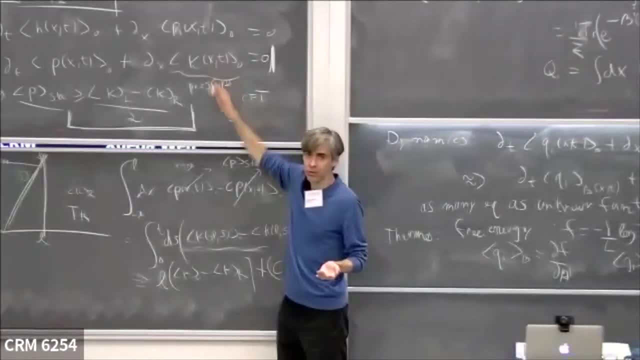 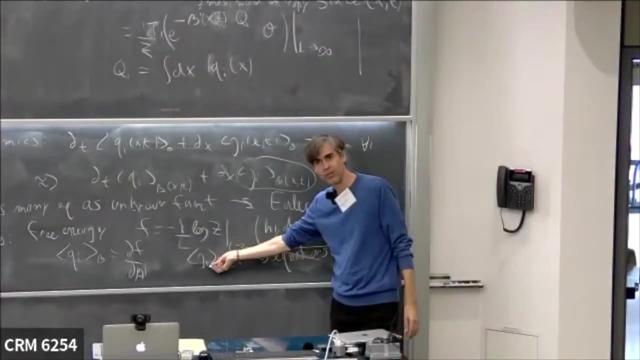 And the pressure is nothing else but the momentum current. So that's it. So you have it, you know, Actually it's not too bad. but, this being said, this was not known in integrable systems, because in integrable systems, well yeah. 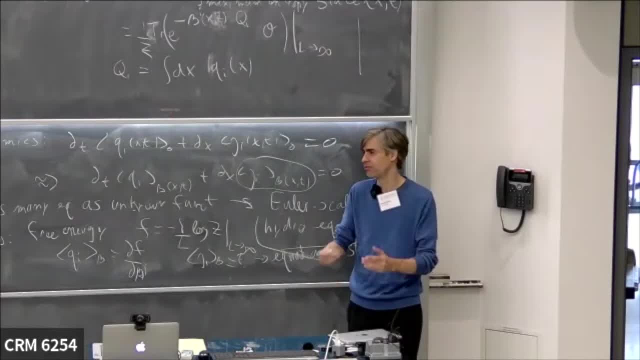 the pressure is in the density. but then what about the current of the nth concept, quantity, which is some weird thing. you know Why? you don't know how to calculate, So people didn't know how to calculate that. So here this is. see, this is a general formalism. 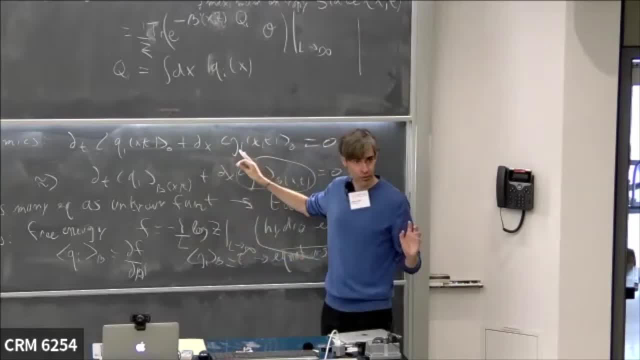 and it should be applicable no matter how many concept quantities you have and what they are, as long as you put them out. Okay, Then that should be the correct thing, And once you have that, if you can calculate the currents, then you have your equation. 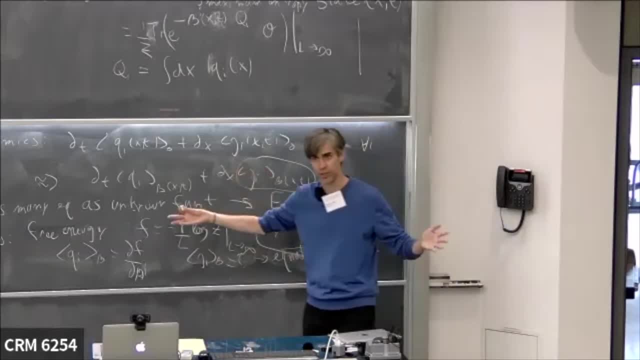 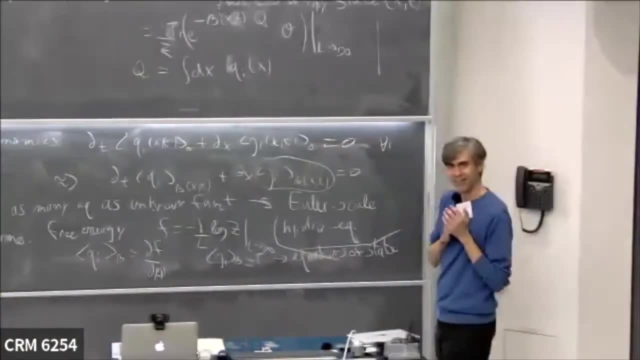 That should be the correct large-scale description of your system. It's large-scale, right? It's not microscopic, but large space-time. it should be correct. Okay, That's the general idea, right? So it's kind of a very powerful idea in the sense that 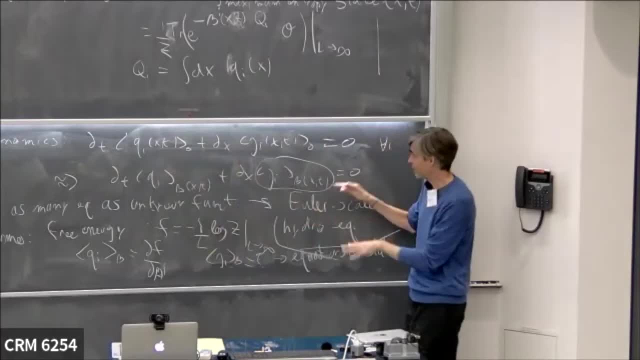 you see, for Hadrow dynamics, Ehrlich Hadrow, you don't need chaos or anything like that. It's not about thermalization Per se. it's not that. It's about relaxation, about the system that relaxes locally to something. 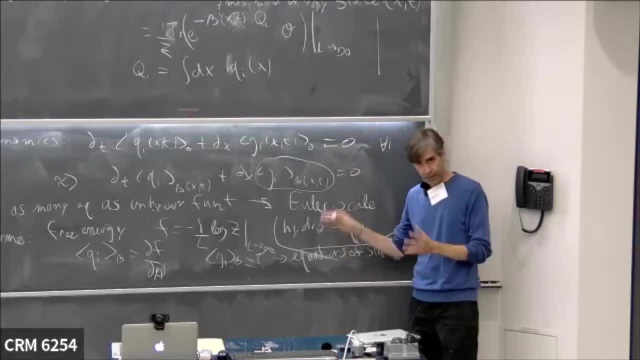 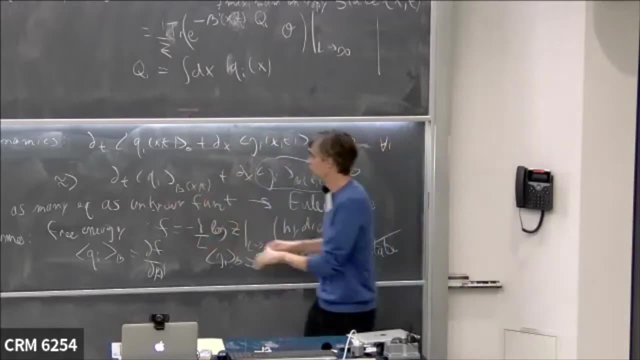 And if you know what, where it can relax to, then you can write an equation. So it may be that the it's a manifold. actually, I mean, it's not completely understood, but somehow these concepts point to be that they're like 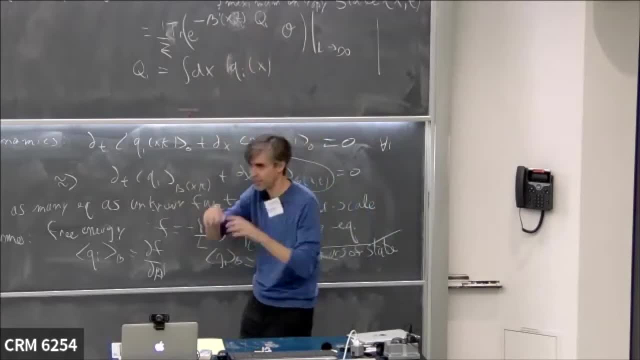 they're like a tangent to the manifold, The beta's kind of, you know, renew along the manifold of all the states and all that. So this manifold of states may be very large, It's infinite dimensional, or very small or whatever, But whatever it is, once you have it. 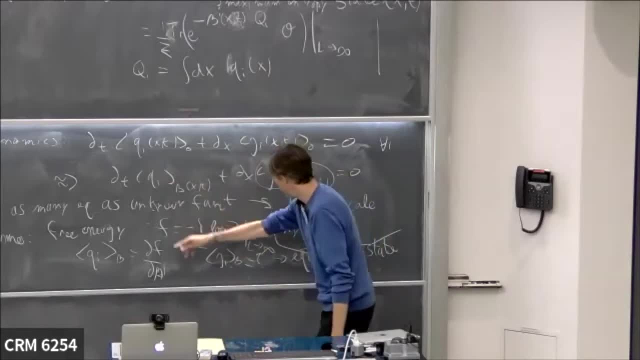 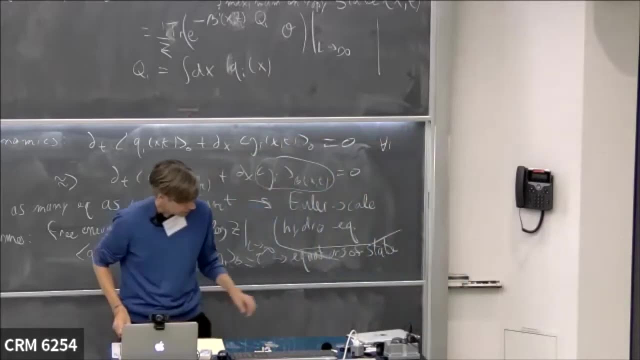 once you have its structure and the density and currents, then you write this and you have the large scale equation. It's interesting, You can even do that for free models. So let me just see what. yeah, So, and I want to give some examples. indeed, 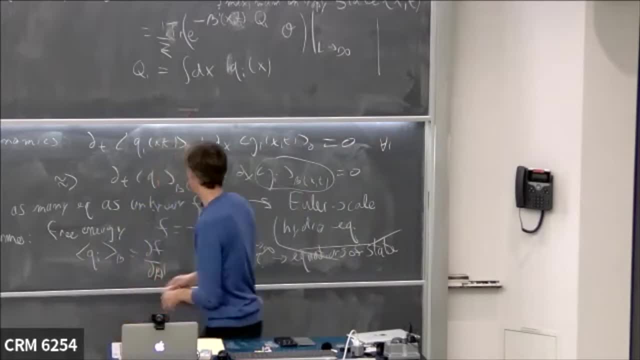 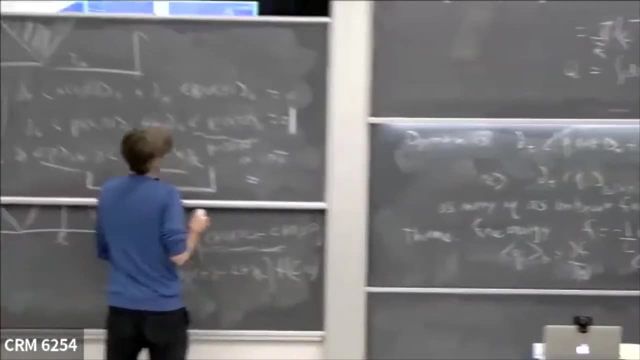 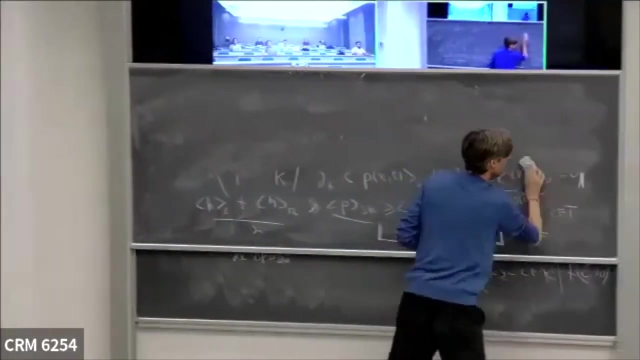 of how this works right. So there's a few things one can say actually before that It's very interesting and it's a very beautiful theory that I think should be taught in basic courses- I think at university- but there's a lot of nice relation that emerged. 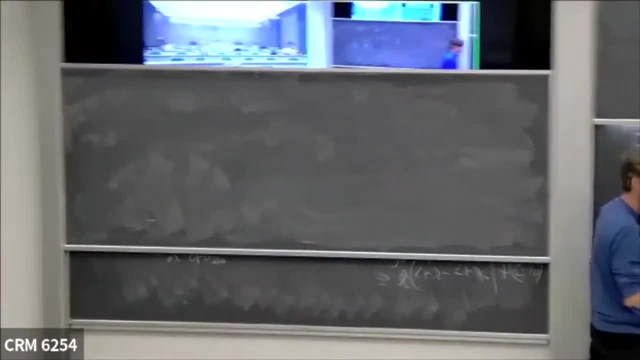 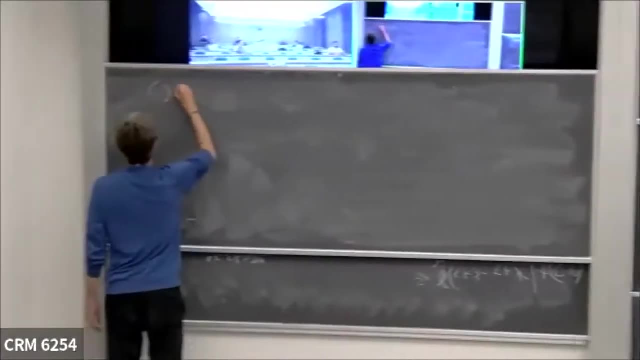 from this earlier tidal dynamics. okay, So the first thing, before I give the example, I'm going to use some example, but the first thing is: what is this equation of state right, The current? So usually, I mean very often. 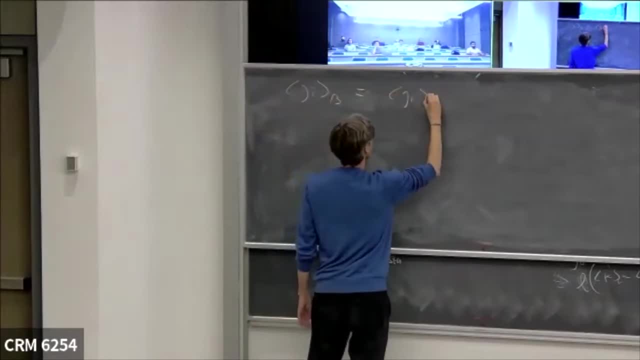 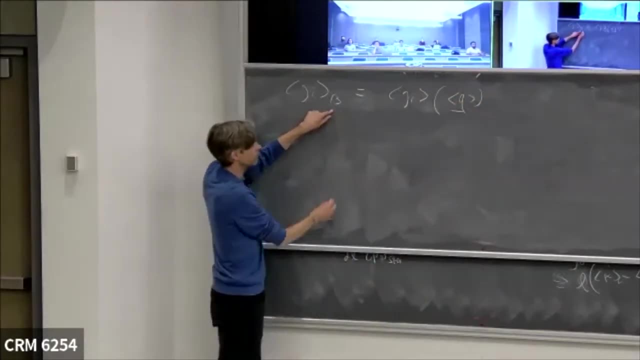 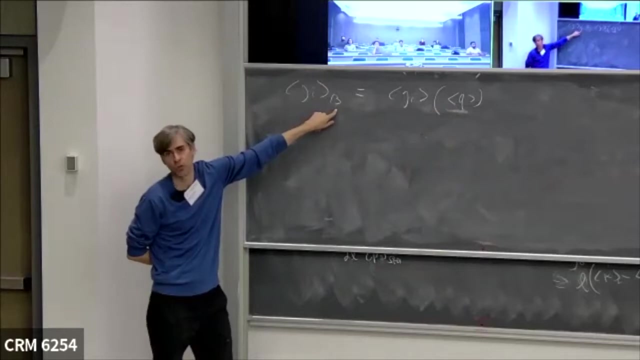 this is actually written as a function of the average density, right? So instead of the function of the betas, I put: well, it doesn't matter, It's a function of the betas. The betas are not natural, not so natural physically, right. 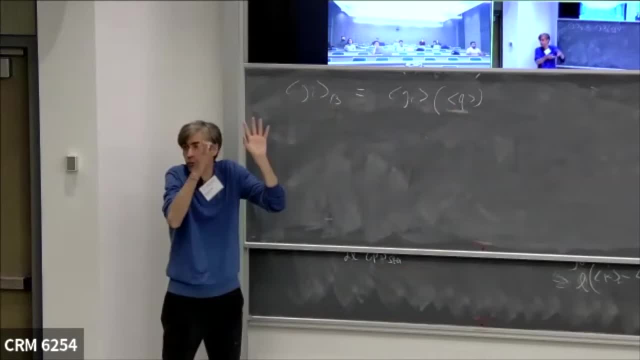 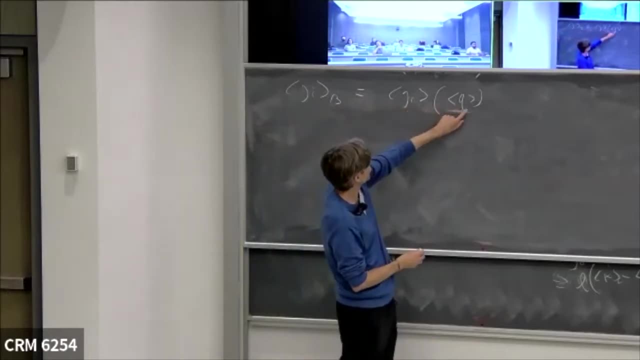 So the average energy is more natural than the local temperature, which is kind of a bit weirder to define something. So the average energy momentum and all that, So you can write a function of the local densities. That is, there is a- it's a bijective map in the appropriate 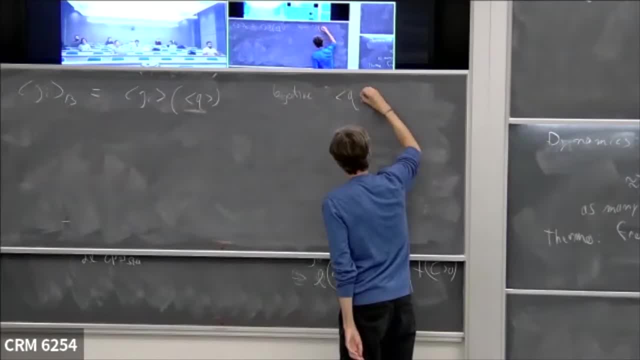 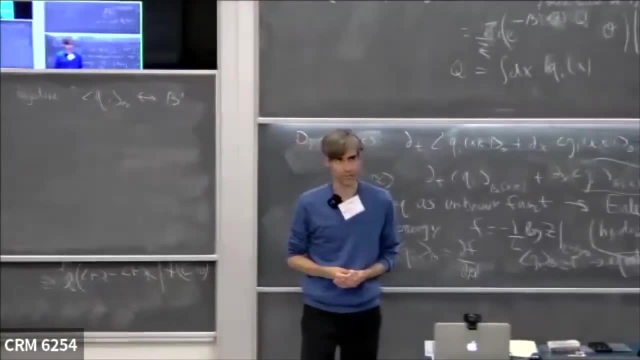 at subspace between the QIs and the betais. It is a bijection between these two things. okay, In fact, locally, the fact that it's a bijection is not too hard to see. And one thing that you do. 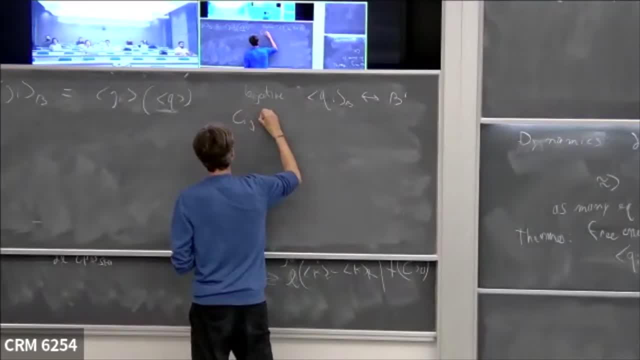 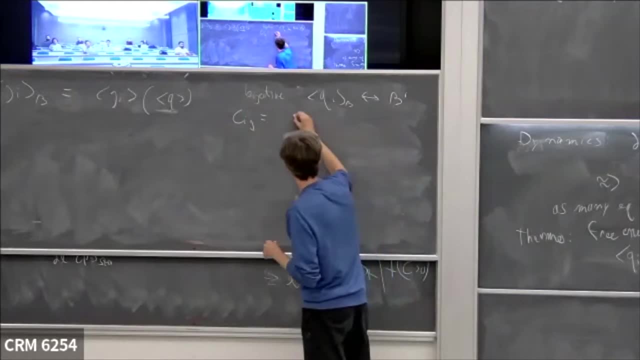 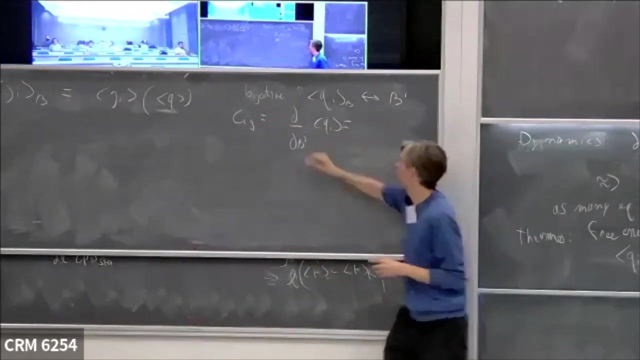 you construct the so-called C matrix, which is a static correlation matrix. It's just a susceptibility matrix. So all susceptibility. so this is just the derivative respect to beta J of QI. okay, And me with a minus sign. So you just bring down the total Jth concept quantity. 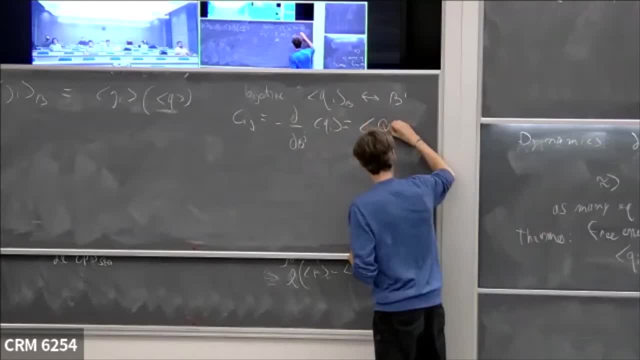 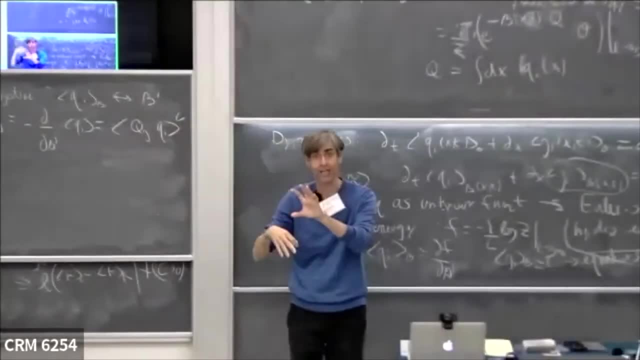 when you do that. okay, So that's just QJ, total point of concept, quantity, QI, And it's a connected correlation function because when you take the derivative, there's a betas in the numerator and denominator because of the normalization of the state. 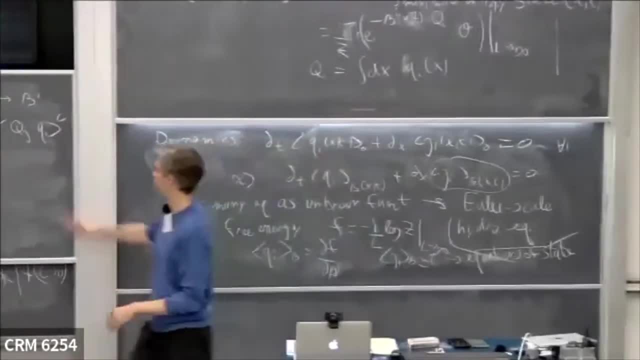 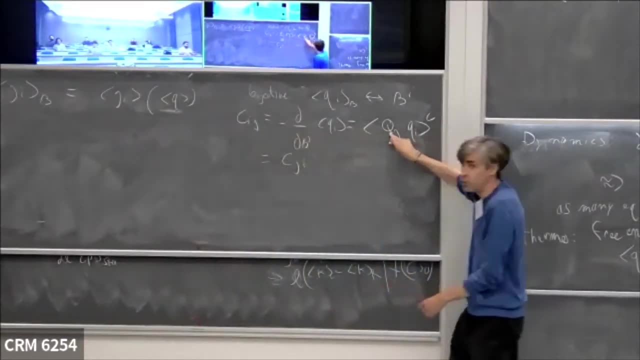 you know, trace minus beta H. So you get the connected correlation function QJQI. okay, So this is a symmetric matrix. By the fact that Q is conserved, I can bring it through. put it there: it becomes symmetric. 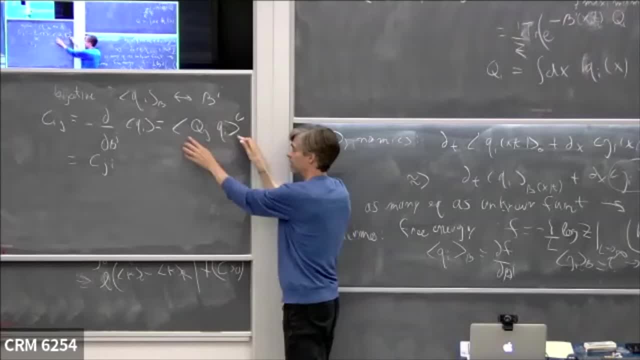 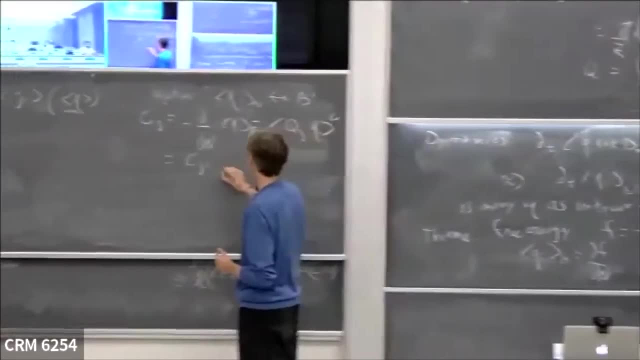 And the X integral. I can put it by the fact that the state is homogeneous. I can put it on the other: the J or the I. This is symmetric matrix And more than that, in fact. this is a positive matrix. 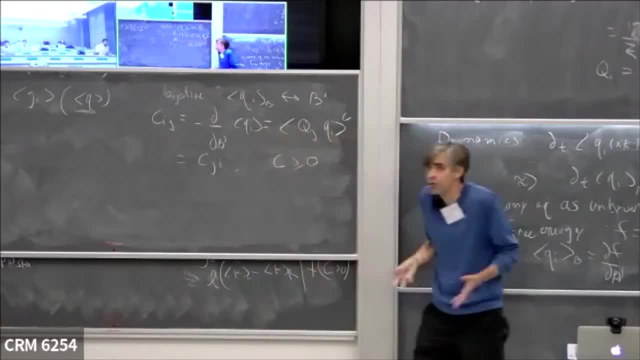 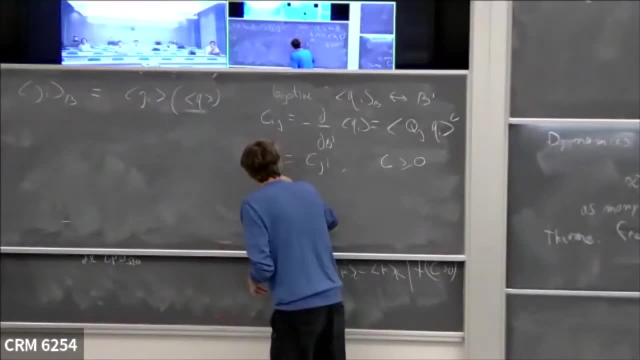 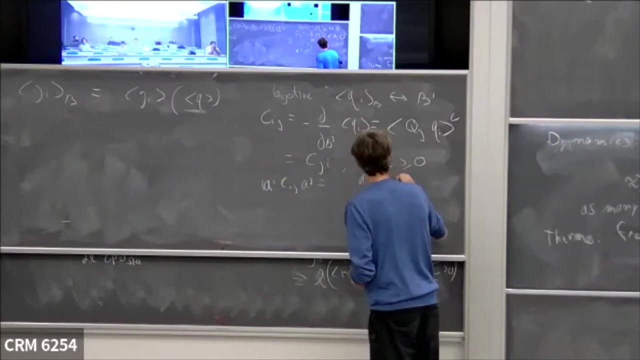 So C as a matrix is non-negative. So because if you do kind of a, so AICIJAJ, what you get is just A I QJ QI AJ, right, A J, no QI QJ, okay AJ. 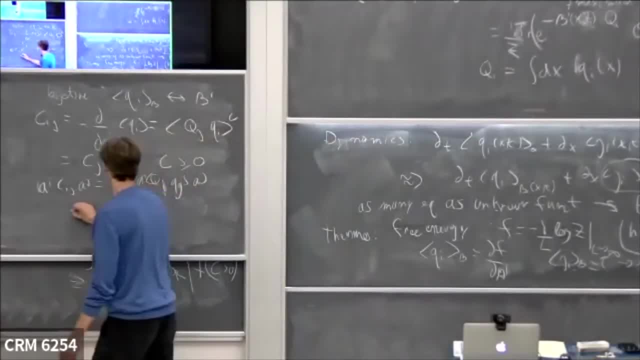 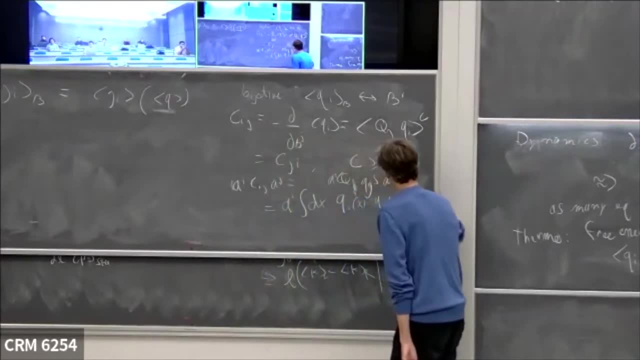 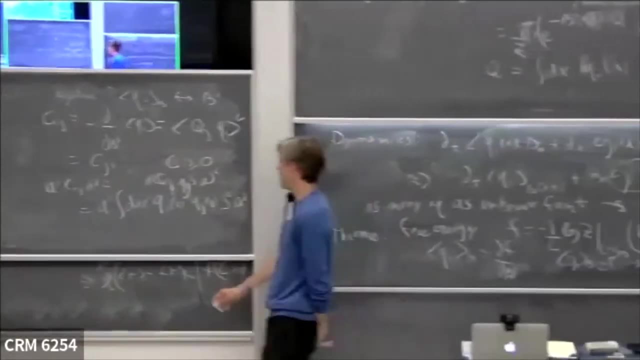 And you know and this. so this is, if I write it specifically, integration the X Q I of X Q J, of zero average, connected A J, okay, sum over Js And I have an integration. 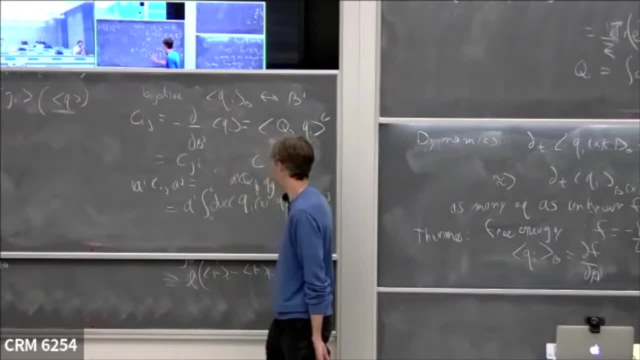 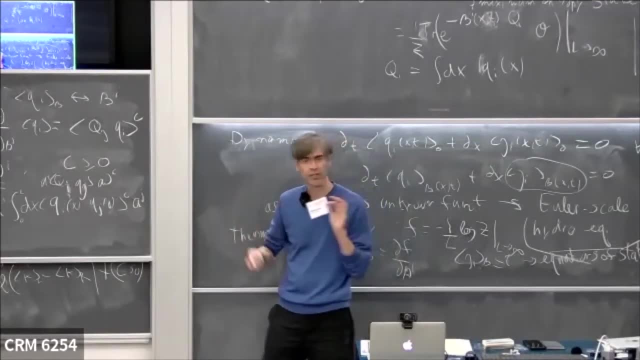 the X here from, say, from zero to L, by using, would you need to? or imagine that the system is periodic, for instance? right, Then you can also integrate over the other variable, like average, over the basic position there. 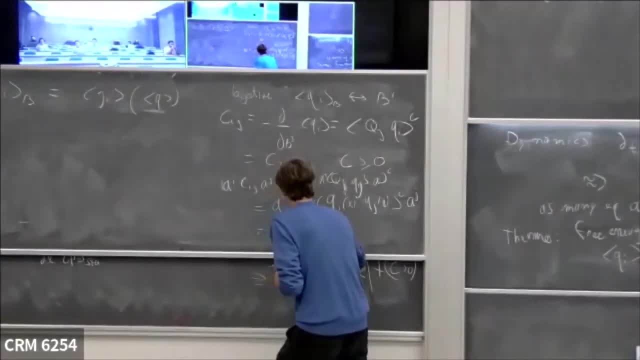 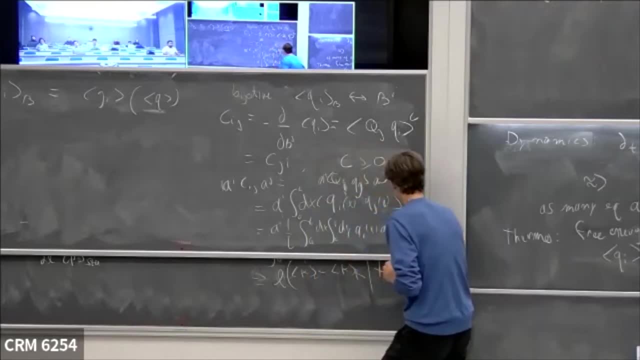 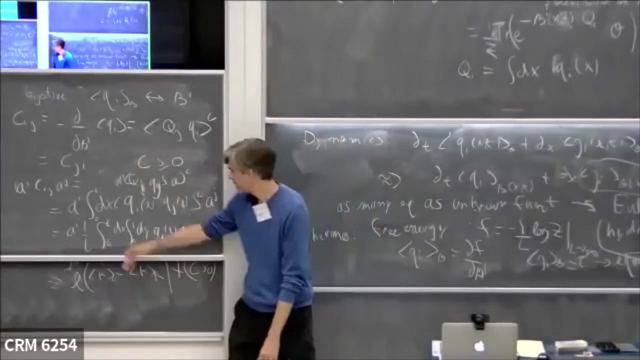 So you can write it as A I, then one over L, and have two integrals, the X and the Y, and have QI of X, QJ of Y, connected AJ. So this is now QI, QJ, so this is average of. 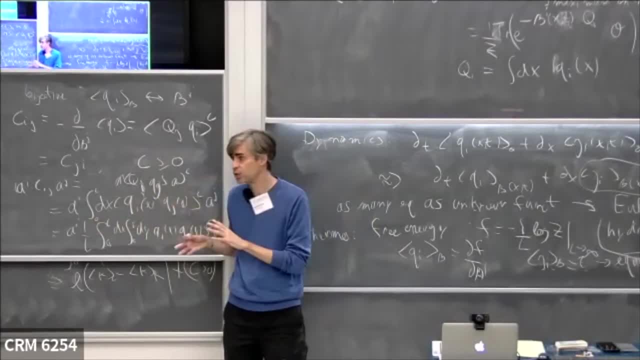 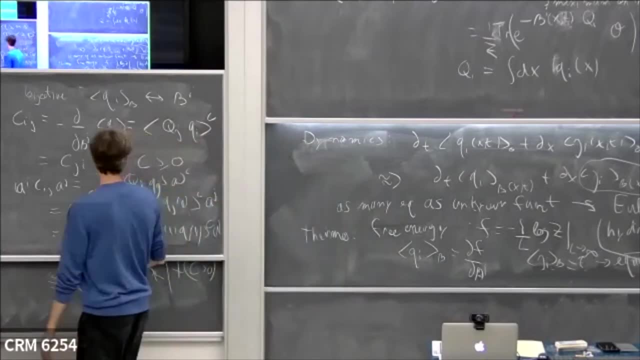 well, the square of an operator, A, I, QI, AJ, QJ, that's positive. If the operator is Hermitian, the square is positive. okay, So this must be non-zero. so, in fact, that matrix is non-negative. I think it's non-negative. 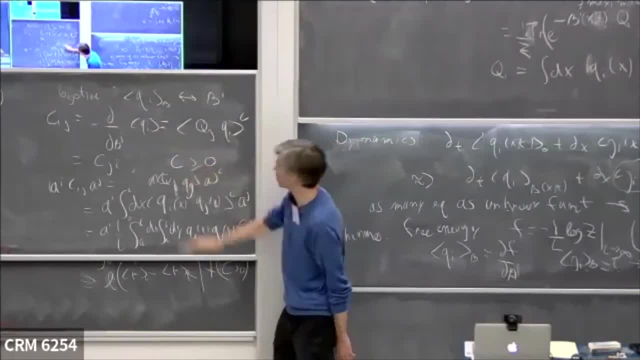 And in fact it must be strictly positive. If it were, if it had some negative bits, some zero bits, some zero eigenvalue, then that would mean that you have chosen a wrong concept. quantity that is zero, that doesn't have any effect. 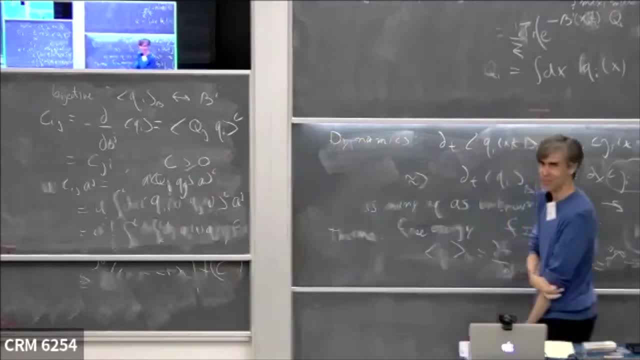 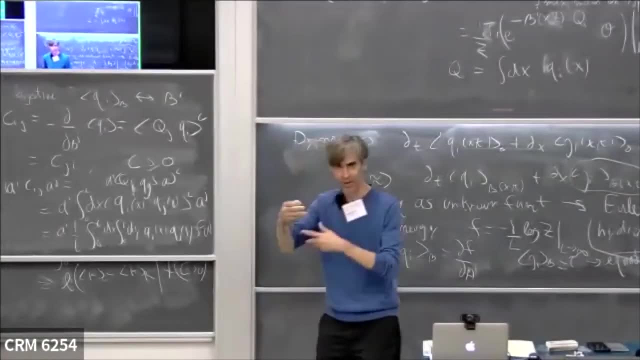 that should just be taken out. That's kind of the idea, okay. So somehow you like a tangent direction in your manifold. that's actually not a tangent direction. it doesn't go anywhere. it doesn't make you move on the manifold. 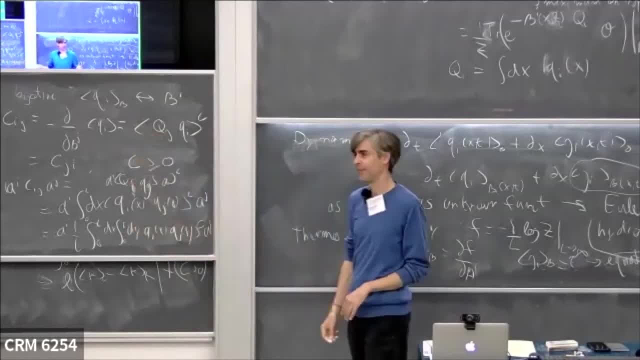 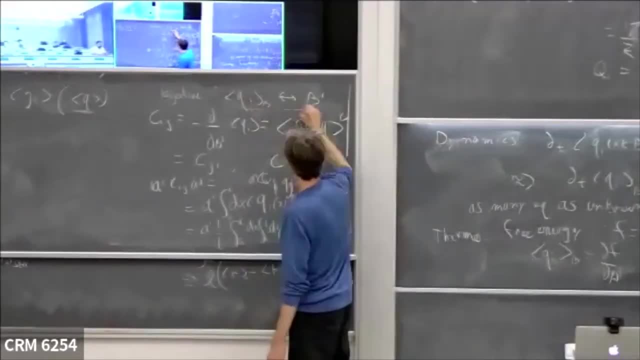 because the dd beta is zero, so no beta derivative, okay, So it must be strictly positive. So this is the C matrix, and because it's positive, then there's, you know, at least locally, but okay, So that's the idea, okay. 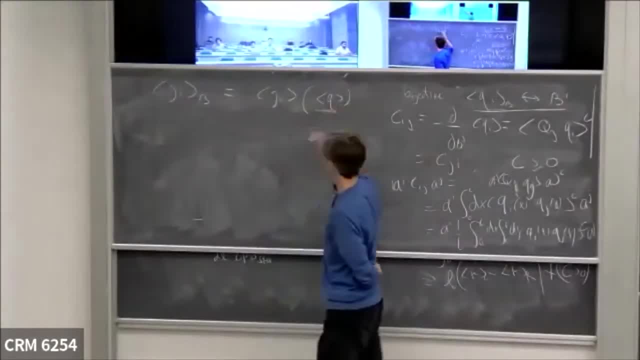 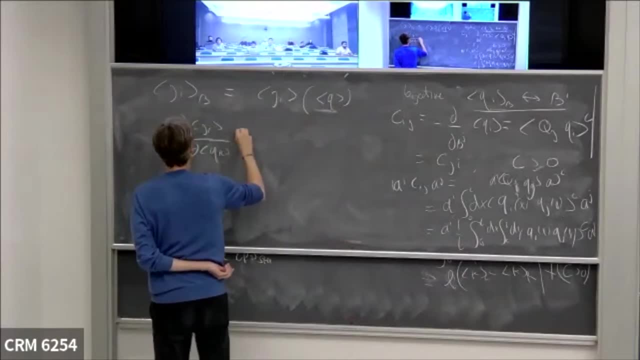 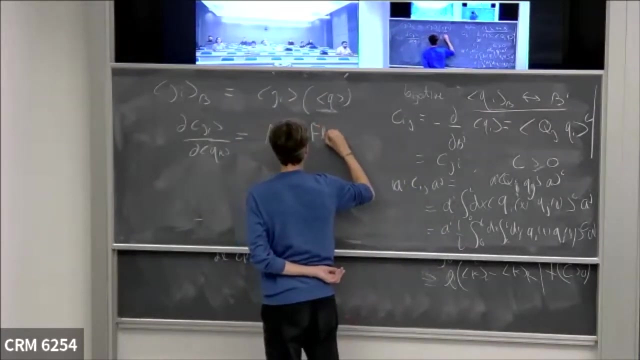 So bijection, so you can think of the currents or any observables as function of q's, and then you can do the dji dqk say okay, By just chain rule, you know, you can write that And this is the so-called flux Jacobian. 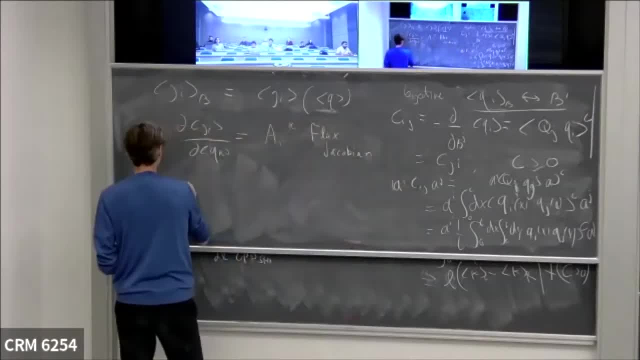 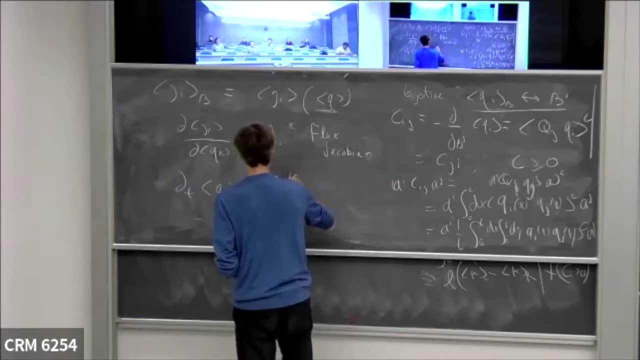 And that is the thing that's important in a lot of the early-calorie dynamics, because then you can rewrite everything like your early-calorie equation, and then you can write everything like your early-calorie equation in terms of this flux Jacobian. 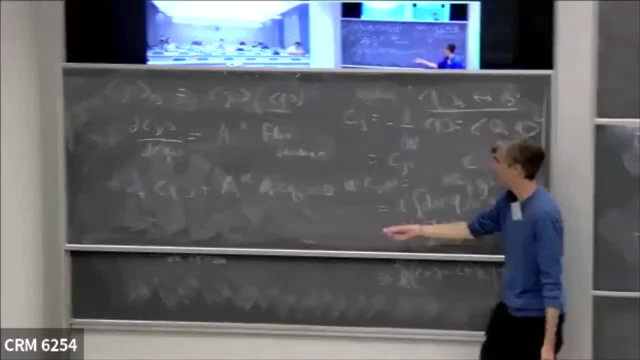 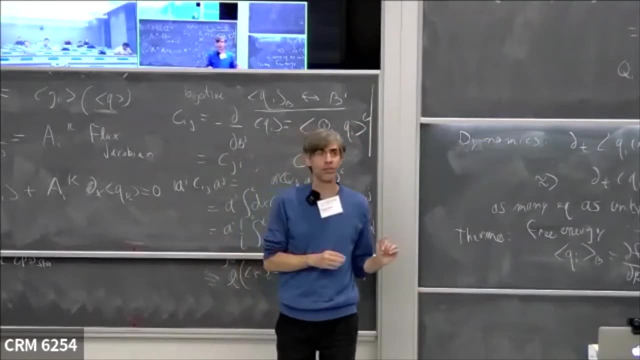 and the conserved density only. So btqi plus aik, dxqk equals zero. okay, So this is the so-called quasi-linear form of the Euler equations. Quasi-linear, it's linear in the derivatives of course, non-linear in general. 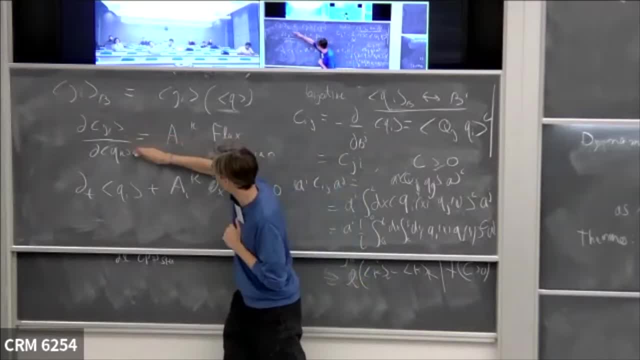 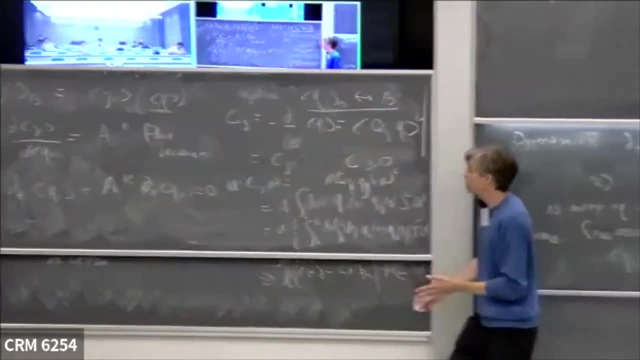 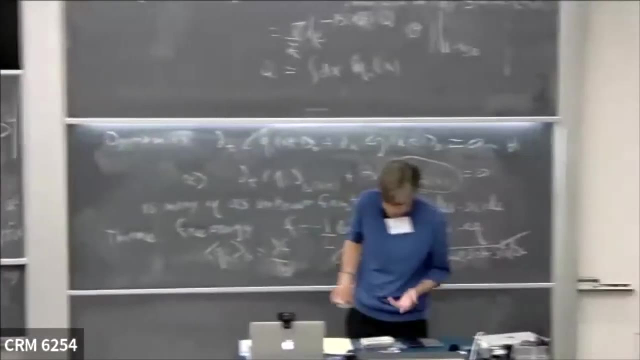 because the flux Jacobian is a function of the state, hence an integral function of the densities. right, It's a function of the densities, and so this is really the early-calorie equation that one should solve and that replaces what we've done in CFT, essentially, 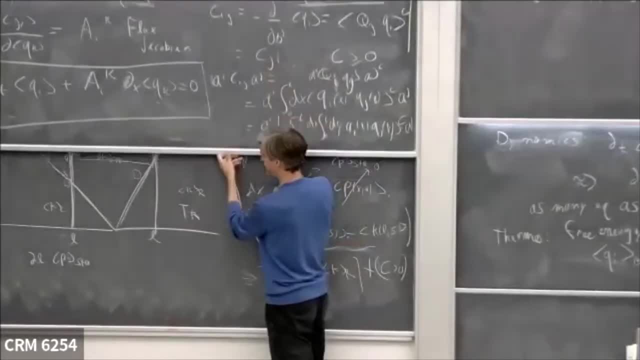 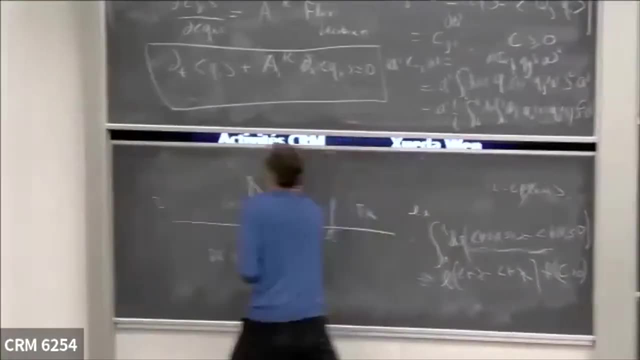 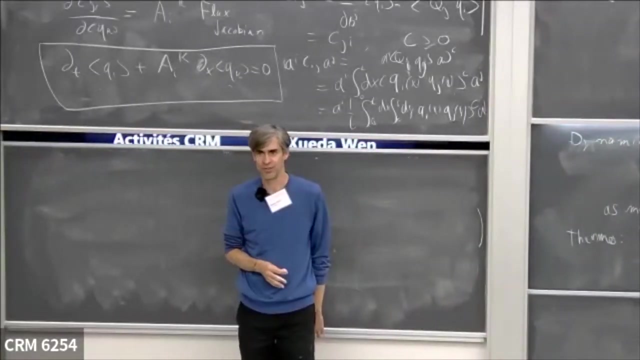 Now. so some general thing we can say about that, and I'm not gonna prove everything, but it's actually not hard to prove a lot of nice things about this. So this flux Jacobian encodes all the functions of all of the physics of the Euler scale. okay, 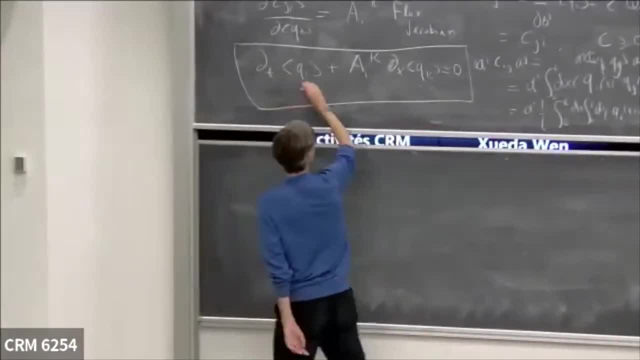 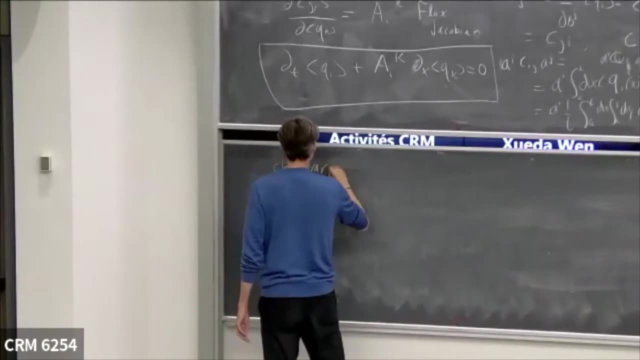 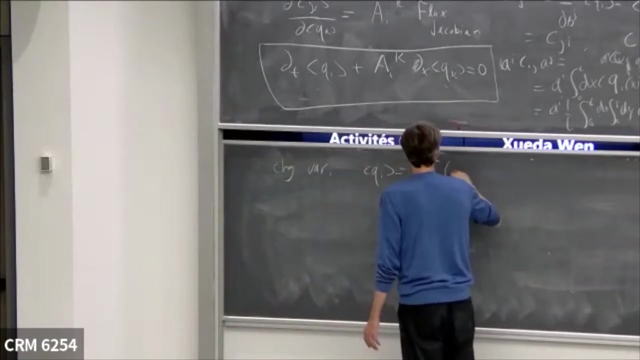 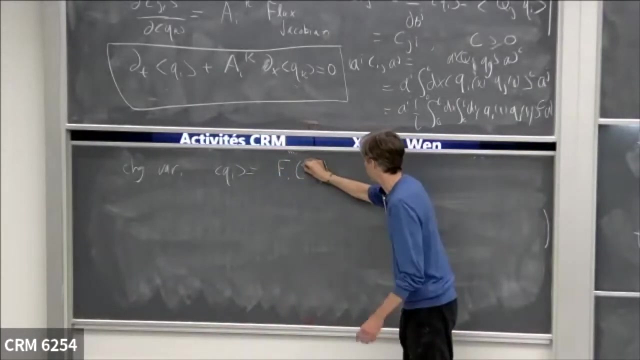 So in particular, you can try to diagonalize this equation. You can change variable, okay. So suppose you find, so you write your qi as some function of some other variable. I call it the n? nj's okay. So all the nj's okay. 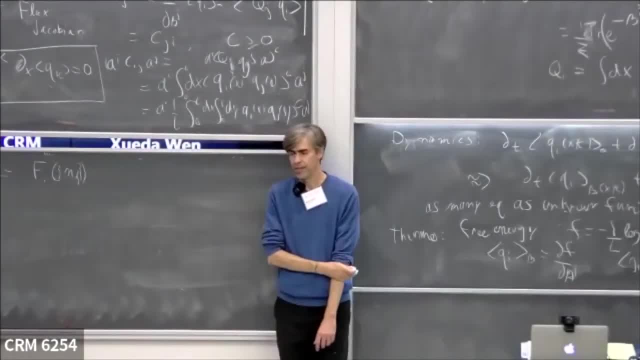 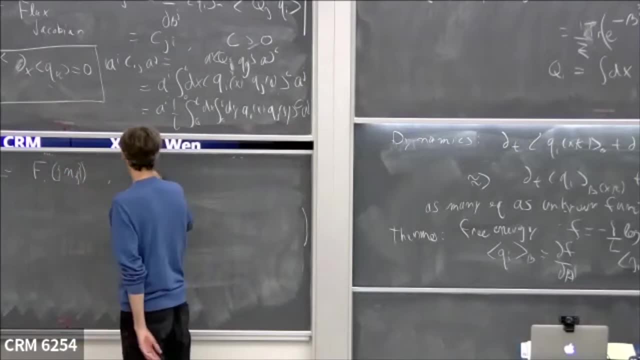 So I change variables. So if qi is some other variable, okay, Well, I can always do that, I can put that in this equation. okay, Now I can take the Jacobian of that transformation. so d, qi, d and j. 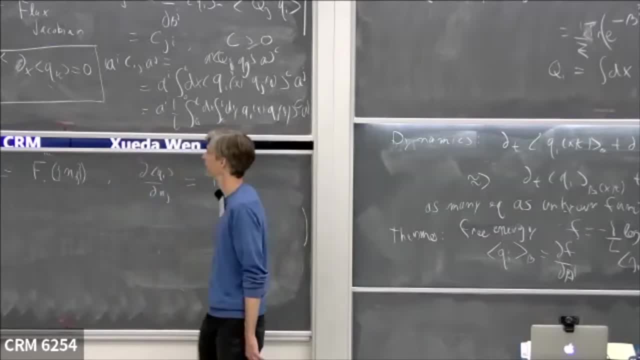 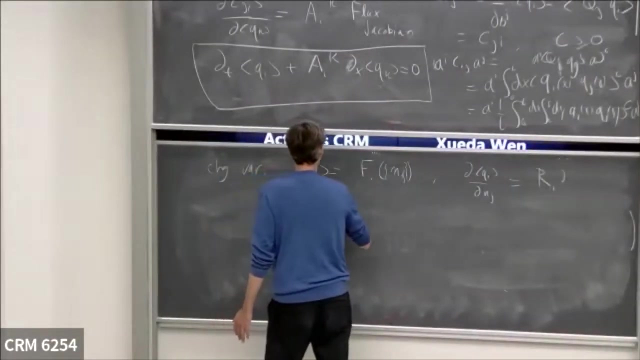 that's some matrix, rij, some matrix. okay, I put that in this equation. What I find is the same structure of equation with a similarity transform of the flux Jacobian. Same structure. that's how I find dt ni plus r, inverse ar ij. 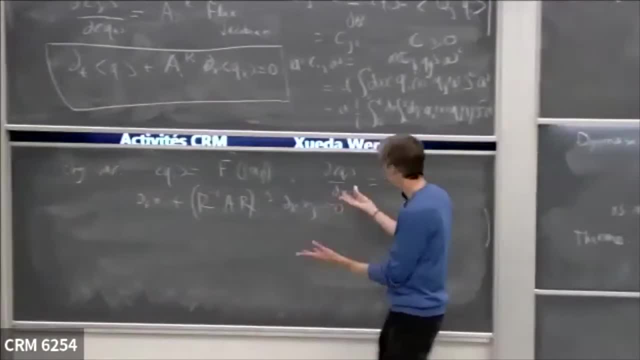 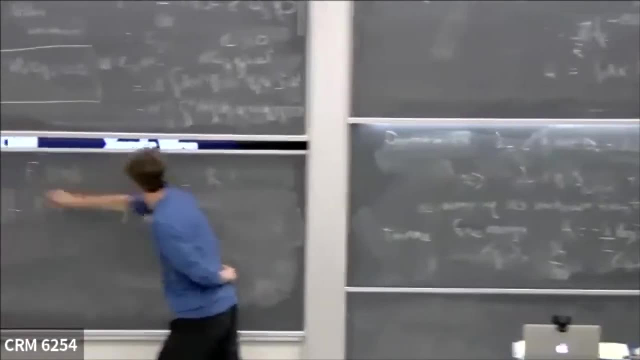 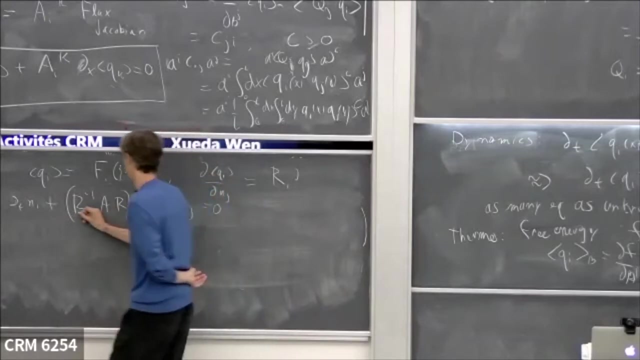 dx, nj equals zero. okay, Same form. So maybe I haven't done very much, but if I can find the f such that that r is the thing that diagonalize a, then I've diagonalized this equation. So if this is some diagonal, 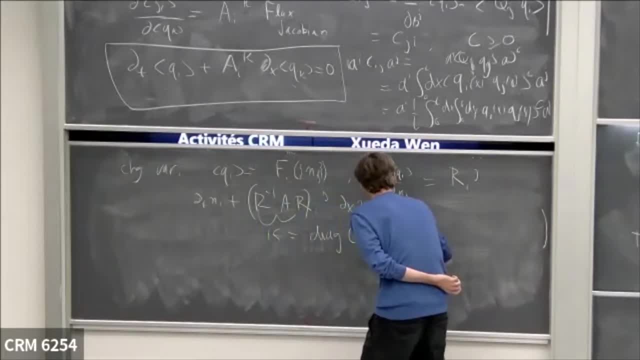 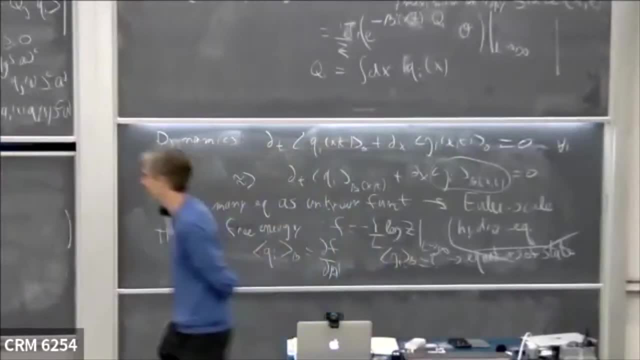 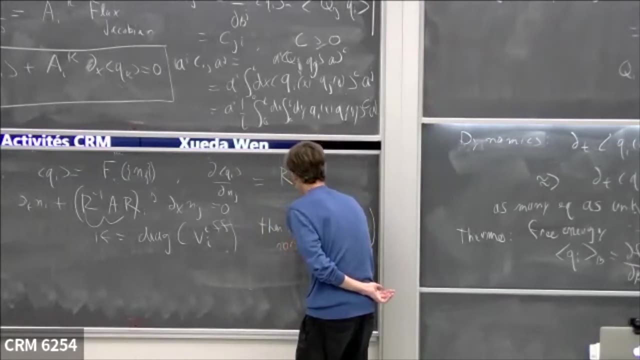 this matrix, say diag of some diagonal element which I call lieffectives, of velocity effective, then these ni's are the so-called normal mode. So they're called the Riemann normal mode. I think So, if you can find. 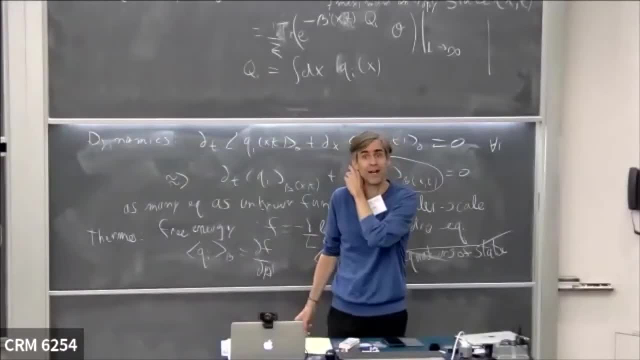 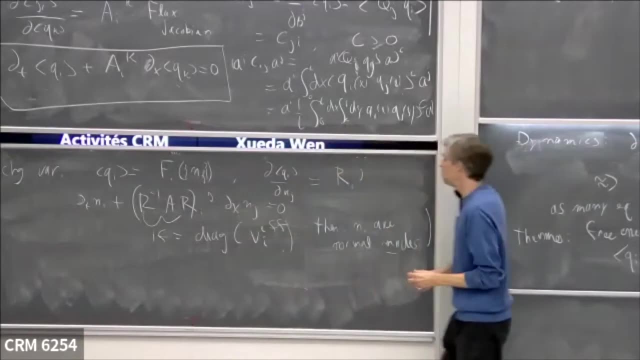 you can. it's not always possible to find these things, but if you can find them, then you have diagonalized. you know your equation of the dynamics. Okay, Now, this is useful. it's nice, Of course. you see, this has a form now. 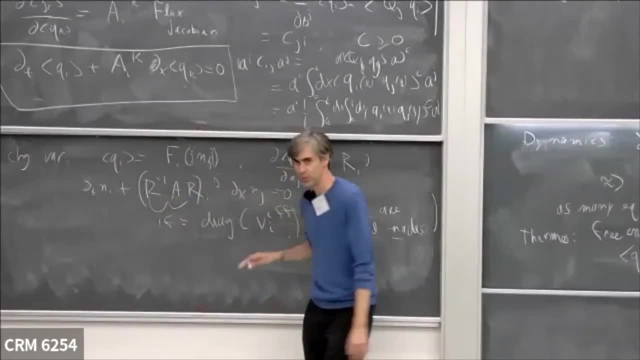 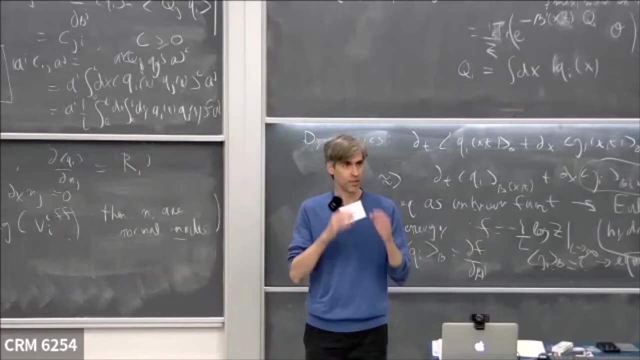 dt n plus vf dx n equals zero, So it has a form of a. it's a bit like the Burgers equation. if you know about Burgers equation has the form of a dt, something plus non-ar dx- same thing, Okay. 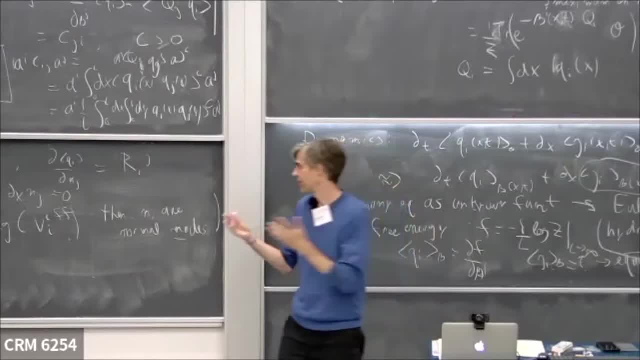 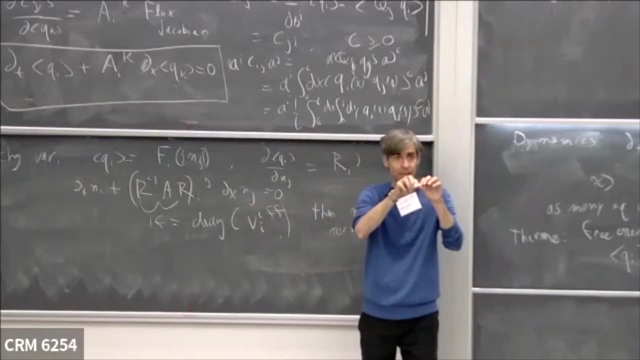 You can solve that by characteristic, As you know. then you can find: essentially, you can just look at this value, okay, And then you can find the essentially. you can just look at this value: velocity follow the velocity and the value of n at one point in spacetime is the value it had. 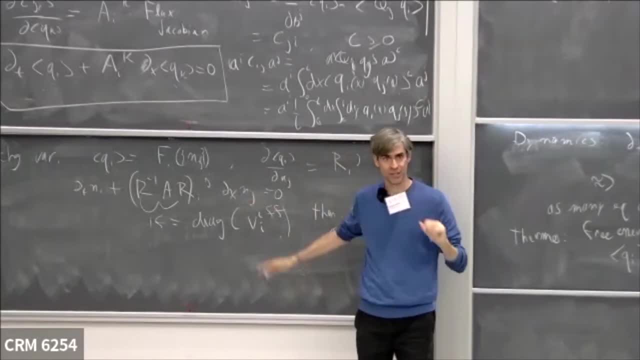 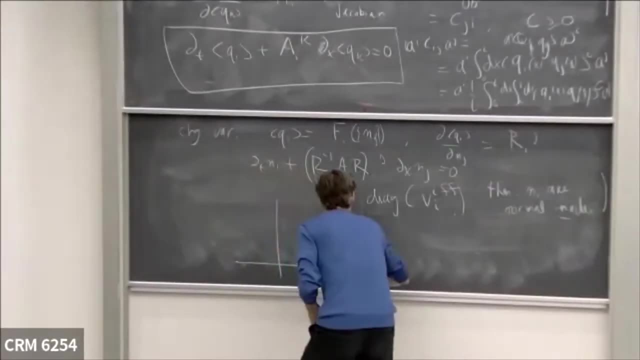 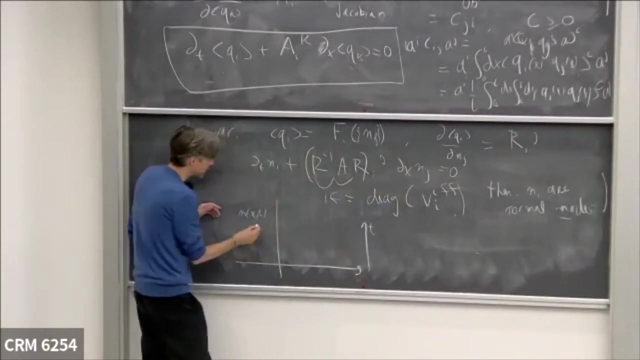 earlier in time, just following the velocities, these effective velocities. so you have this, this form of characteristics in spacetime. so if you have my spacetime now, time going up this time, okay, so i have some n value there at xt. i want to know what it is. i just have to follow, i don't know. 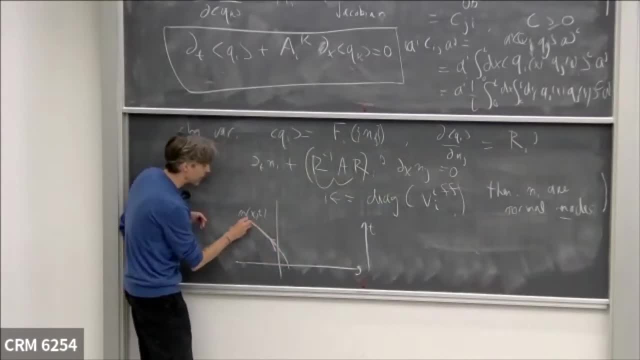 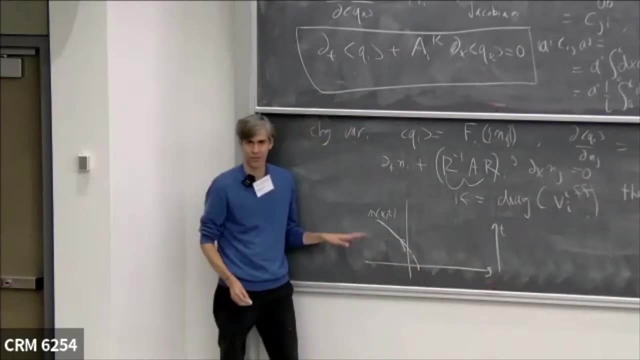 kind of the, the whatever line that is parallel to the local effective velocities everywhere and look at the value that's there and it's that value that it takes. so if you know the initial values, you can know that. of course you know you have to to find what these velocities are and 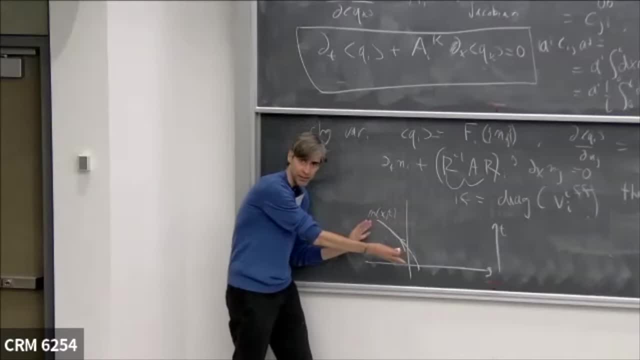 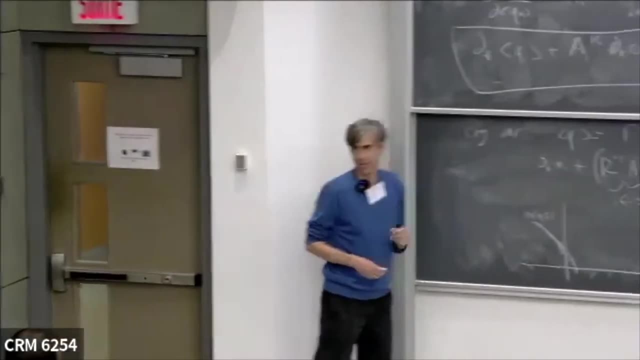 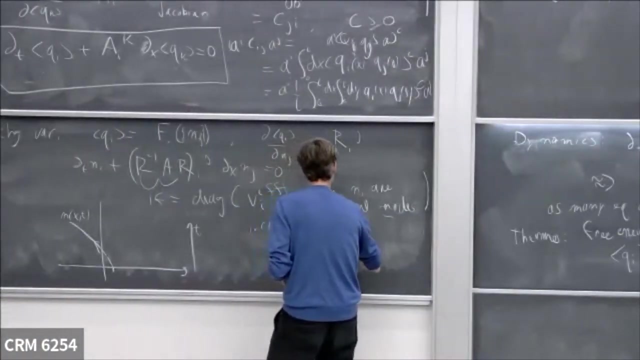 they depend on n non-previally. so it's kind of a non-trivial system still, but still it kind of it has a nice structure right. so this social characteristic that comes out from this diagonal equation right in cft. cft is so simple: a is zero one one, zero constant. you can do linear transformation to diagonalize it. 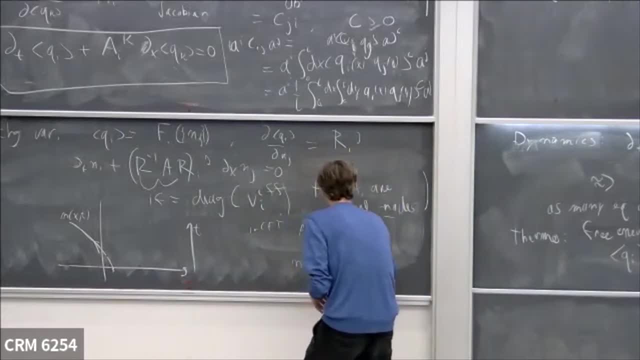 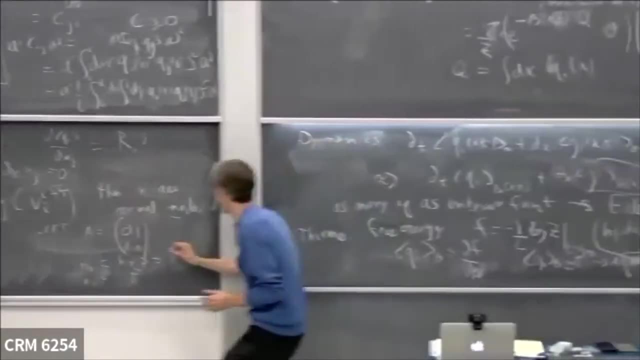 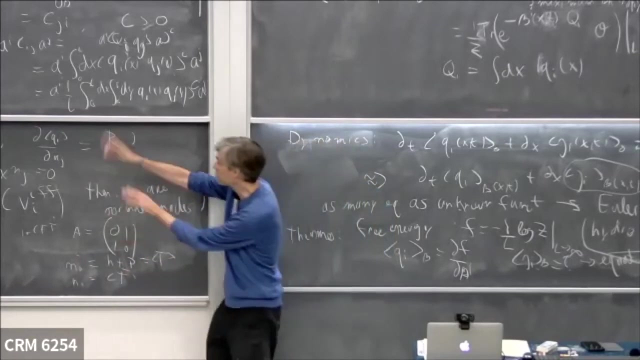 so n? zero is a h plus p is just what i was trying. t and n one say is a t bar. t and t bar are the normal mode where the average of these things- okay, these are the normal modes, t and t bar are normal modes of the cft hydro and everything follows and these characteristics are: 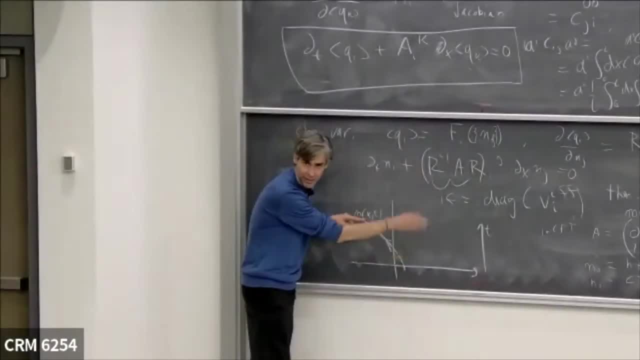 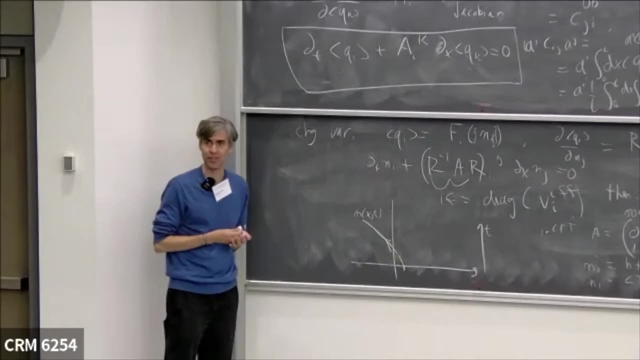 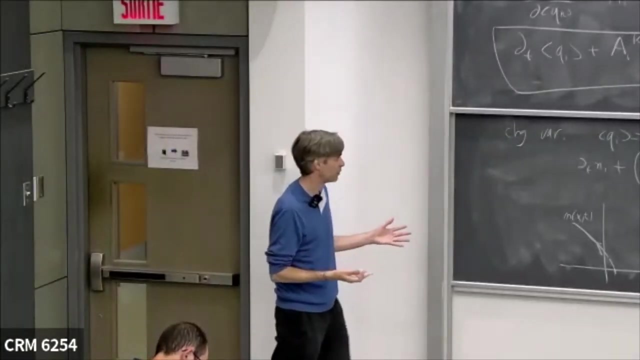 just a straight line going back to the initial state that i was showing at the beginning. for for the solution to the session mistake, just a generalization of this cft picture. it's more complicated, but see the same ideas. okay, but non-linear, because now the flood, jacobian in. 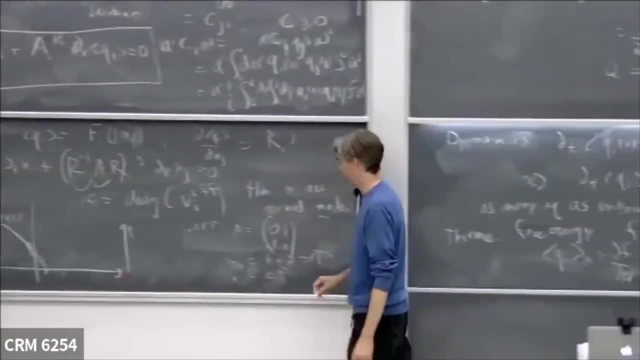 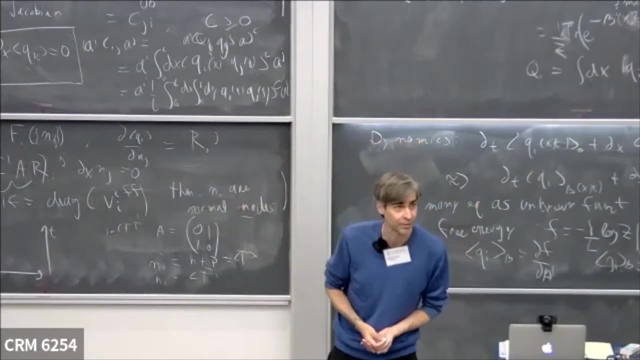 general depends on the state and, by the way, so the the the definition of a free system. you may want to. so what is a free system in general? what does it mean free, if you current people know that the definition, in my opinion, is a system where the flux jacobian is constant and it's free and 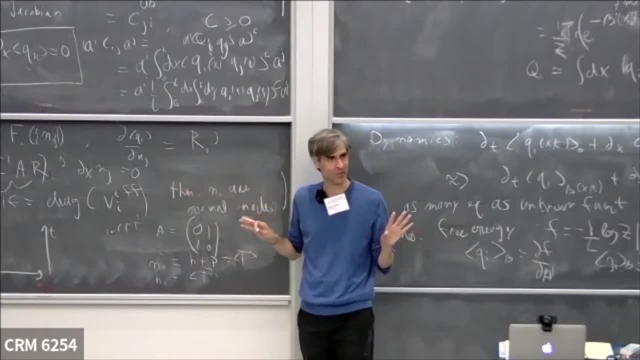 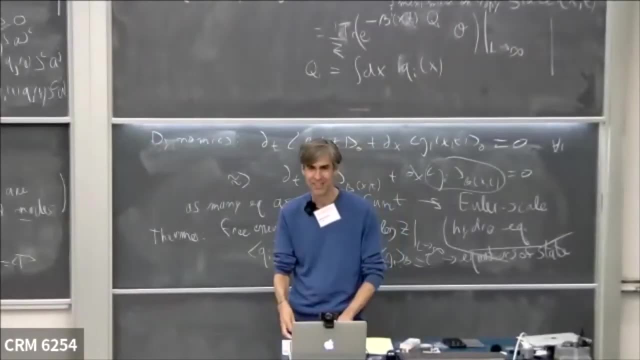 then you can solve everything. it's free for the particular hydrodynamics, for sure. if it's not constant, not free. so cft is free at the in the viral sector. from that perspective, okay, any questions about this? yes, yes, yes, indeed, indeed. so this is, you see, the question of particles. 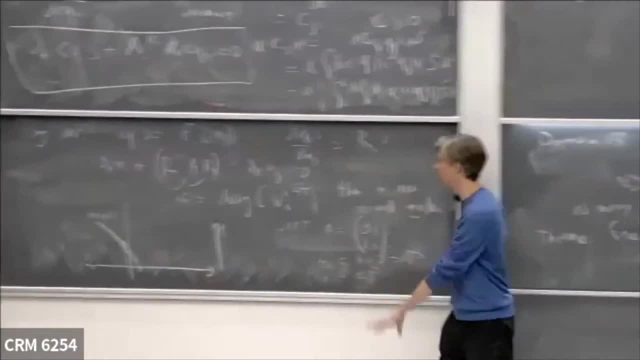 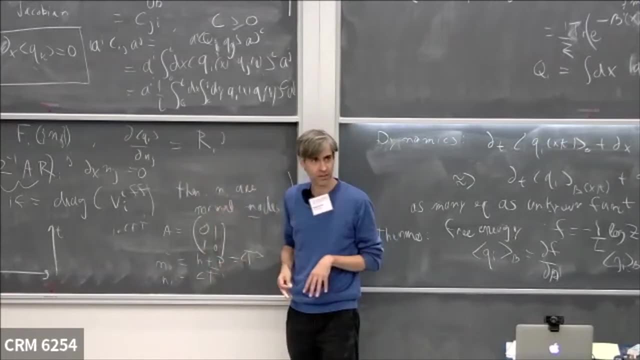 because the particles are very interesting. so once you do the hydro, the quasi particles, what they're are is the normal modes. so these are the particles of your earlier scale in cft. these are the basic particles of safety. you know kind of this asymptotic particle that you can define in these. 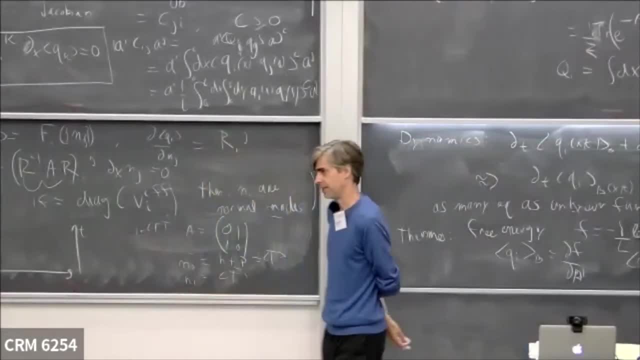 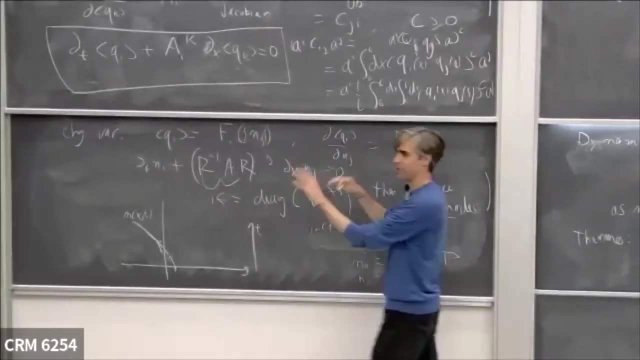 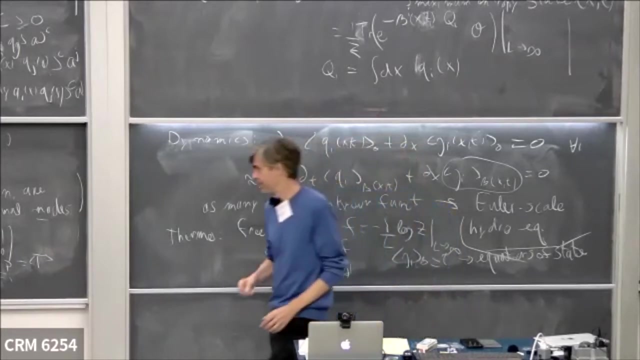 these, uh, masses theory. you can define them okay. so now you have something general and now the. the point is you have to find what are these modes and what are the, what is the flow, jacobian, and how this whole thing works for give an example, you know, sorry, ah, yeah, yes, yeah, so so 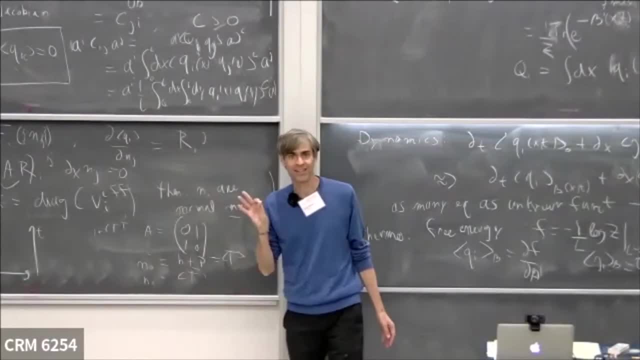 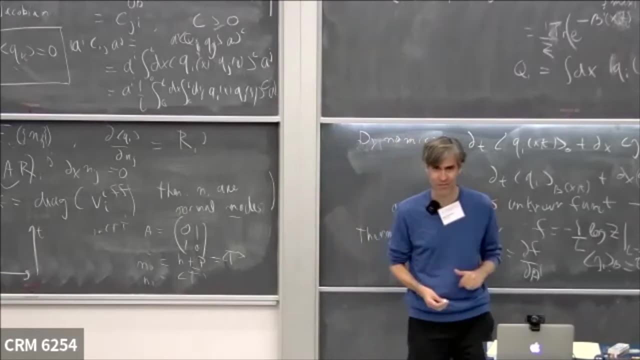 okay, i can do that with free theories out of that. and what you think of a particle in the free theory? what is the normal, normal modes? so it kind of all works out very nicely. maybe i give- i mean, let me give the example- the free theory. i think i could give the higher d. 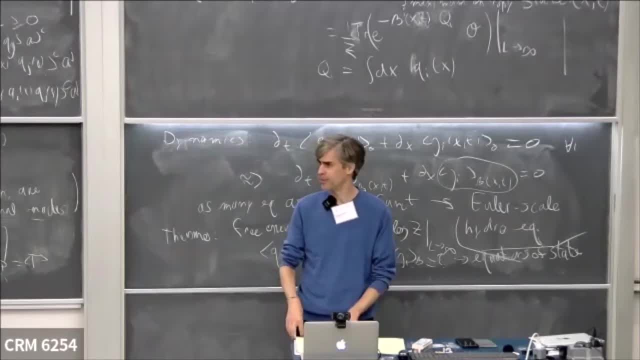 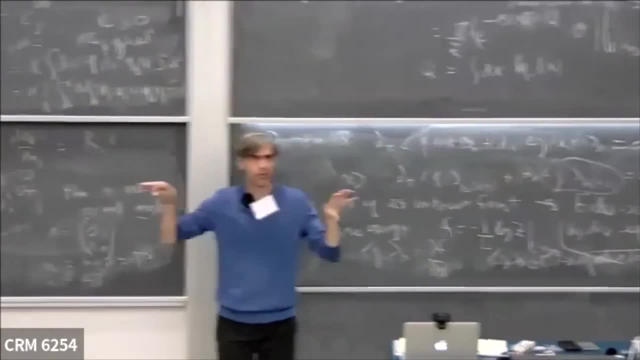 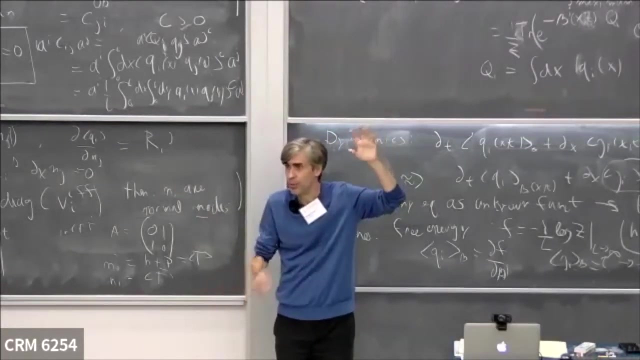 uh, the higher dcft example, but it's a bit technical so so for higher dcft you can. you can kind of restrict that to one plus one d by just looking at currents going in one direction. of course the stress sensor in higher d is traceless in higher d. so the bit of the stress 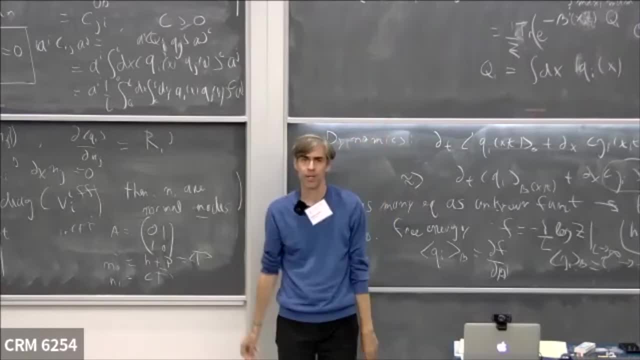 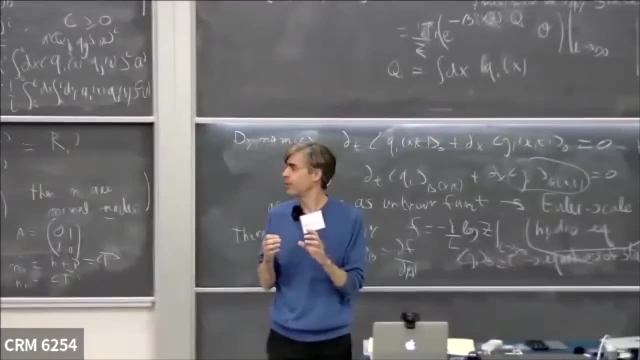 sensor, just in the one plus one. d is not traceless, it's something else. so you have a non-trivial uh pressure, but it's not so complicated. in the end the pressure is still uh proportional to the energy, but with a different, with a constant that depends on dimension, like pressure is d times z or 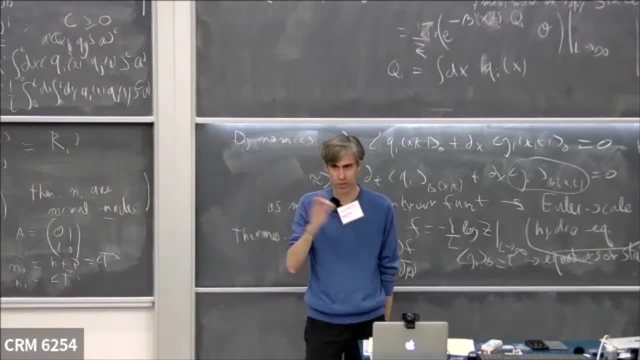 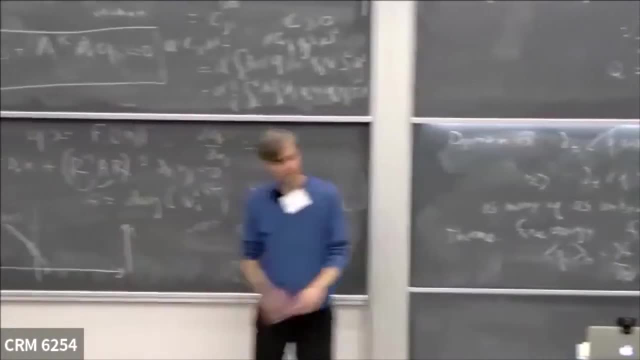 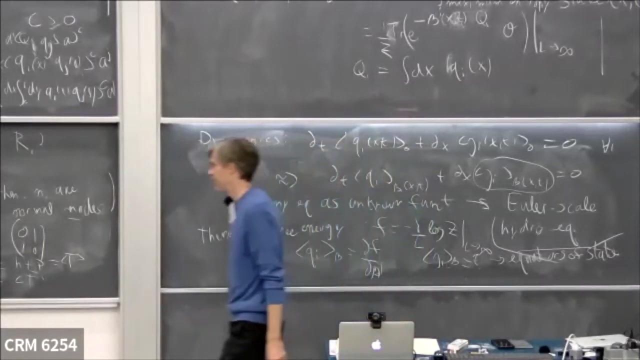 something like that. it's just a small change, a small change of the equation of state, okay, and you put all that in it and then you can. you can solve that. you have a flux, jacobian, that's a bit more complicated, that depends on the state, and then you can do the whole thing, okay, so the one thing he was talking about, uh, kind of um, kind. 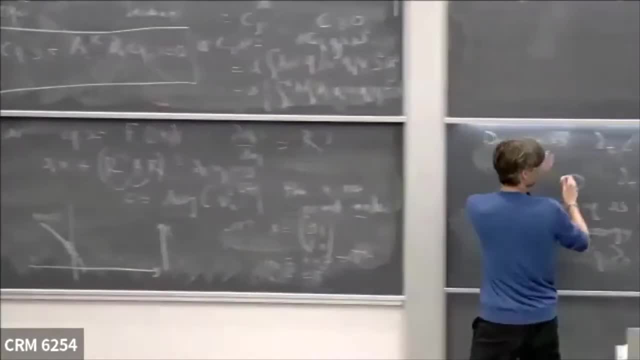 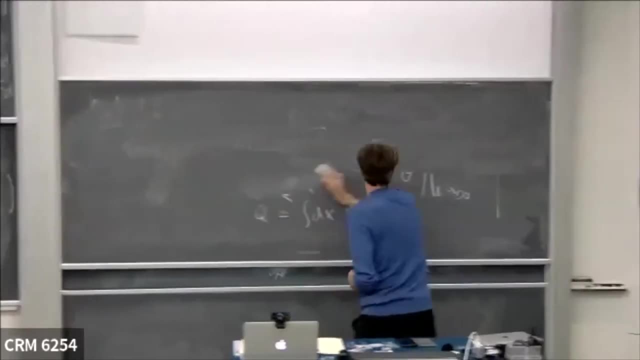 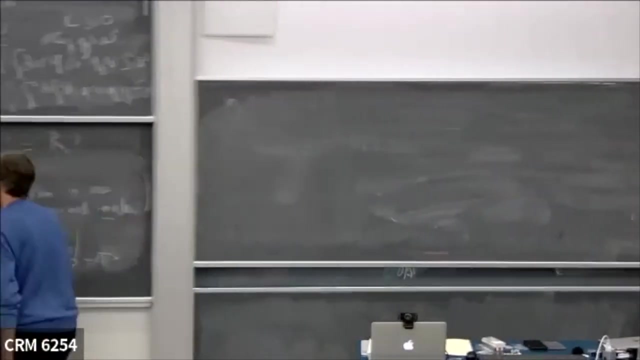 of uh, the light cone and all that. so if i want to solve uh, if i want, if i want to solve the, the problem of uh kind of left right and all that. so so if, if i have this, i have this problem, okay, i have this thing there. so i have t left and t right style there. now this initial 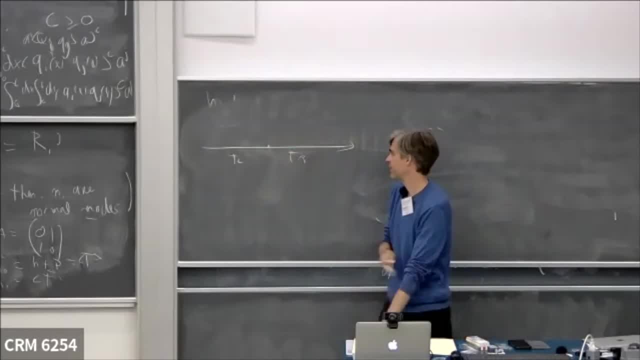 state is actually scale invariant because it's it's the same everywhere, all x. there's a zero where it changes the same way because it's the same as the initial state. that x and that lambda x is the same, so it's scaling invariant initial state. it's actually it's not cft, but it's a. 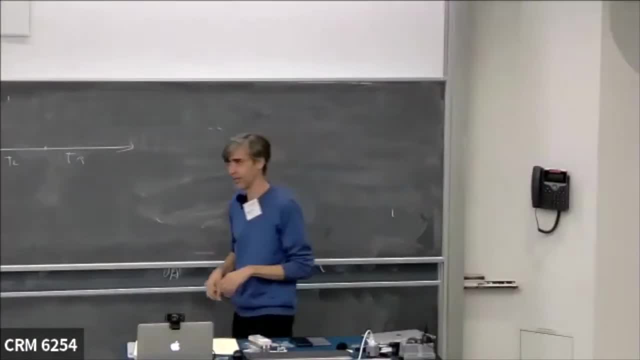 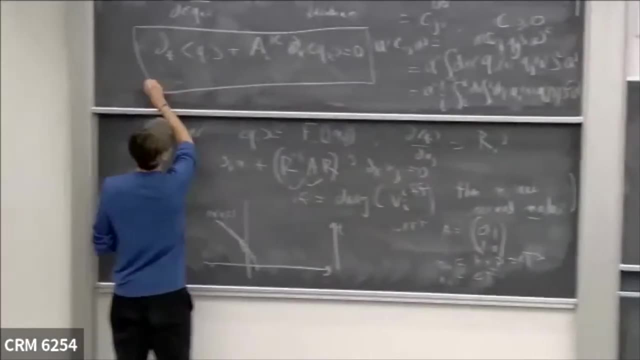 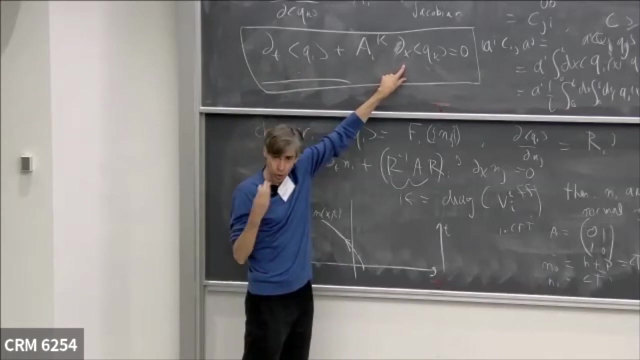 scaling variant at the level of local averages, right for our local averages. so as i evolve, then our equation itself as well as say: like that form is also scale invariant in space time. now this is dt there and dx there, same power. okay, so earlier, how do that makes a scale invariant. it's not cft. 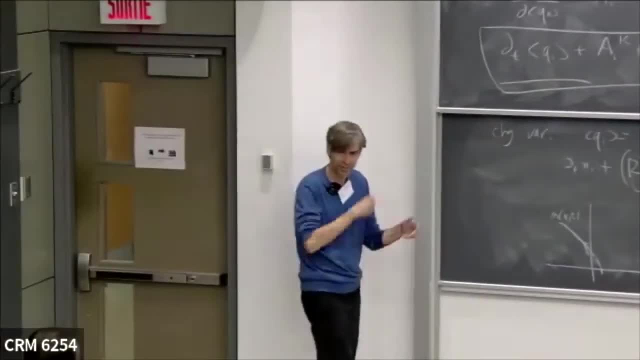 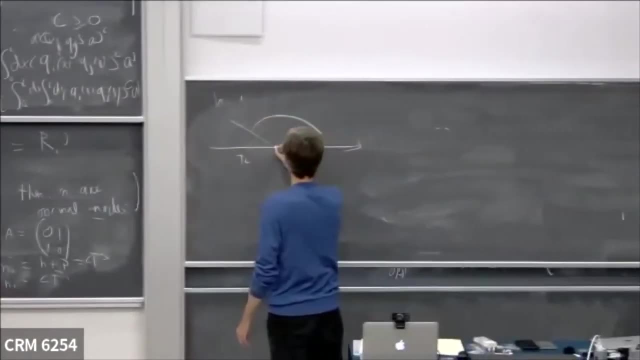 but it's scaling variant right, at least with scale transformation. it doesn't have the structure of cft- now that- but still it has that invariance. so initial condition is scale variance and final condition. so that means that the whole solution is going to be ray dependent, only here invariant. 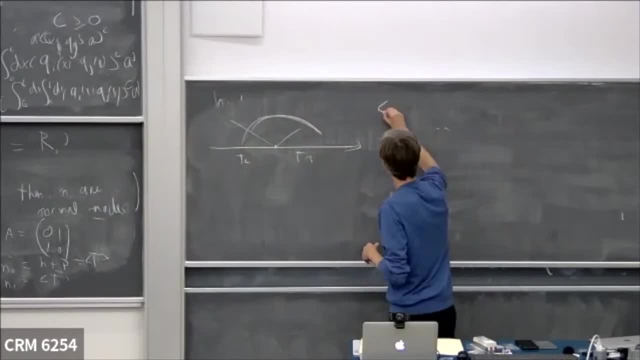 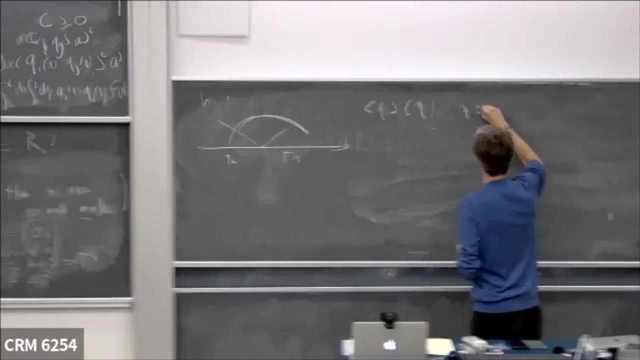 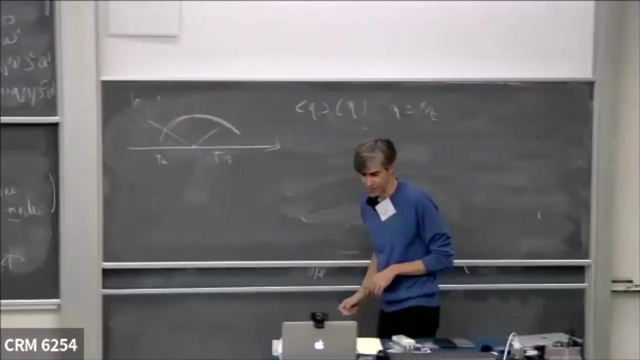 respect to zero. okay, so all the averages of all conserved densities in space time? they will depend just on some rays, or eta is x over t. so which way you look at, okay, when you put that in this equation, what you get is a very simple equation. if you find, find the normal modes and all that, just get it, get it. 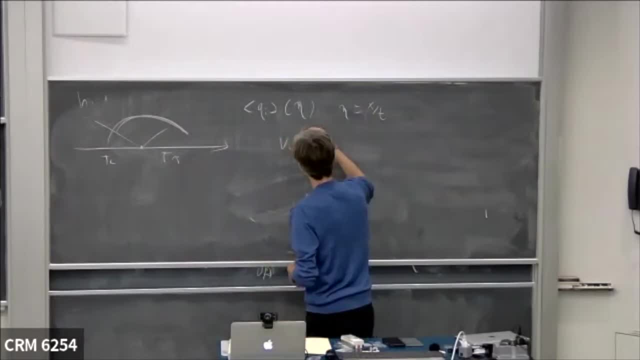 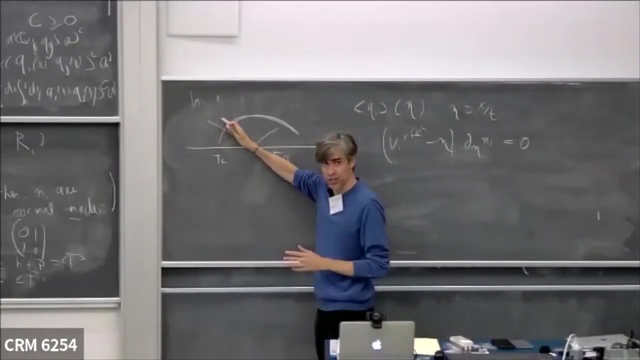 right. what you find is that v i effective minus eta times v eta of n i was equal to zero. for i to find this is an algorithm. so what you find is some kind of eigenvalue equation and you find that this n- either it doesn't change or the ray at which you look at is equal to one of these. 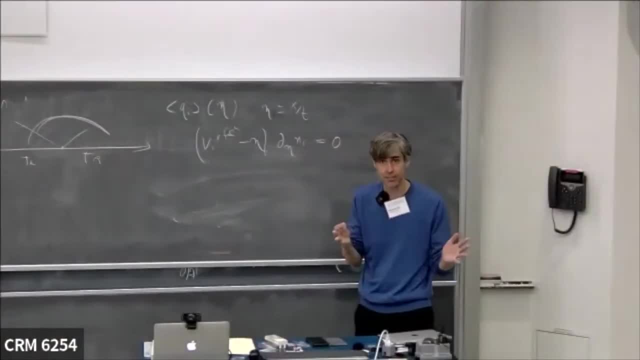 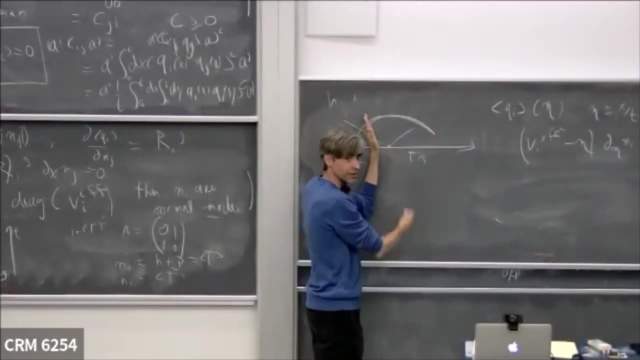 effective velocity at that state. and this is, this is the situation in generic uh system. so you, typically what you're going to have is going to have no change in the shock somewhere in some velocity, or maybe a discontinuity at some- no, that British- and then what you're going to have is going to have no change in the shock, somewhere in some velocity, or cidade, or maybe uh discontinuity at some- no, death vs- and then no change in the отдельän. so to complete, and then between the two���ہ we have to 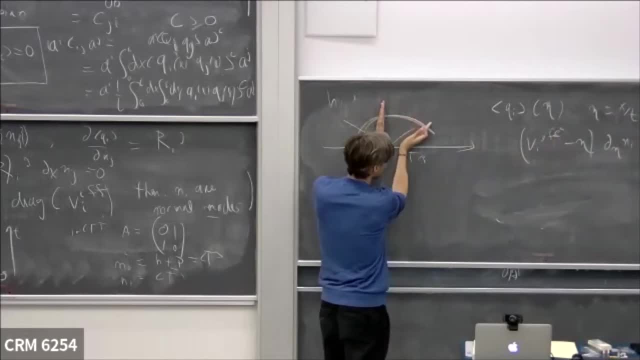 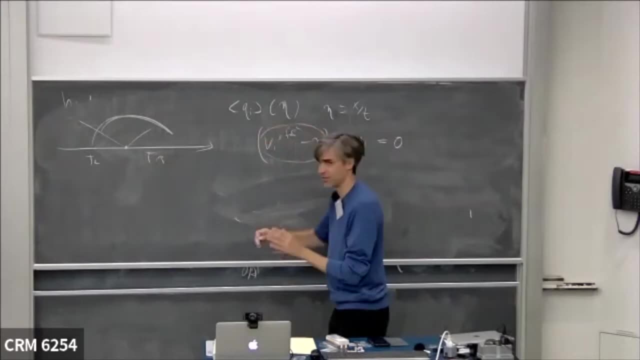 and then you may have what they call a rarefaction fan where somehow you manage to change your end just in the right way so that this relation stays valid, kind of everywhere, for a whole fan of eta. As you change eta, the Vf changes as well and you kind of manage to make that correct. So looking at 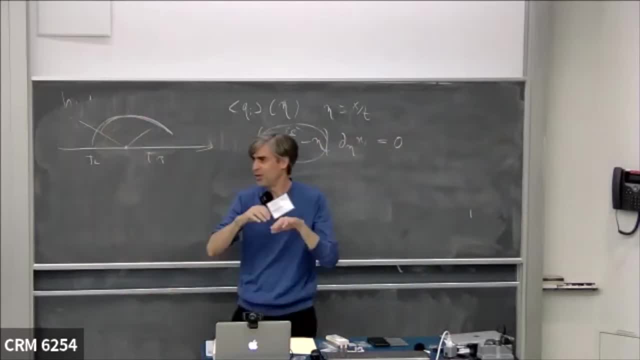 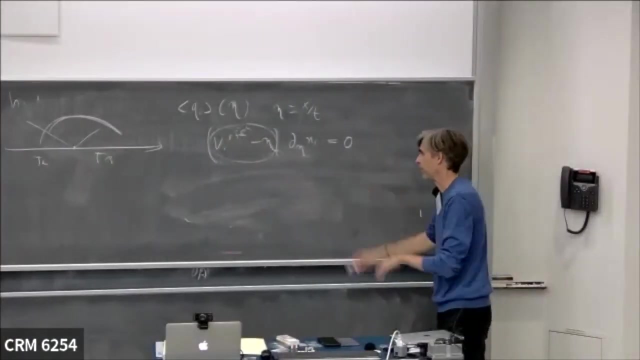 that equation, then you get a non-trivial structure in spacetime of where it changes, where it doesn't change, and that depends on this flux, jacquard, which is the spectrum of the A matrix, of this Vf, which is the spectrum of the A matrix, and you know the various structures of this hydrodynamics. 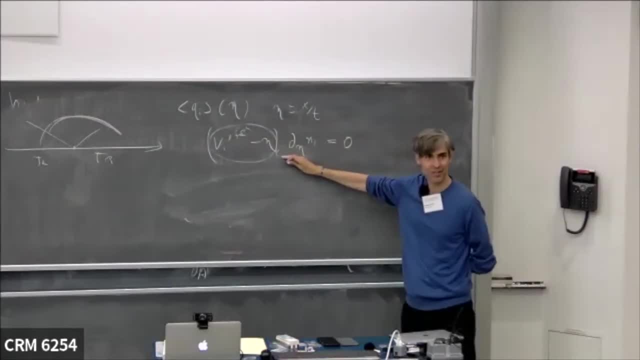 So anyway, I don't want to. there's a whole theory of that equation. it's very beautiful hyperbolic equations and the solution for the Riemann problem and that problem there for this equation is the Riemann problem of hydrodynamics- books written about that. 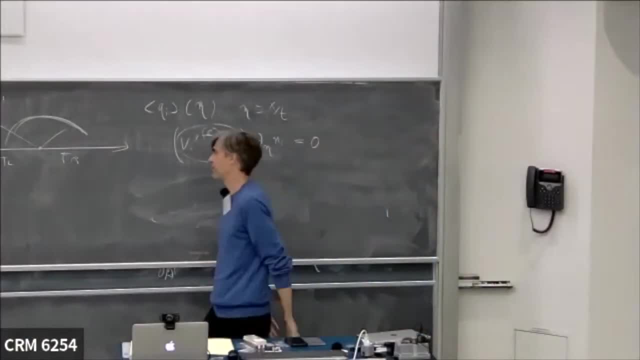 In Pascal you can have shocks and all that, but I don't want to go into this details of that in Pascal. So in higher DCFT, that's what you have to do. you have to look at shocks, rarefaction fans and how the theory of the hyperbolic equation. 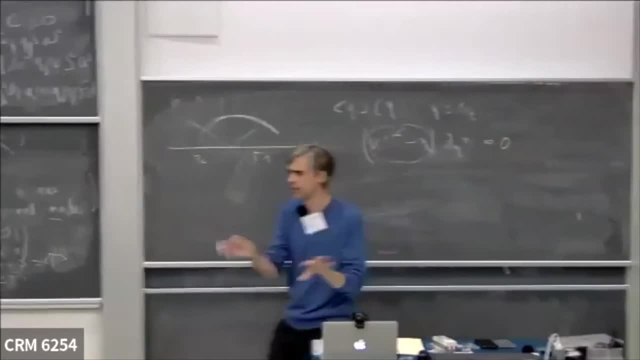 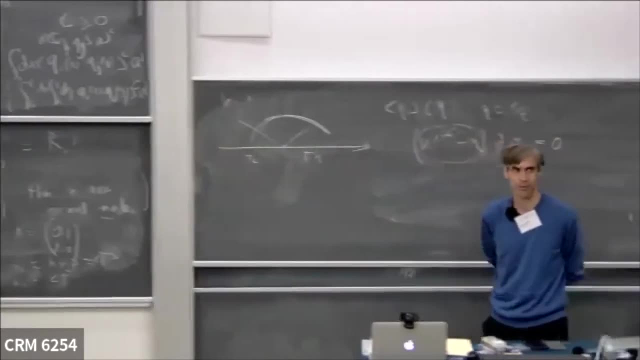 You go in the books and in our papers. originally we hadn't gone in the books and we have found a solution. it was incorrect. If you go in the books you realize, oh no, that's not quite the correct solution, then you have to do this and that which we did eventually. 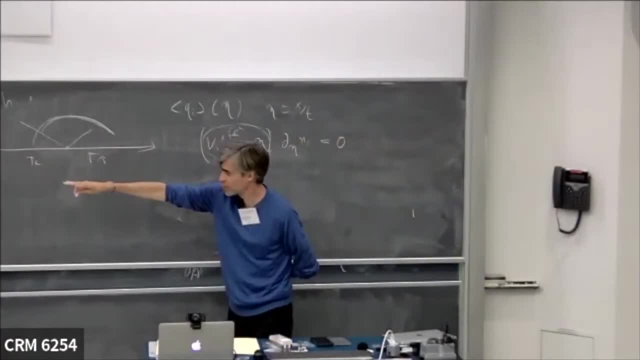 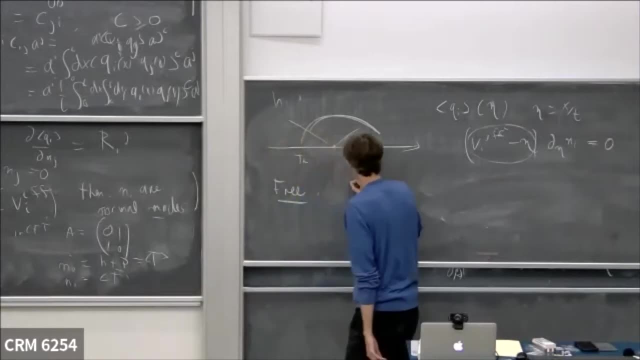 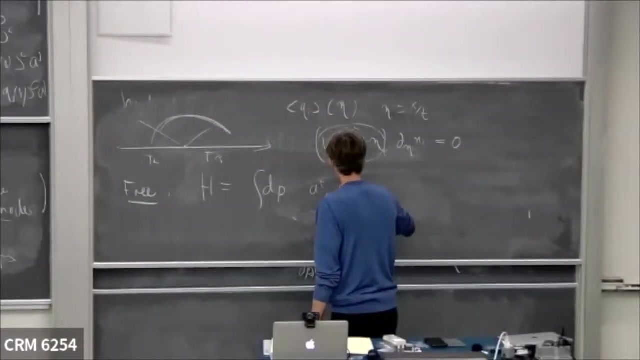 Now, but for free models you can also do the same thing. so you know, then you can write equation and all that. But how do you do for free model, free particles, model. Well, suppose my Hamiltonian has that structure. Now I'm gonna become maybe a bit less precise, but okay, I have these creation. 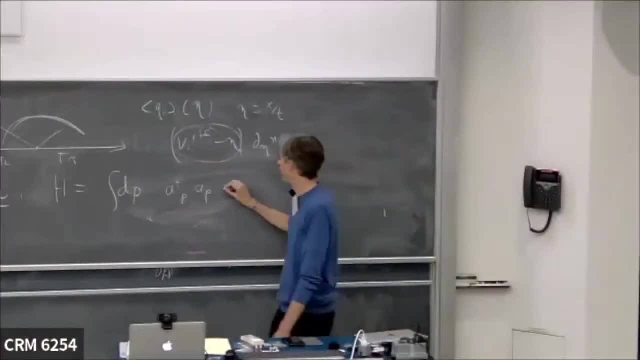 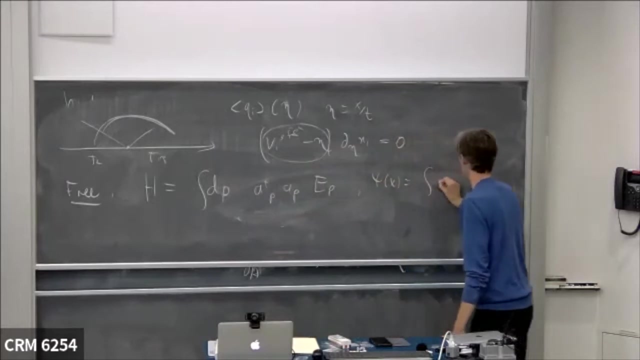 and relation operator, a dagger p at Hamiltonian, have this form times: some energy ep, some dispersion relation. okay, And even my fermions. they look like that cx is supposed to integration ep to the ipx. ap will be one of the square root of two pi to have the right normalization. 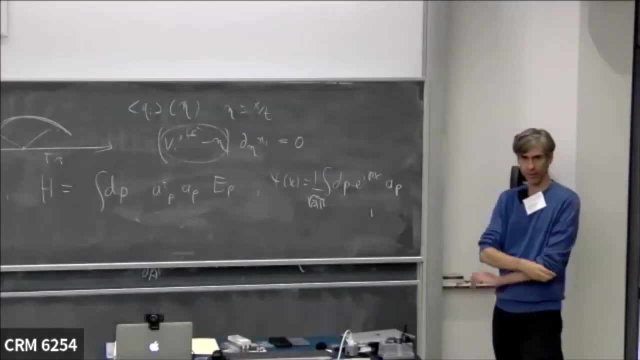 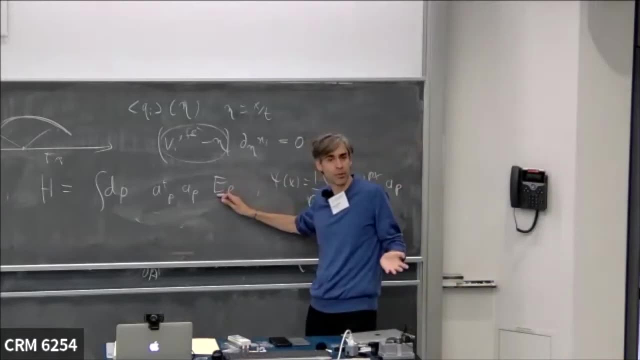 and then everything is normalized in the usual fashion and all that. okay. So I construct this free fermion model for some dispersion relation. p square is going to be a galleon model. If I wanted to be relativistic, actually I would have to do the Dirac matrices and all that. but I don't want to do Dirac matrices. 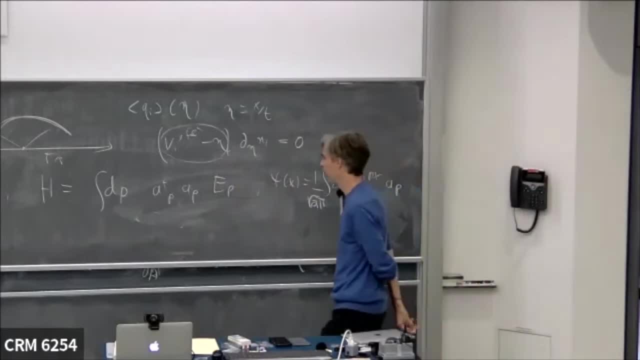 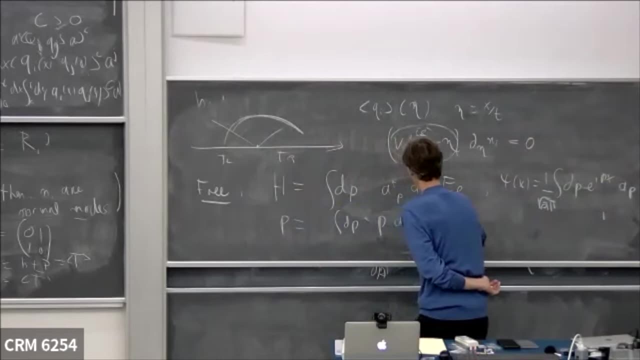 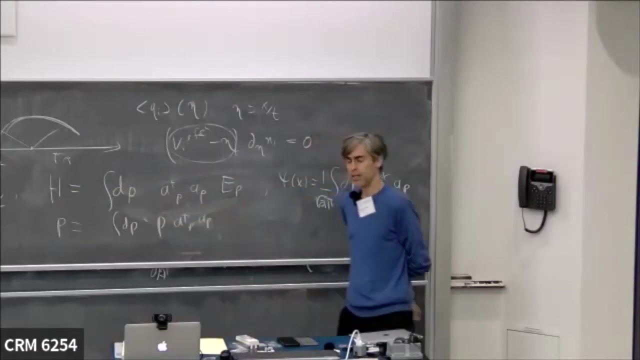 Okay, so this is a nice little pre-fermen models and of course this is a constant quantity. the momentum is also a concept quantity, just special vp, p, a, dagger, p, ap- the number of particles, any power of momentum. there is going to be constant quantity. okay. Now, in all these, 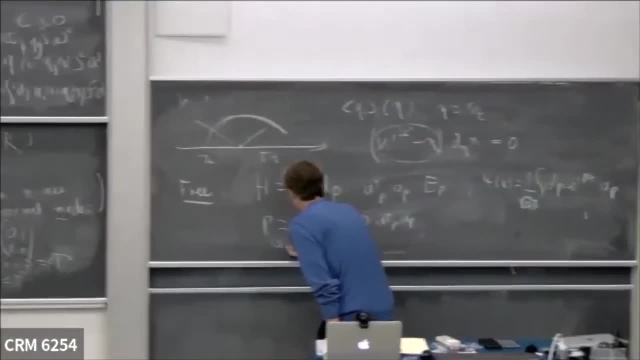 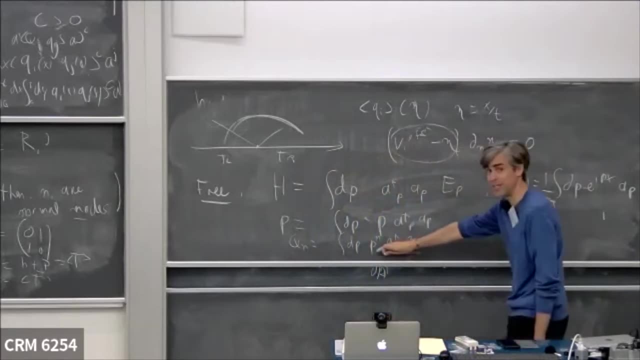 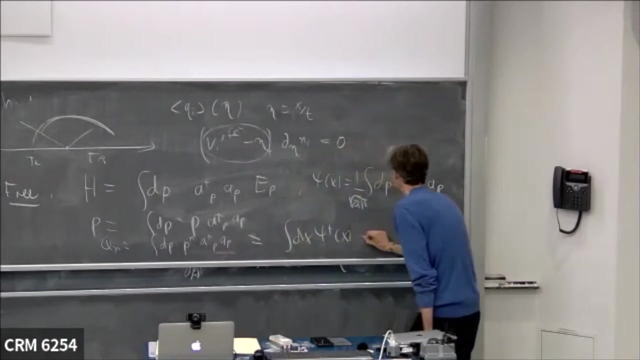 powers of momentum. so like the qn, something like that, the tuition of the p p to the n a dagger p, ap, That's also a concept quantity for any p to the n Anyë can be written as integration over x psi, dagger x, and then minus i d to the n psi of x. So 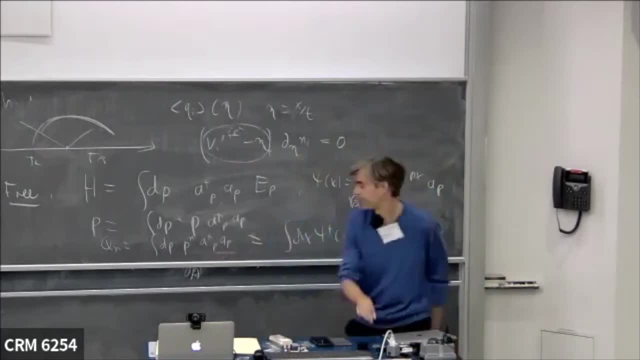 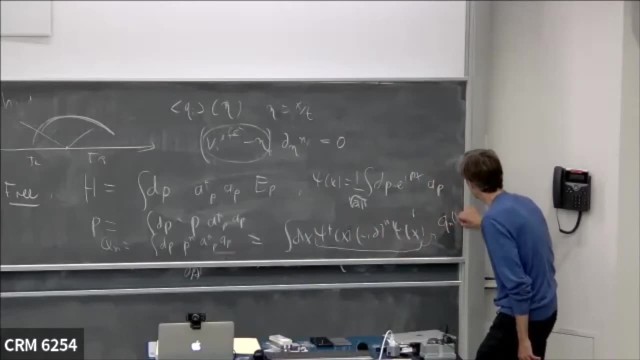 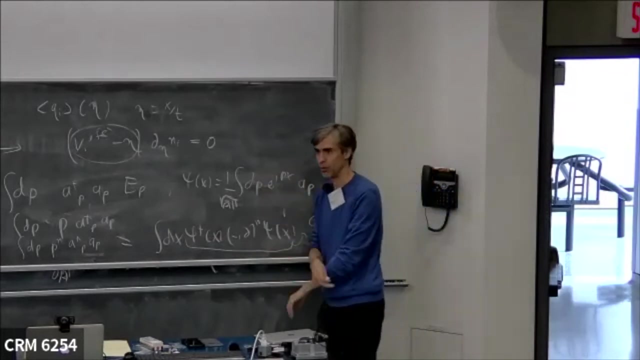 this is actually a nice extensive concept: quantity with a local density. This is my qn of x, my local density. So that's a very simple three-terminal model. This is straightforward: direct, just Fourier, transform and stuff. There's nothing complicated in there And I can do that. 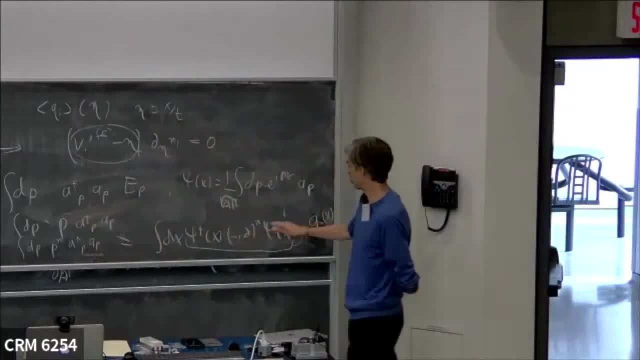 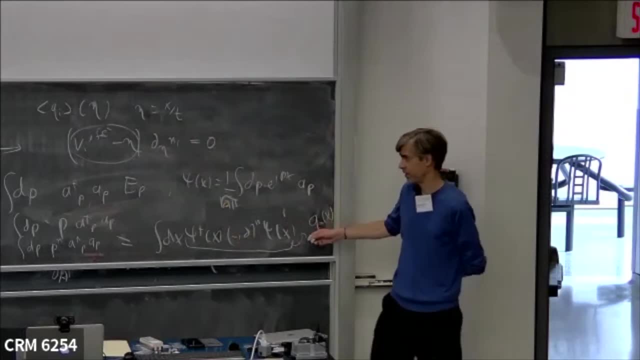 This is perfectly fine many-body system, local, Hamiltonian, local concept quantities, with all these conservation, So now I can apply earlier dynamics on that- with all these concept quantities, And now I have infinitely many concept quantities. So how do I do that? infinitely many. 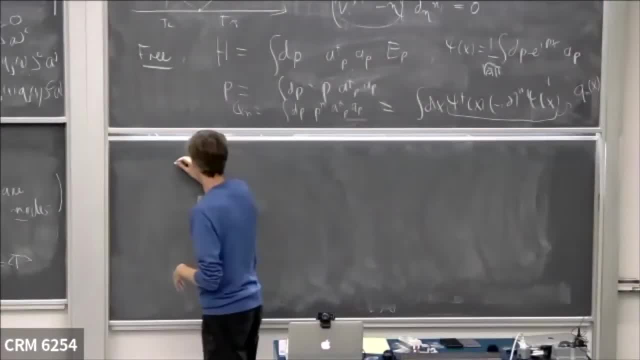 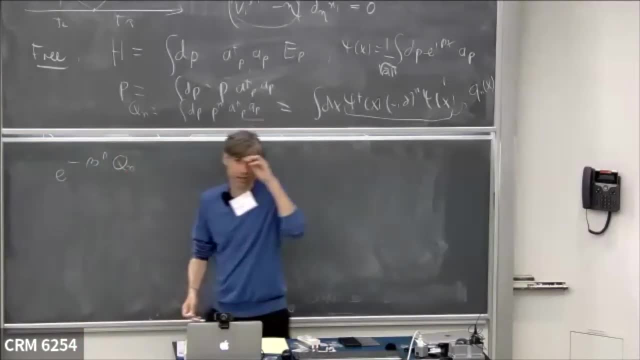 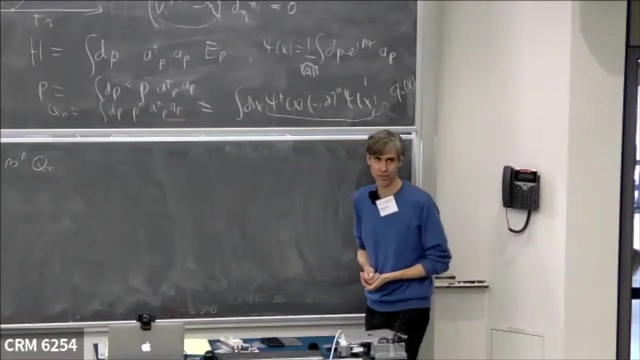 concept quantities. Well, I have infinitely many betas, So I have exponential minus beta, n, qn, And that's my kind of maximal entropy state. It's a GGE, generalized Gibbs ensemble. I can write explicitly: exponential integration, dp, And then there's some function w of p. 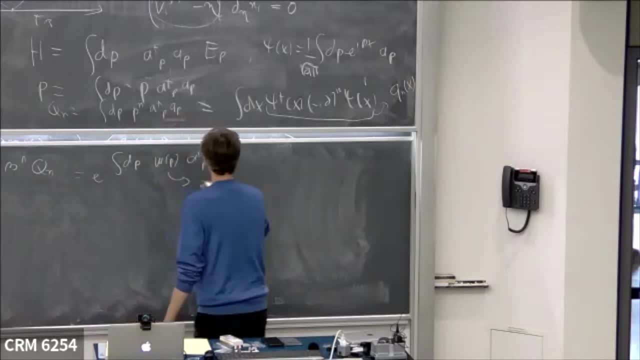 a dagger, p a p, And that function is just sum over n beta, n, p to the n. I guess Something like that. Yes, It's just that Some function, some function, but it's okay, Some coefficient. So this is a GGE. And then I 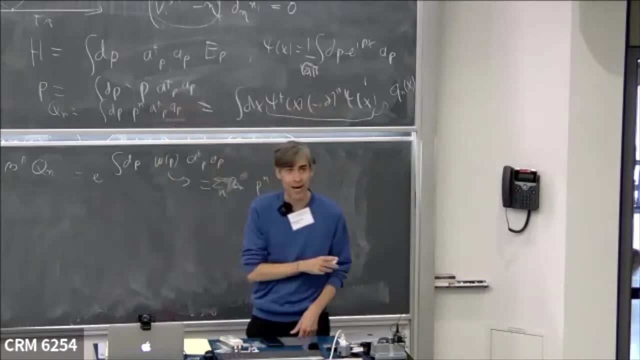 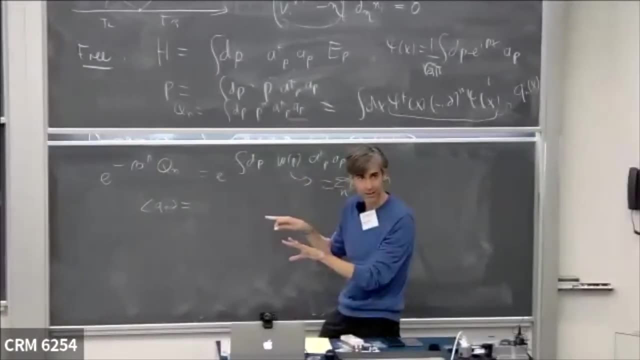 can calculate concept densities and all that. Now the question arises: I can calculate all these average of q, qn. It's simple to evaluate with theorem and all that. Okay, There's an answer. You can write specific deviation dp And I guess it's one over. 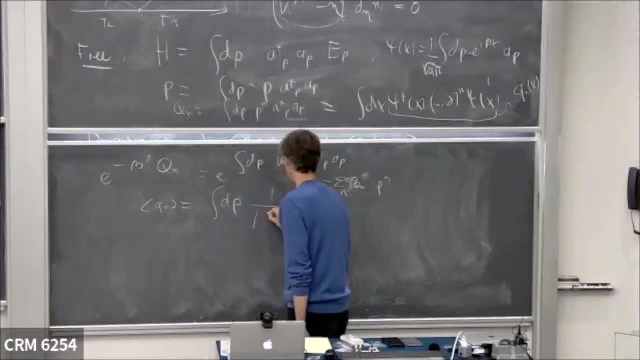 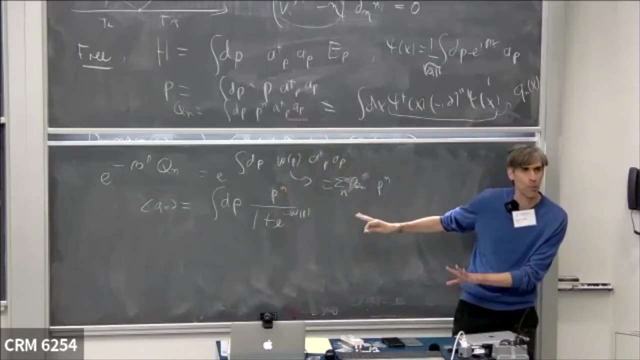 there's a Fermi factor minus w of p And there's a p to the n. I think It'd be a factor of 2 pi, something Probably a factor of 2 pi, something like that, I'm not sure. So something like this: 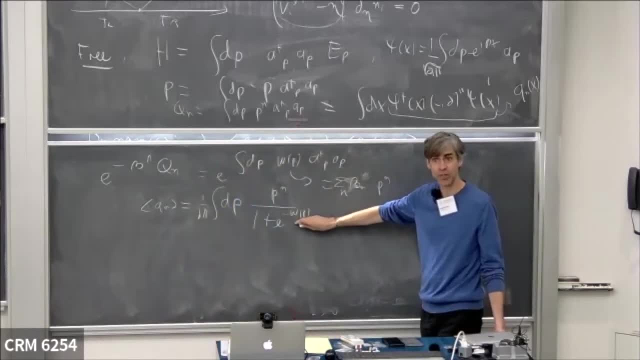 right. So this is the Fermi factor that tells me how many particles I have for this momentum And then for each particle. well, how much of this concept quantity it carries, You can calculate explicitly with the traits, with the free fermion system. 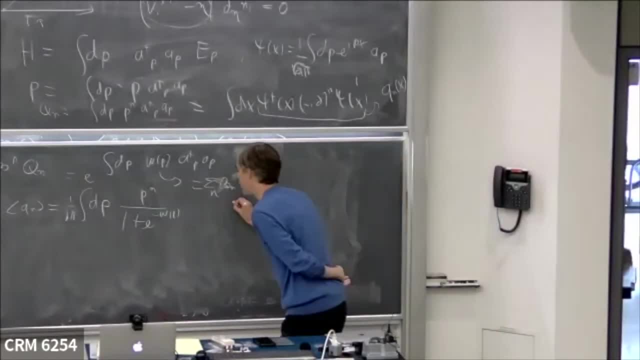 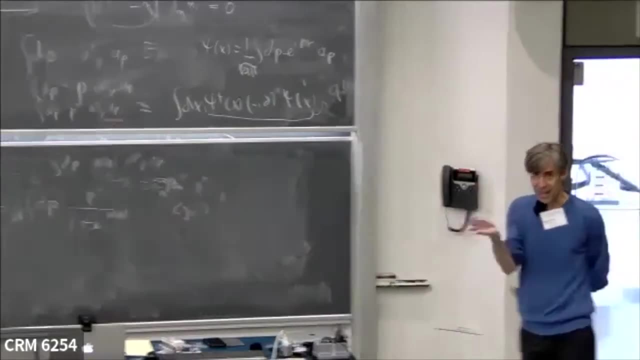 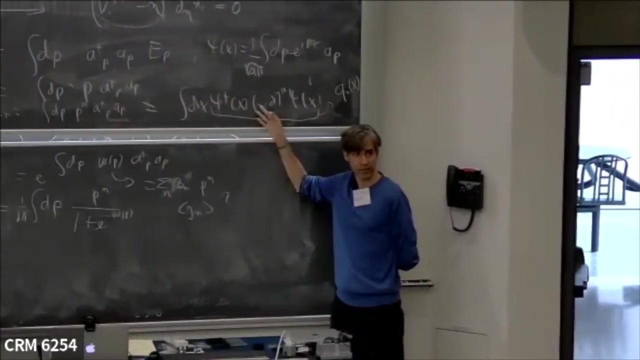 And all that Okay. So that's good. But what about the average currents? I have the average density. I need the average current. I mean this can be calculated. It's an exercise you can do. You know the exact average density. You do dt of that, You get something bilinear in the size. 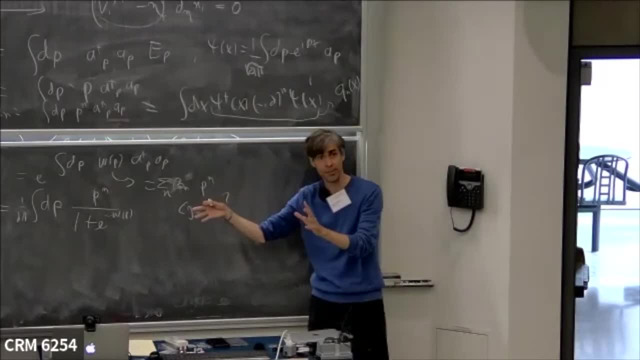 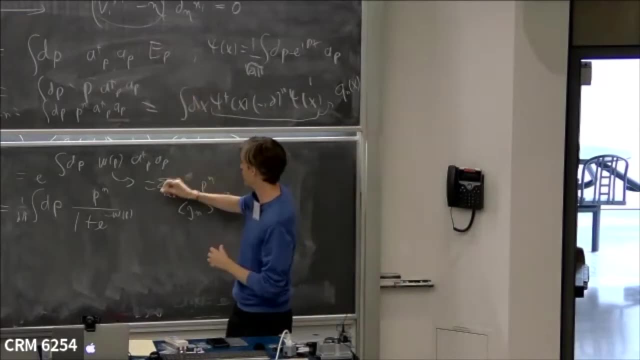 Okay, You write it as dx of something And you will be able to do that And that something is a current. It's bilinear in the size. You use Wiktorium to calculate the trace with that density matrix. It's all doable in maybe two pages. I don't know Something like that Actually. 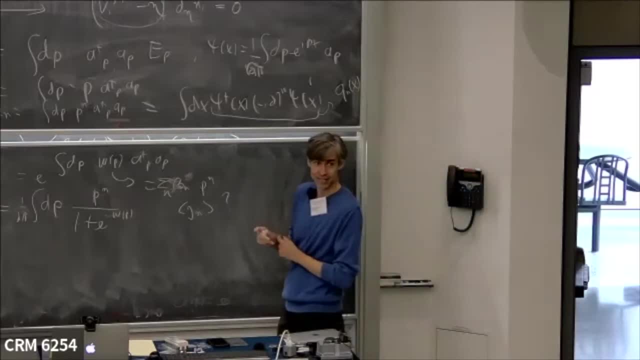 I haven't done it, But people have done it. Yeah, It's all doable, But what's the result? Well, the result. actually, it's relatively simple. You can calculate it like this and calculate it in other ways, But let me just express the result. Let me just run over to pi. 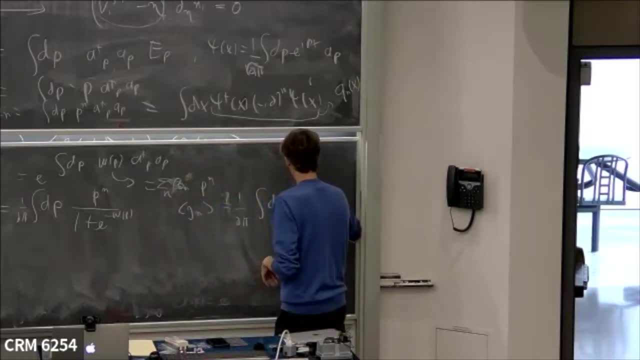 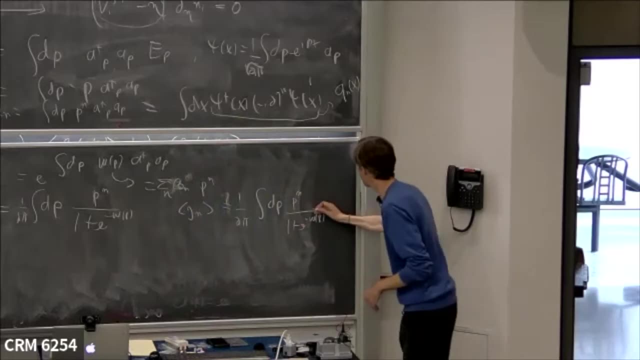 again. So you have integration vp p to the n Again. this, Okay, But the result? it's very simple. All you have to do is multiply this by what Maybe you know, You can guess it. The current is this and this. The current is the density times. what Times? You don't need to. 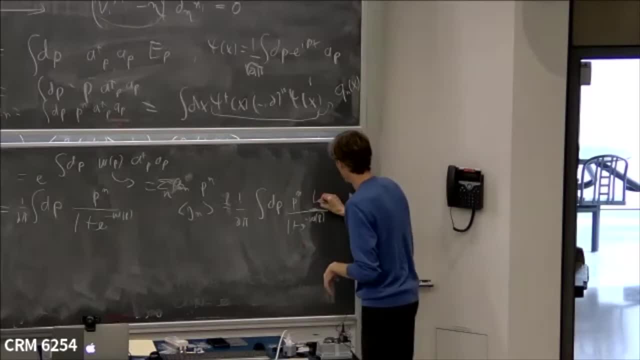 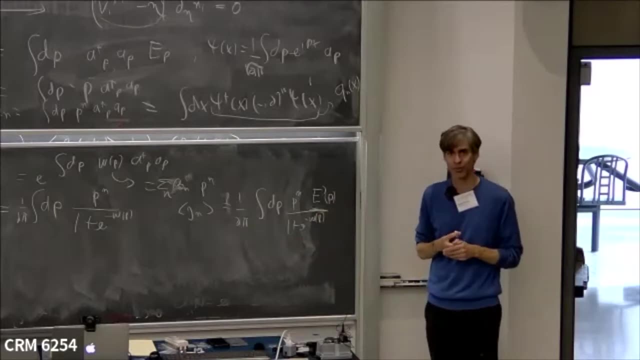 know, I don't think I would have guessed if I was a student like that. So you just have to put e, prime of p, The dispersion relation, The groove velocity, The groove velocity, e, prime of p. That's a calculation that you can do explicitly. There are different methods. 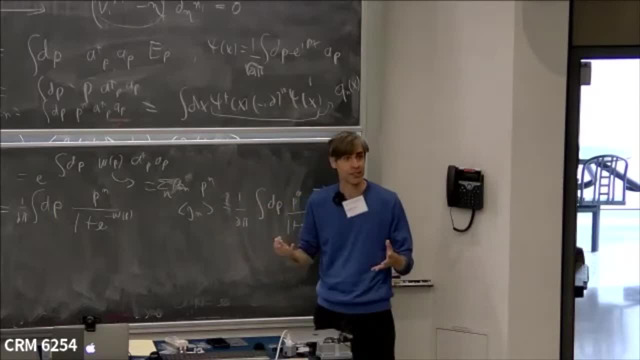 In fact, to do the calculation not explicitly, Implicitly. that gives you that, But for now, just think about that as a calculation that you do explicitly. Okay, So this is that, Now that I have that, well, I can write down my hydrodynamic equations. So I have to write down, Well. 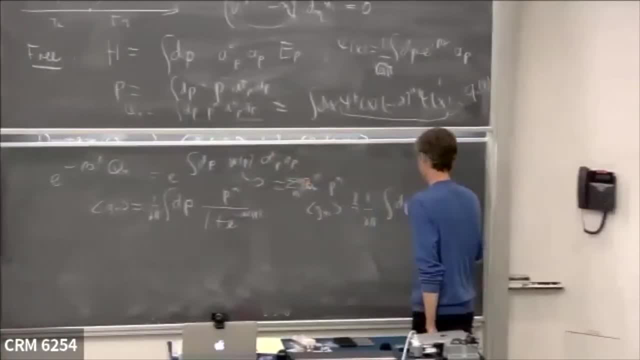 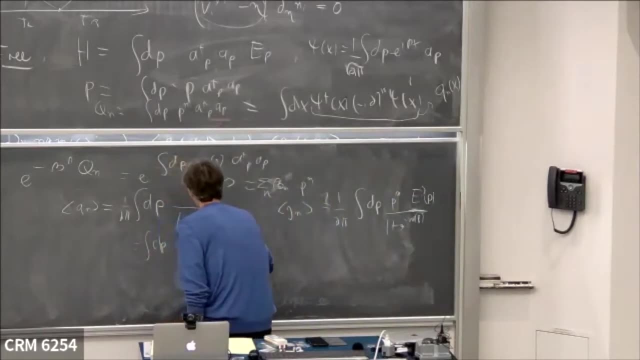 I have all these concept quantities, pn, and all that and all of that, And so why don't I write this as integration dp? some p to the n and then some density, rho of p. This is that thing, W, And that's integration dp. There's p to the n, There's the velocity v of p, rho of p. 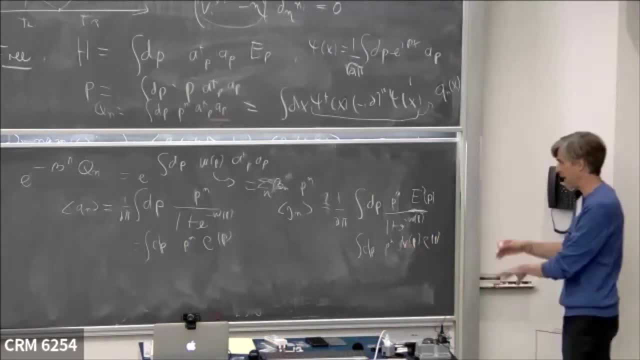 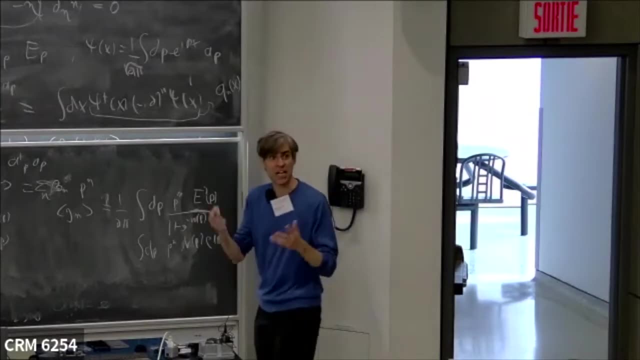 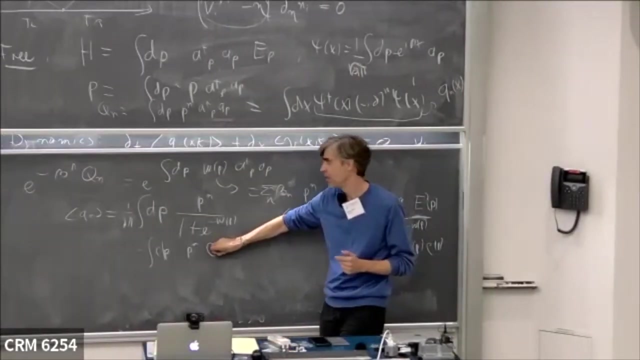 Some density. So now, Okay, So I have infinitely many equations, right, Infinitely many. But where is the spacetime dependence In the betas? Where are the betas? They're in the w, So w. Where's the w? In the rho, So rho is spacetime dependent. So what I do, Moving, So 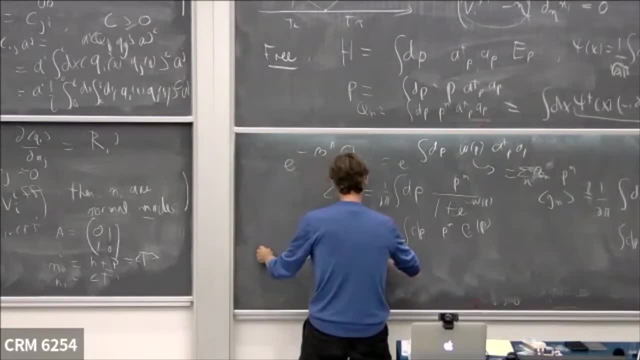 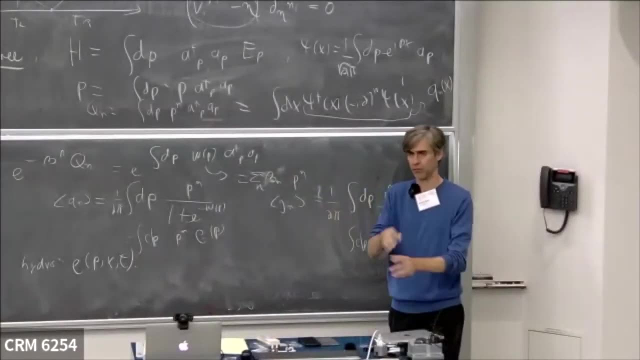 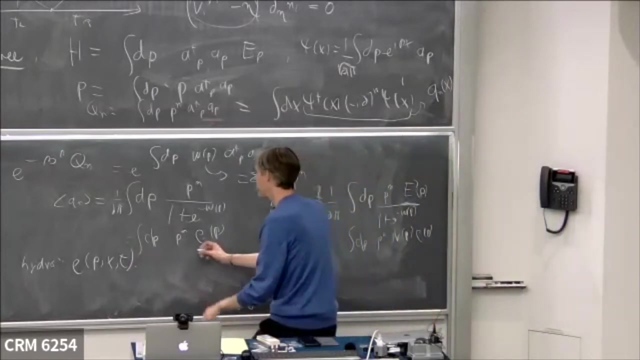 hydro. I do. rho is now a function of p, x and t. This is my local state And think of rho as being my local state and kind of any function of p there, x and t. Okay, Yeah, Local state, The betas are there And then I write the equation. So 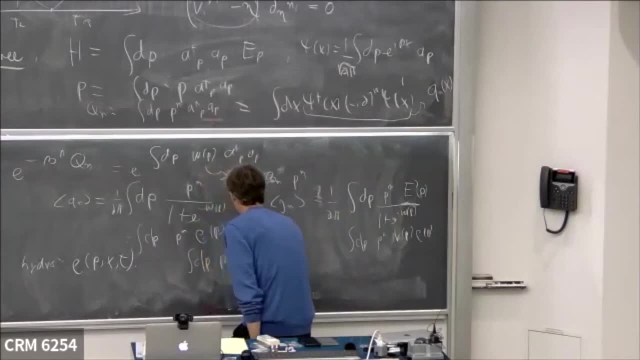 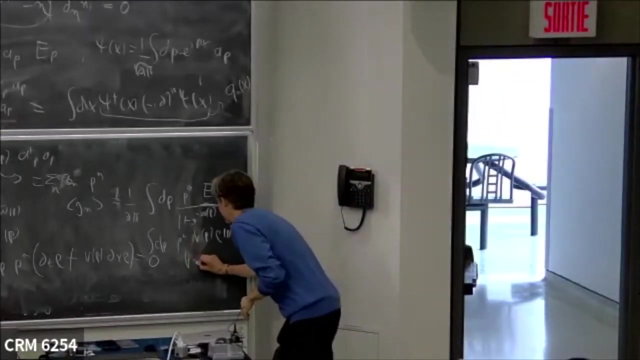 I have integration: dp p to the n. I have dt. rho minus v of p. dx, rho equals zero. This is my equation: dt to the n plus dx to the n equals zero, And that should be valid for all n. So 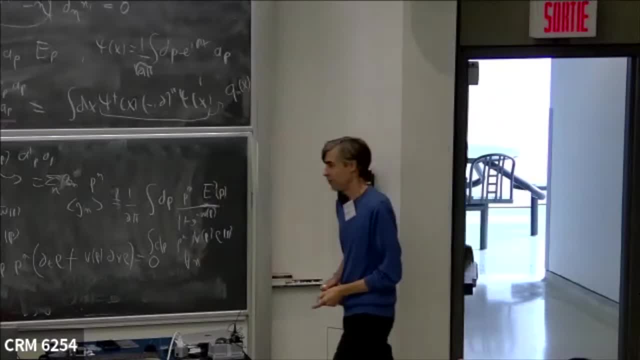 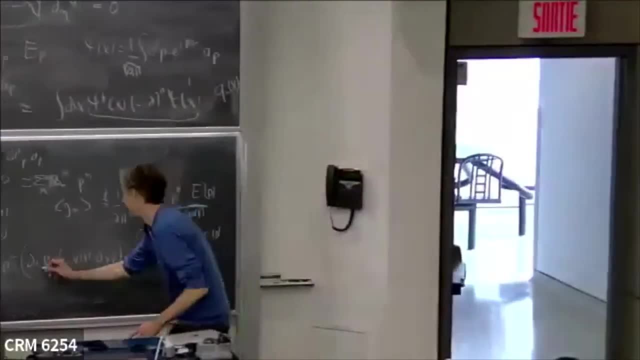 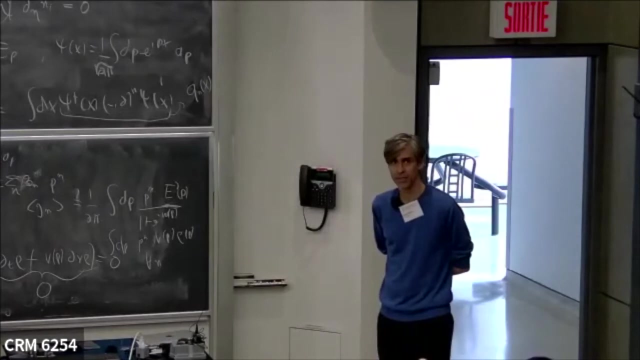 what do I conclude from that? Well, I conclude that, well, this should be orthogonal to p, n in the L2 space. I don't know. What I conclude is simply that this is zero. So I conclude that I have an equation for a phase-space: density: rho, p, x, t. The equation is nothing else but. 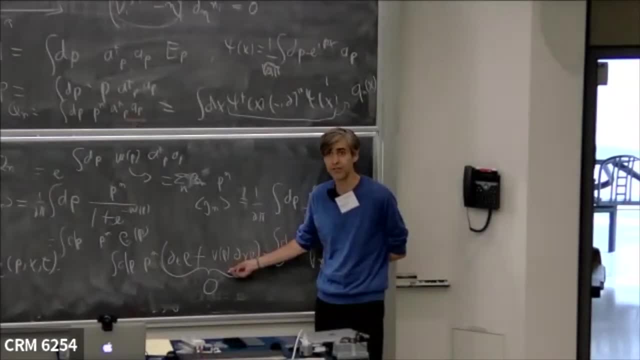 the equation, isn't it? The equation is nothing else, but the equation, isn't it? Heubel equation: in phase-space, You know the Heubel equation: when you have three particles and you have the conservation of phase-space elements for three particles, This is conservation. 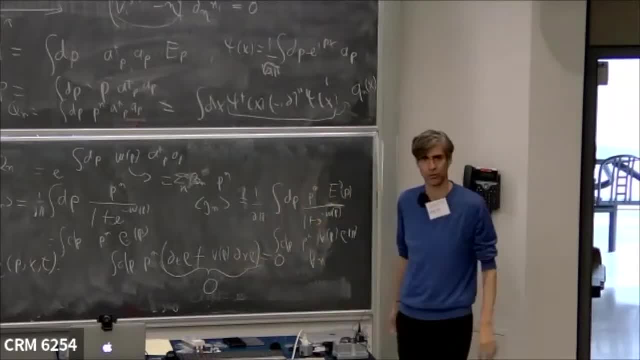 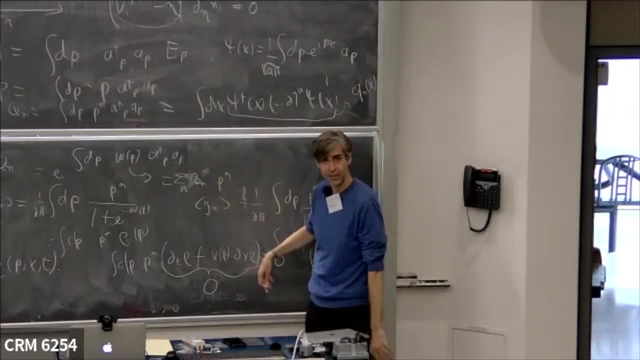 of phase-space elements, So the Heubel equation for three particles going in phase-space, And they all go as well as t v o p, So the free fermion that could have done the free boson as well. The Euler-Harder dynamics is the Heubel equation of phase-space conservation, So it's 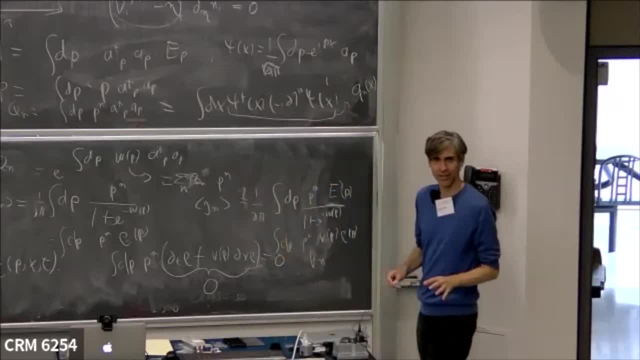 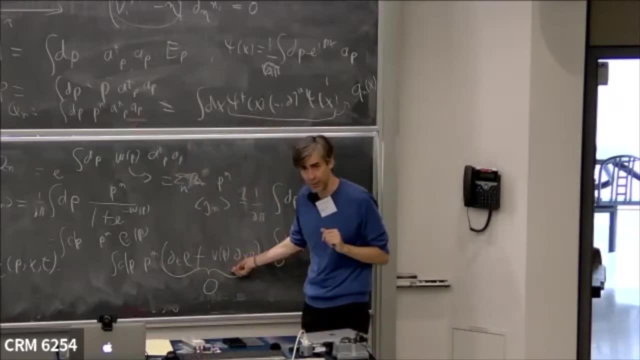 kind of a nice reinterpretation of this basic equation. Okay, And this is true, So that's true. Now, this was derived from Hydro perspective, but it can show, it can prove that it's correct at large scales in the free fermion system. Yeah, So five minutes? Yes, Excellent, So you can. 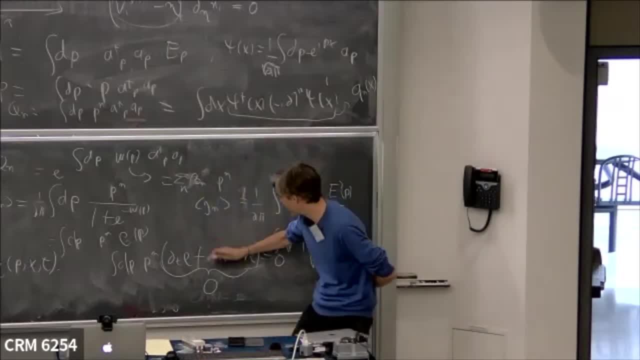 Yeah, sorry, Yes. So from there to there, Yes, And in fact p to the n. they're not quite complete, actually They are not. In fact there are many more constant quantities than these. You can put here an antiviral kernel of x and y. 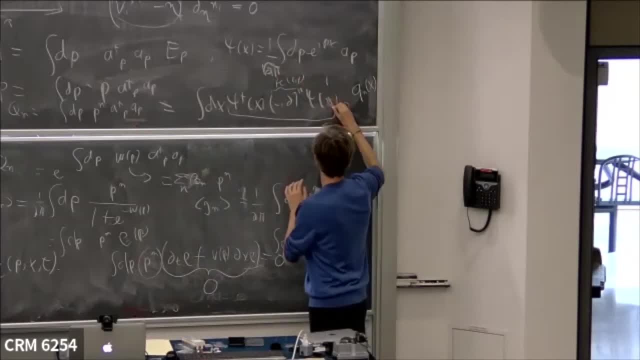 Or x minus y. You have an x and a y there, And as long as x minus y decays sufficiently and has the right properties for being, consequently that will work. And there are infinitely many consequences. So there are many, many more. There's a continuum. 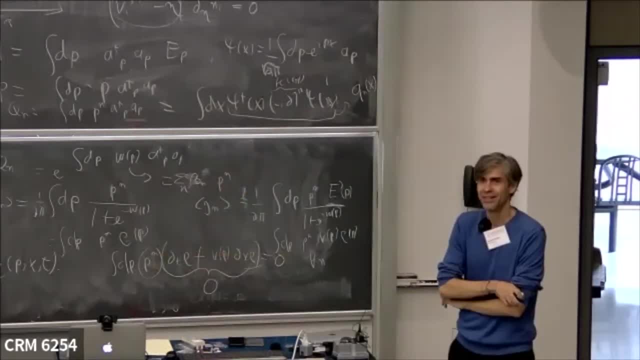 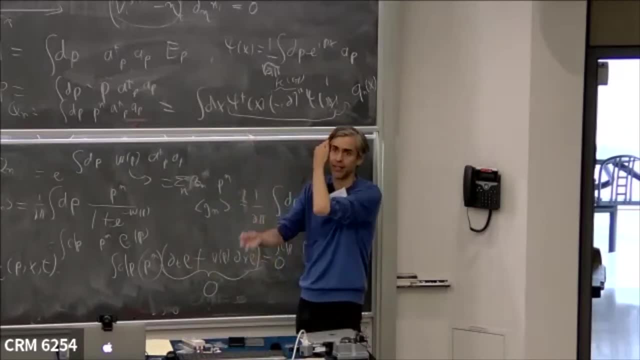 And that's why you can actually do that. You can go to a constant Yes. exactly, This is the last bit Now. maybe I described that then at the beginning of next class And I think that would be the best. I thought I would finish, but okay, Of course it was a bit too much. Yeah, you can. 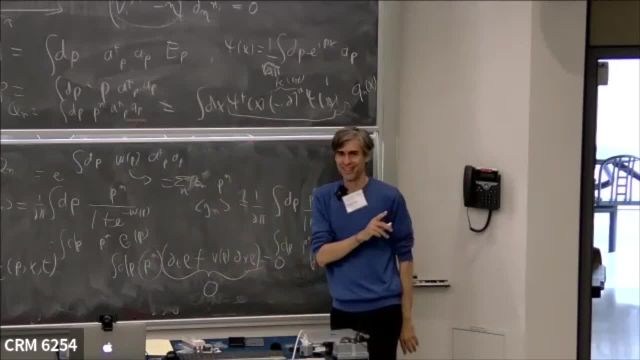 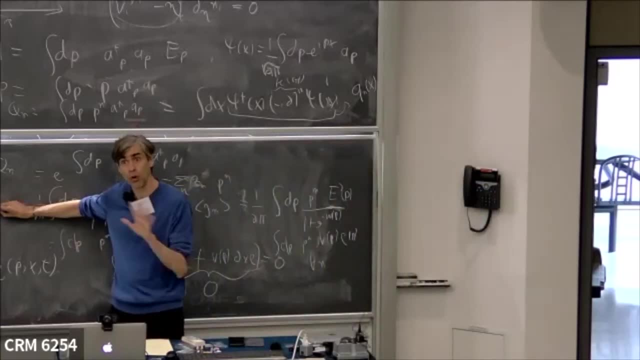 redo all of that for integrable systems. And the trick, integral system, the non-trivial bit You see for integrable system, these average densities. they're known for a long time. actually This is from thermodynamic beta and that, Something similar to that with the pseudo. 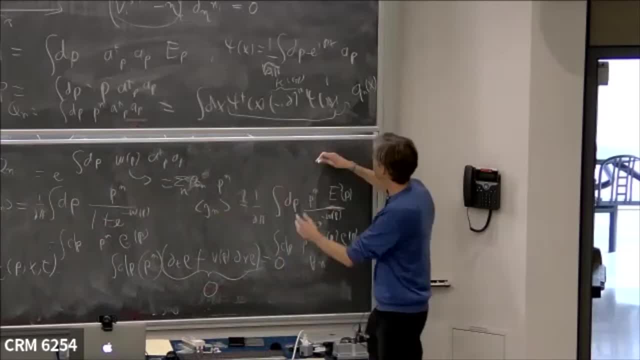 energy, that's there. But the average currents, See, I said: well, you have to do that. Well, we don't know. in LS, for instance, We don't know how to write explicitly. Well, there's some trick to generate them, But then how to write the currents, how to calculate the current, that is. 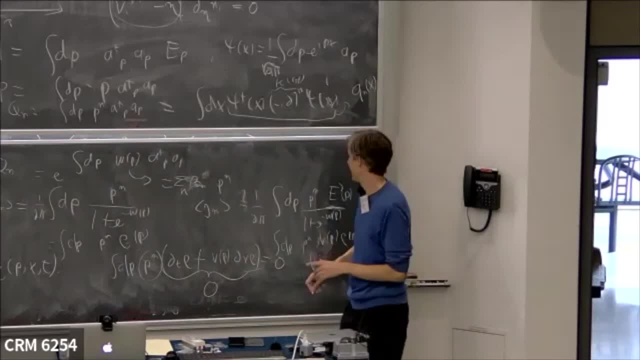 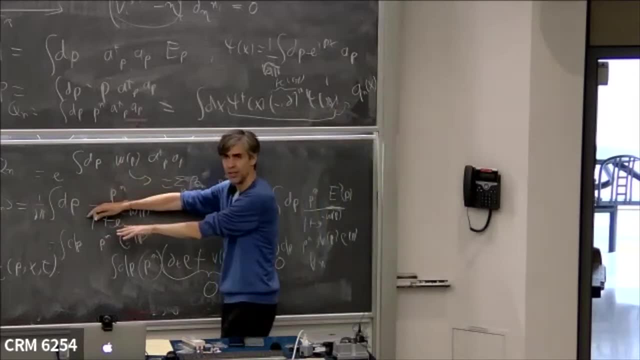 hard. So you need some other tricks, and there are other tricks- And then you can write that also in the TBA form, thermodynamic beta and that form. So you can use the old result that people have derived, Use the tricks, write the currents, do that and get an equation, And that's this. 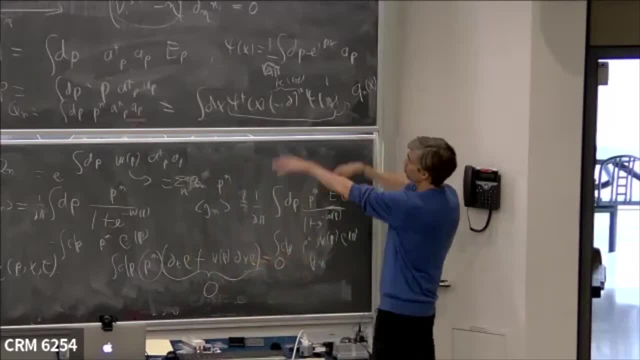 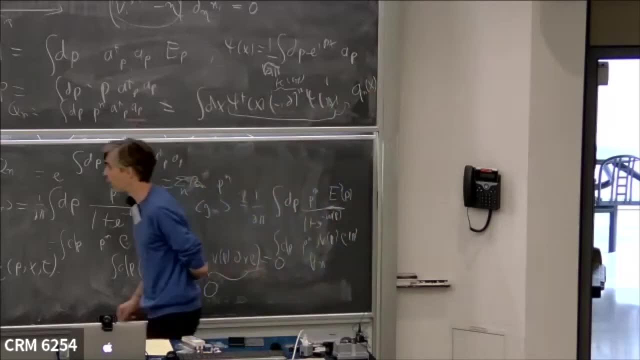 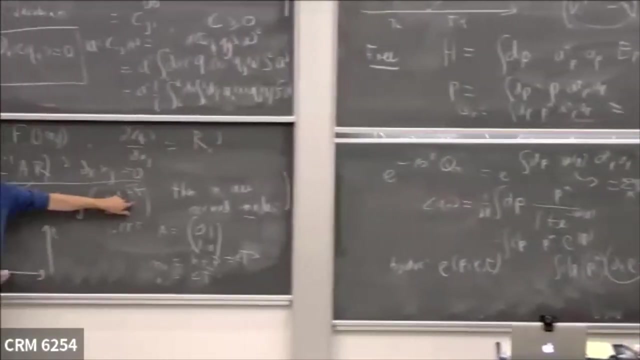 generalized hydrodynamics equation And then from that that allows you to solve this initial value problem. And here you see that. You see this is directly in the normal mode form, diagonal form, with the V of P being this V effective. So the V of P are the spectrum of the Flux-Jacobian. 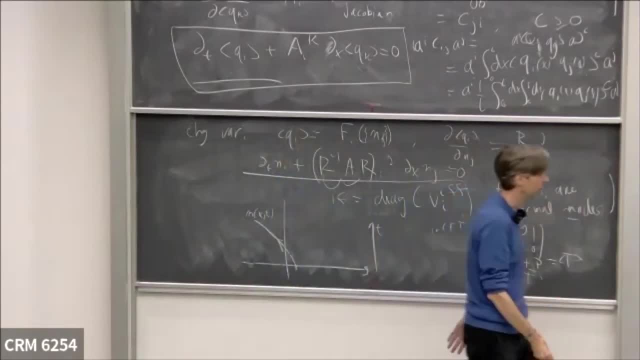 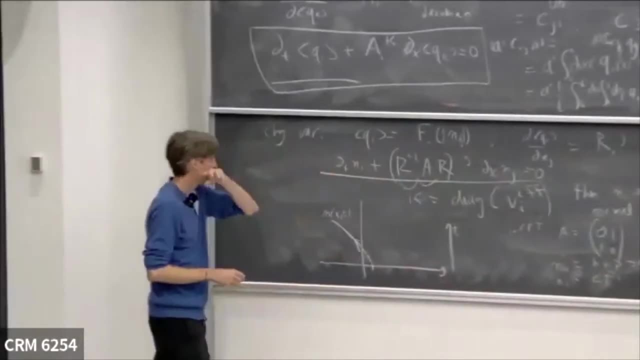 free models, It's immediately in normal form And in integrable systems. one can also write the normal form and find the right spectrum, V, effective of P and all that. And you see that these modes, I and I, they are the particles, the momenta, the piece, So the quasiparticles. 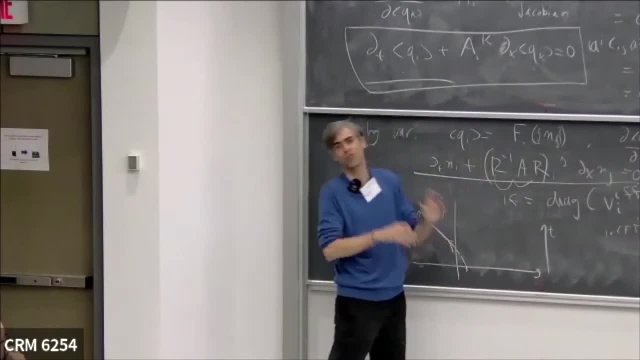 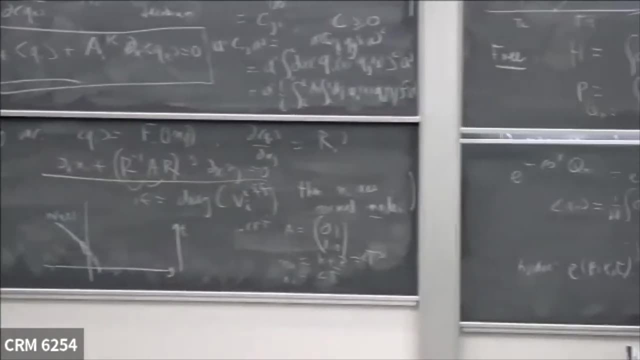 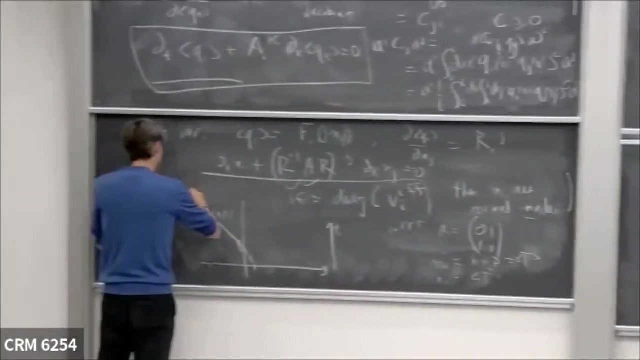 are the hydromodes In free models, same thing also integrable models. And yeah, then you can just solve. I finished there. You can solve that equation quite explicitly And all you have to do is the particle of momentum, the row of P X, T, you evolve it. 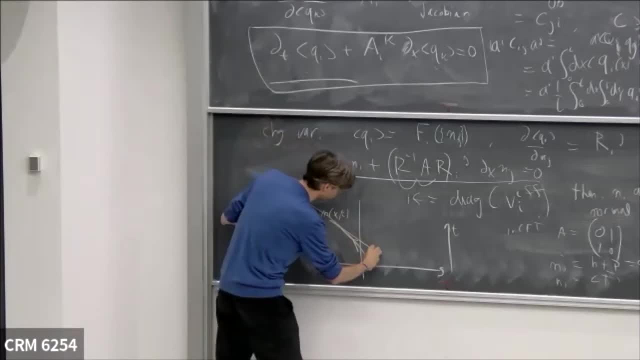 back at its velocity P, And in free model it's just straight line. See where it goes. If it's on the right, then it's No T right. If it's on the left, then it's T left. 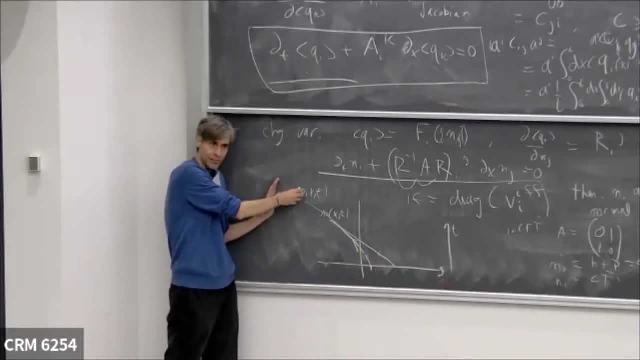 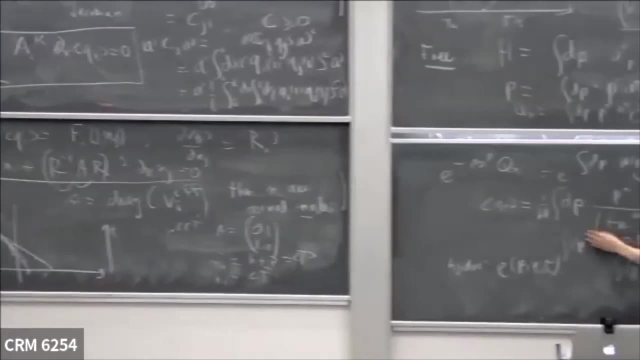 right, It's temperature that particle, as if it was in the left, T left or T right temperature. And you know how to do that because this is explicitly. you have a separation of temperature for every mode there, So you kind of know explicitly what to write. 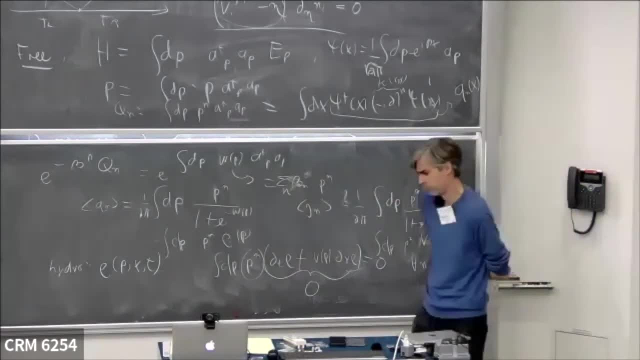 So you have an explicit form and also similar. you have something relatively explicit in integral models as well. So you solve the Roman problem. So that's the idea of hydra. It goes beyond the CFT. I think that's it. I'll stop for now, Thank you. 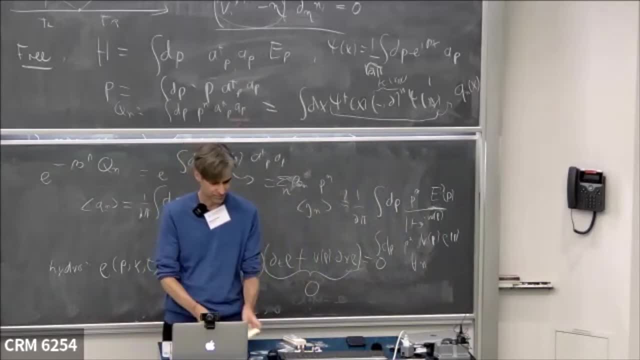 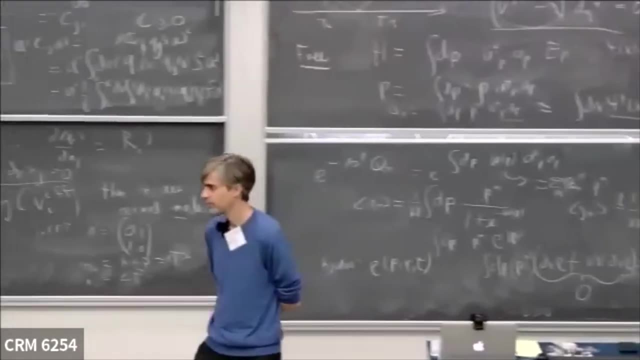 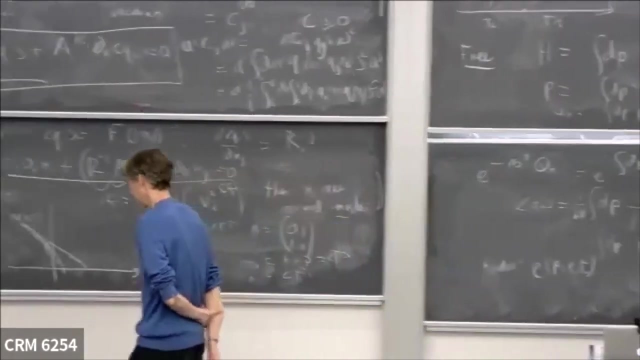 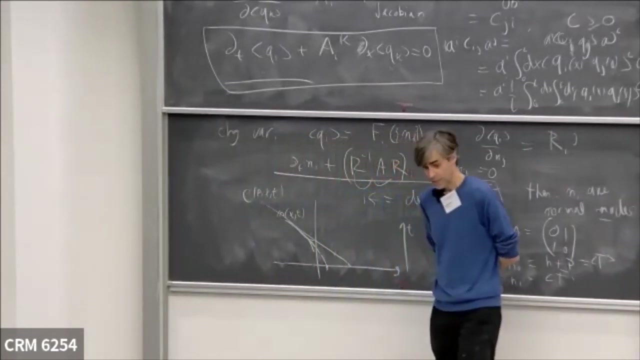 Yeah, I think I have a question. So, as you know, for two terms, one view is friendship and the other one is the entanglement of this. So the function of the property is the entanglement of this. So is it directly related to the function of entanglement? 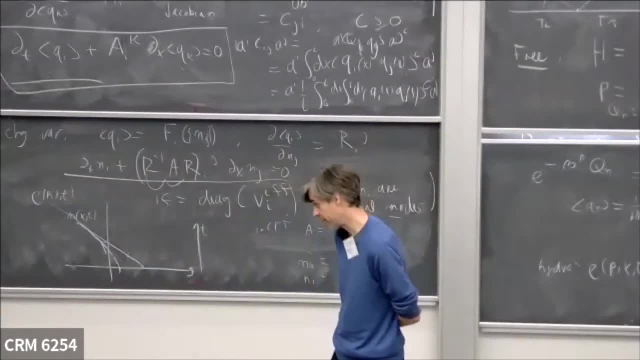 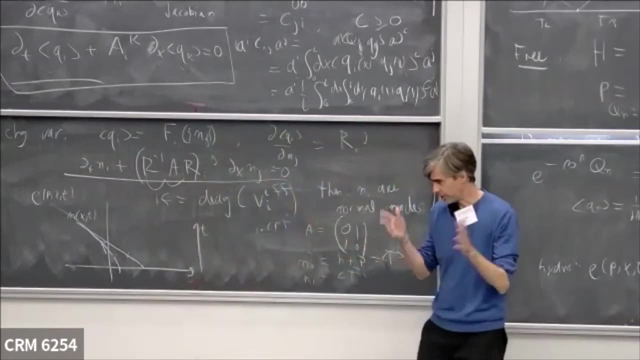 Yes, the answer is yes. So this is actually an interesting Nathan's question. So in free model you can see that even in integral models there's also this entanglement, growth, and all that when interpretation in terms of quasi-particles, And that involves exactly. 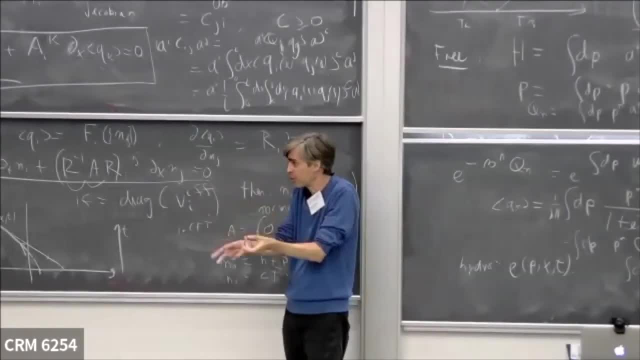 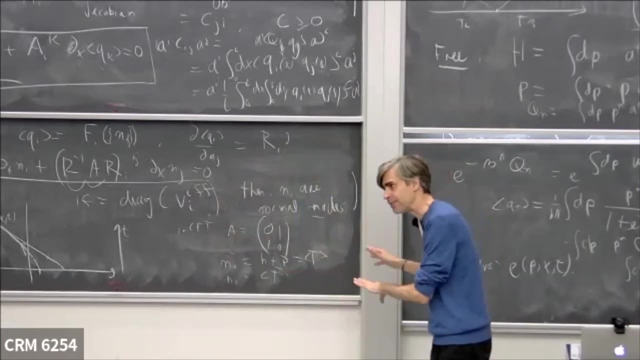 the flush Jacobian spectrum, And so the quasi-particles have these velocities. And now the full relation. the proof of this picture from hydrodynamics is not really yet done, So we're kind of working on that, the hydro-re-understanding. 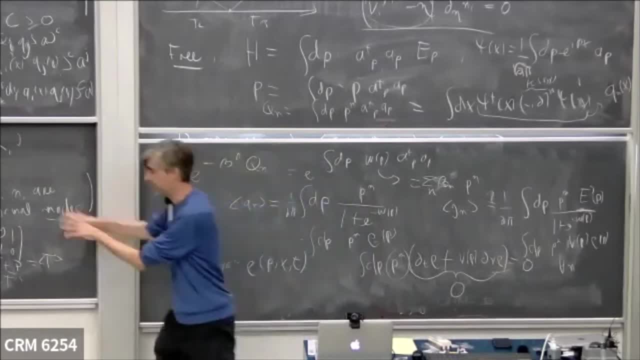 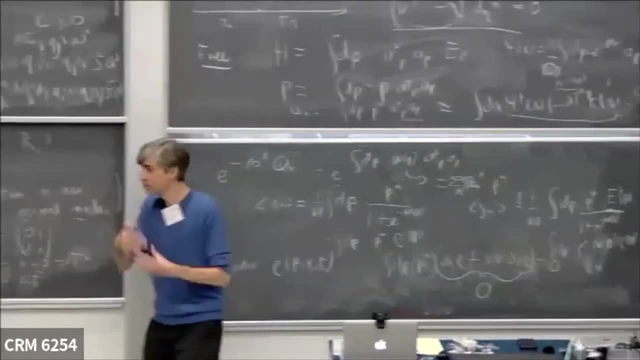 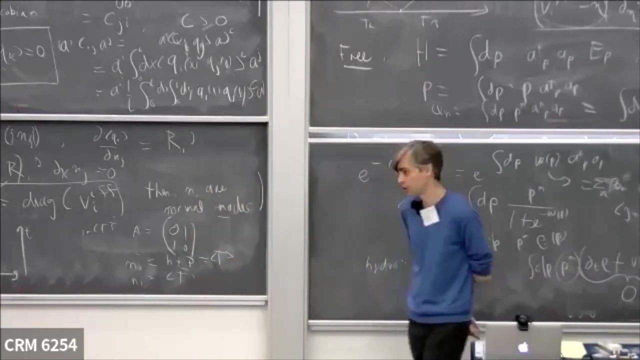 but the formula is already there And it's the same object that I involved. But the proof using hydrodynamic ideas actually requires fluctuations, study fluctuations, Because entanglement raises fluctuation. So it requires certain fluctuations, not just averages of local observable. It's non-local. 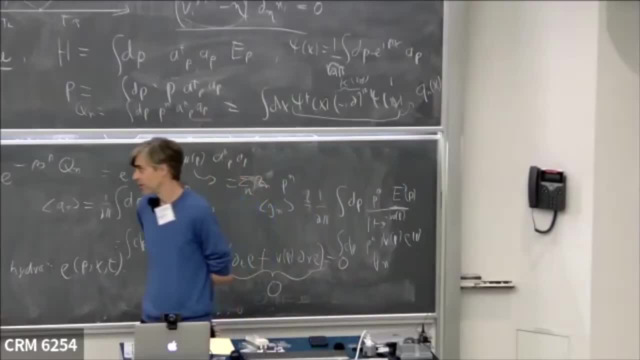 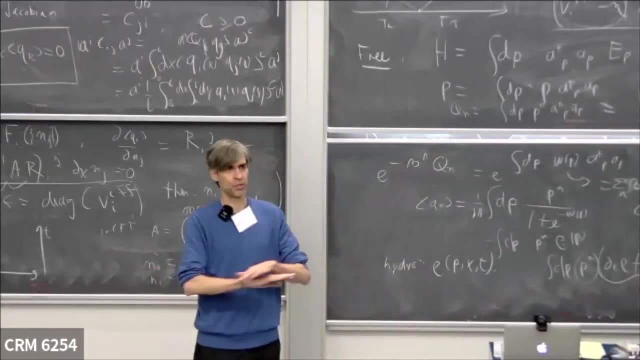 So you need to go a bit further, but it's the same idea. Yeah, This is also a very good question actually. So it very strongly depends on the initial state. So this is like where you have some initial state and you suddenly change it and then you have particles. So the way I can write this, I'm going to get that in the talk. So I'm going to write an energy function and I'm going to write it down. So this is part of the idea of that. But 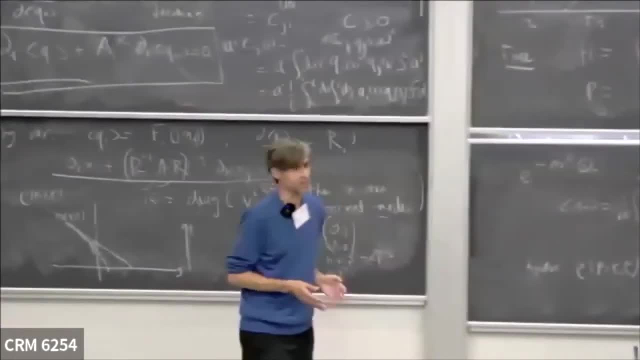 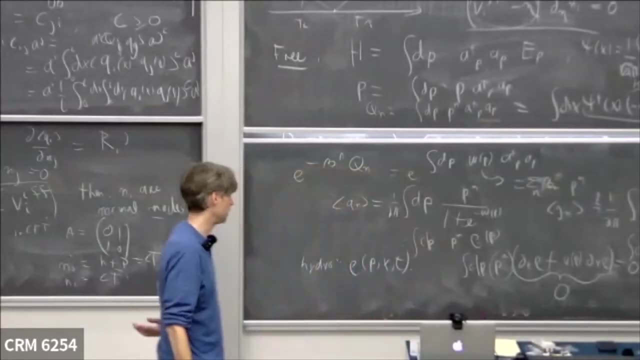 So it depends on the initial states. The initial state, if it limits pair of particles, then you can deal with that. If not, if it's more complicated, then it's a bit less clear, And otherwise what other properties it requires. 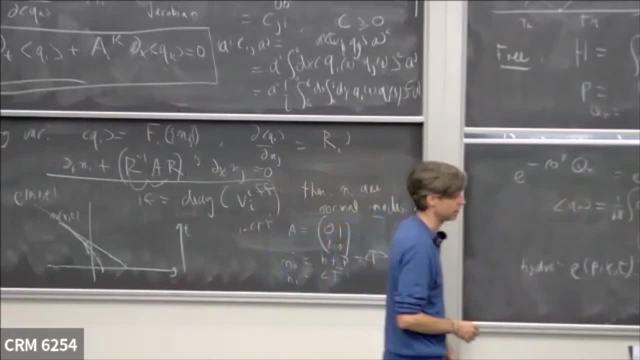 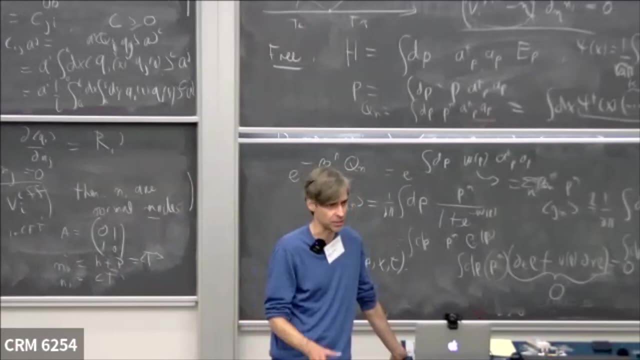 I mean for integrable system is relatively general. Now I don't know, maybe there are some special cases, No, no, no, it's especially the initial state, as far as I understand right now. that is crucial to have nice interpretation of the particle. Thank you.